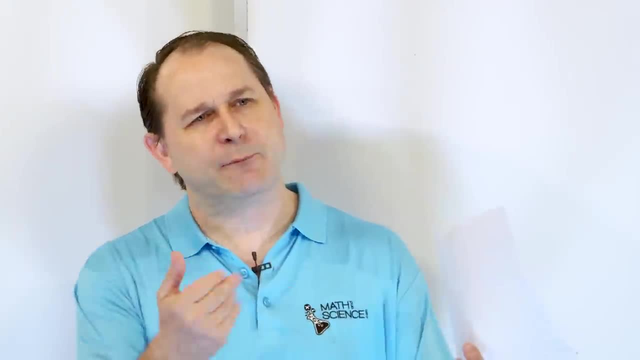 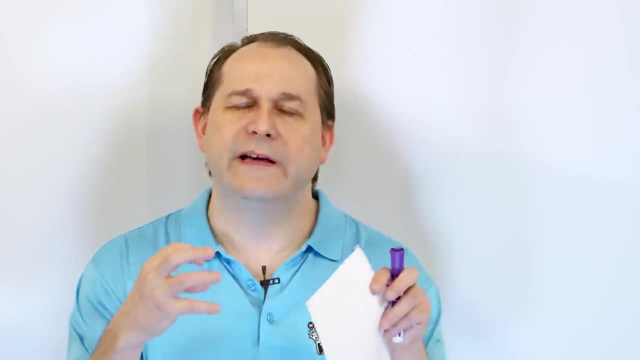 bones. I want you to wake up in the morning and say, well, that's a chemical process there, How does that work? And have some excitement and curiosity about that. All right, That's my goal. I want to give you those tools so that you can be excited and kind of like ready to conquer this. 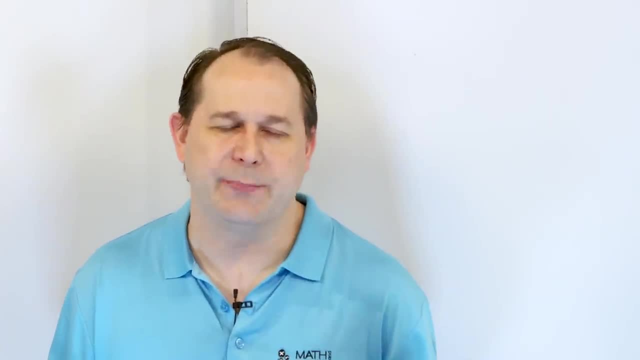 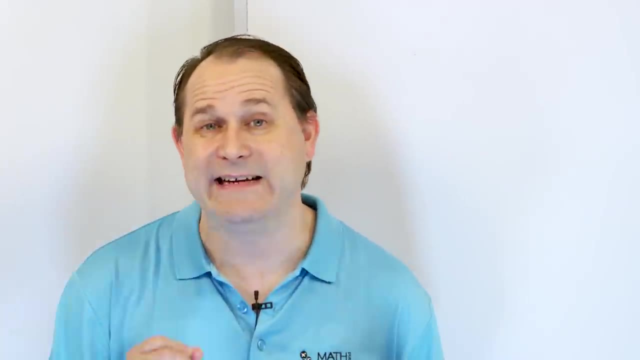 journey that's ahead of you. Now we do have to come back to reality a little bit. Why do students have problems in chemistry? A lot of students have problems in chemistry. I will tell you my opinion of what I see with the people that I teach. The main reason they struggle is because of a 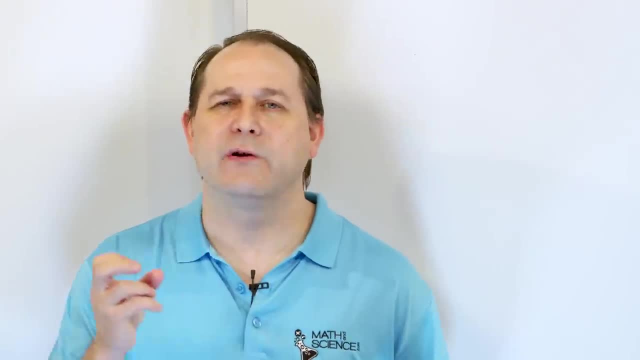 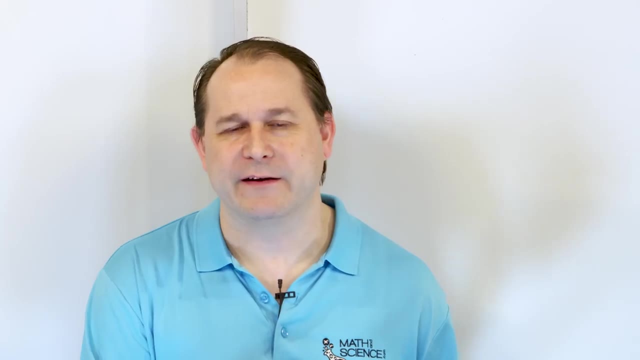 couple of different reasons. The main one is that every single chemistry problem, almost every single problem, is a word problem, right? So when you take algebra, for instance, I tell you solve an equation. I just write the equation and bam, you have some steps and you solve it. And there's. 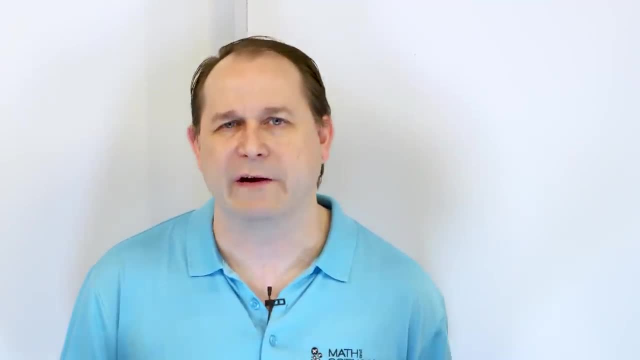 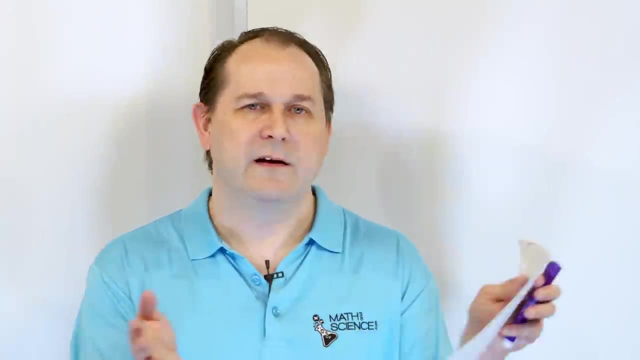 a certain way you're supposed to do it. Once you kind of get a feel for it, you can just solve it right. If you move on into trigonometry or calculus, it's the same way. In calculus I might say: calculate this integral. That's a topic you learn in calculus. Same kind of deal like boom. 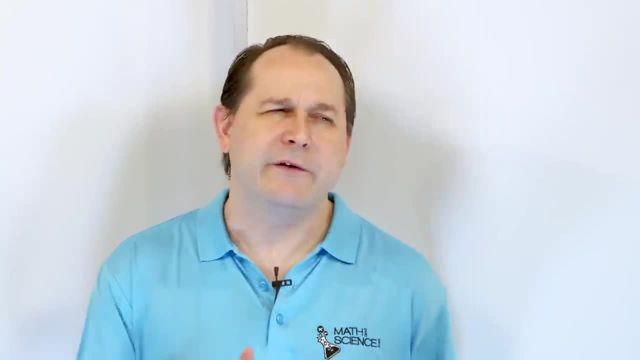 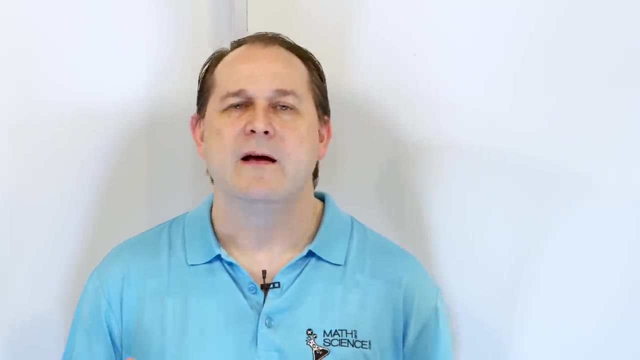 boom, boom. You learn the techniques and the methods and you solve it right. There's some word problems in there, but most of those classes are based on just learning the steps and how to handle these different kinds of situations. But in chemistry it's not like this, It's never. 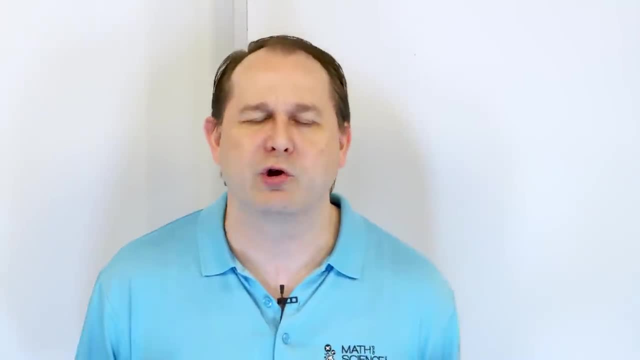 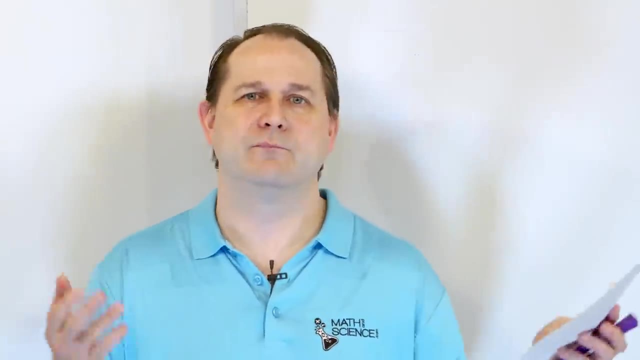 cookie cutter. It's like you have 32.7 grams of sodium chloride in a vessel at 32 degrees Celsius And then you increase the temperature of the vessel and you add some potassium, whatever, whatever, to the thing. What's going to happen? How much chemical product will you? 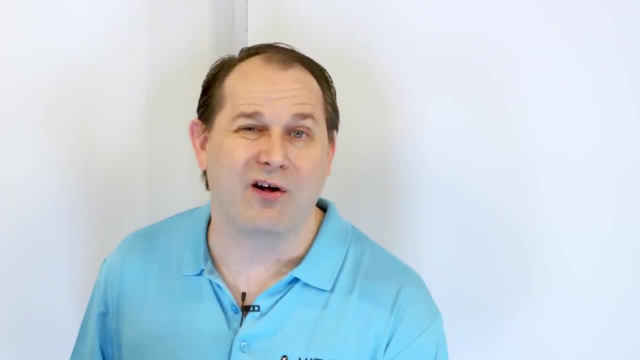 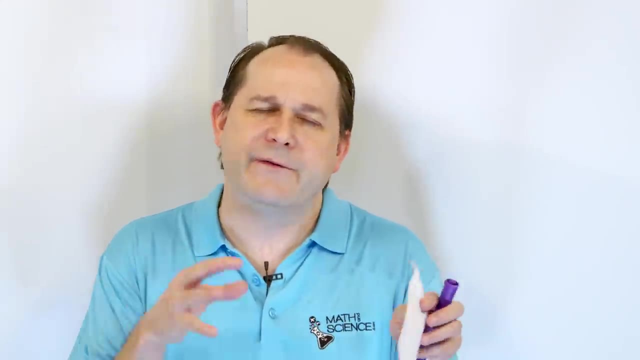 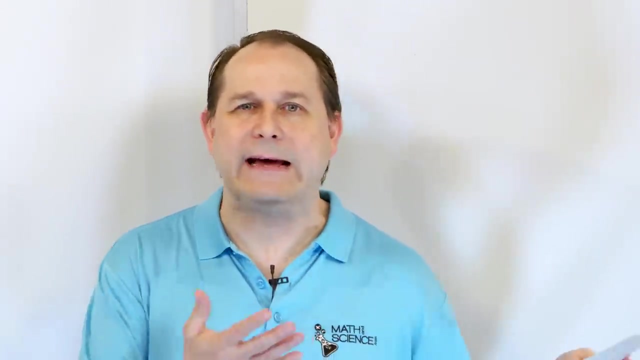 form? And also, by the way, will it form at all? And if you increase the temperature by 50 Celsius, is it going to form differently? There's so many different variations on problems that you really cannot just read a problem and just know exactly what to do, like you can in an algebra. 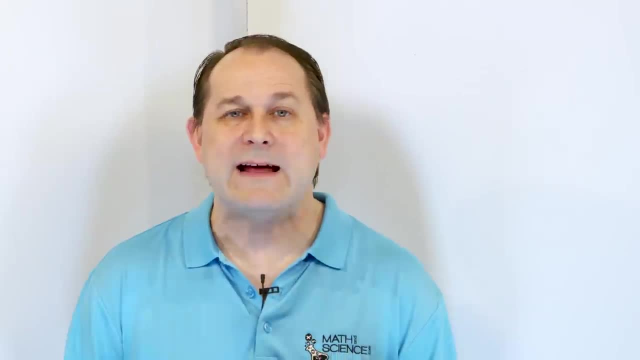 problem? You can't, And that's because they're all word problems. Now that's the bad news. But the good news is it's conquerable. And the way that you conquer it is: you have to practice it. There's really no way that you can do it without practice. 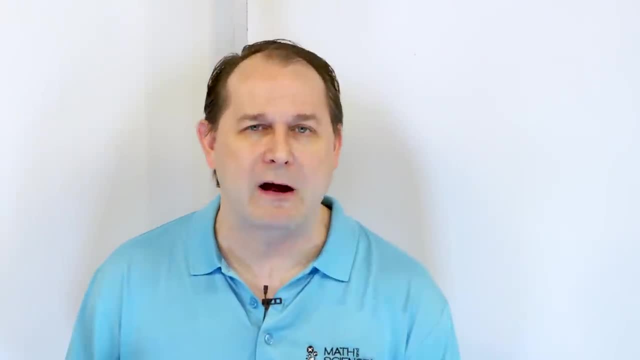 You have to read a bunch of problems and you have to solve a bunch of problems And after a while you will know what's important in a problem and you will know how to set it up and you'll know how to put it together. That is the crucial thing, important thing number one, about chemistry: 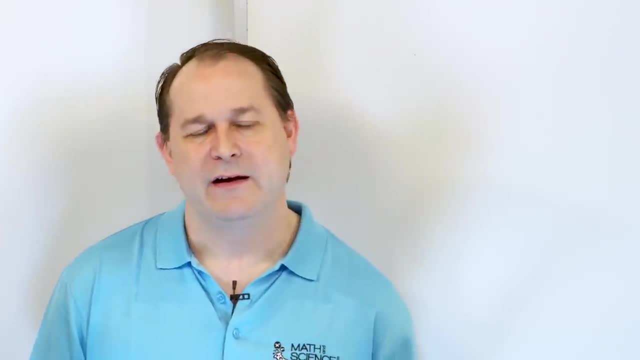 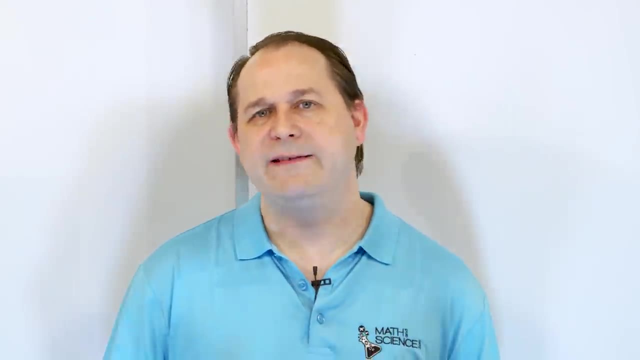 Number two is that it all boils down to definitions. You see, if you don't know the definitions, you can't follow anything right. So if I tell you you have a molecular mass of this, or if I tell you that you have a boiling point of this, or I tell you that you have an isotopic, 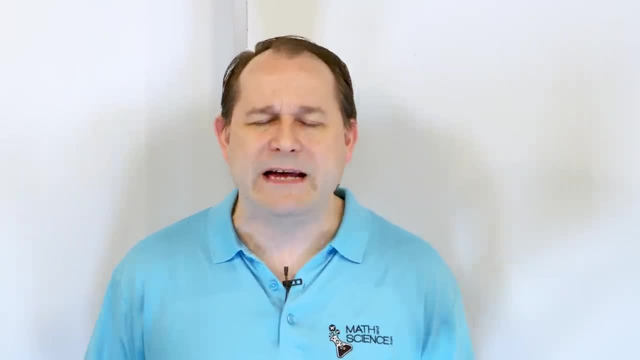 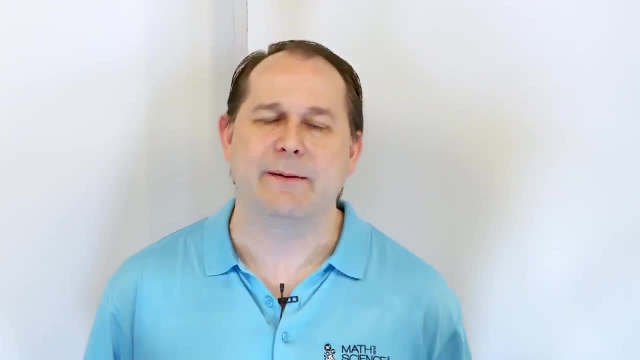 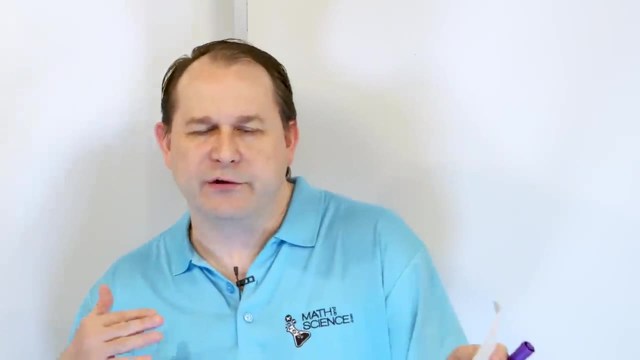 class, we have to front load with some definitions, And I hate doing that because it kind of bogs us down a little bit. But you have to trust me, if we don't cut through these definitions of what atoms and molecules are, for instance, then later on you're just going to be lost And there's no. 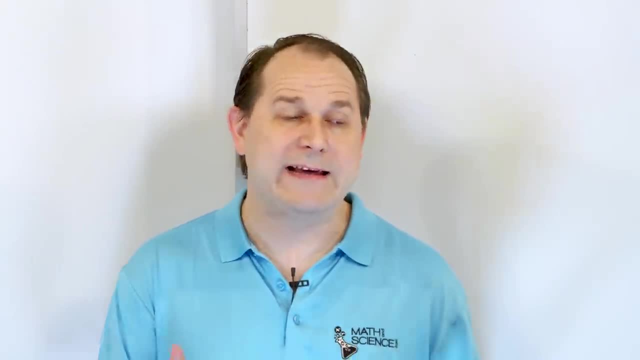 reason for you to be lost, because we can learn this, I promise you. I came from zero knowledge and we can all do it together, And I promise that's my goal here: to help you with this. All right, Why? Why should we learn chemistry, right? Why should we? In my opinion, chemistry is the most 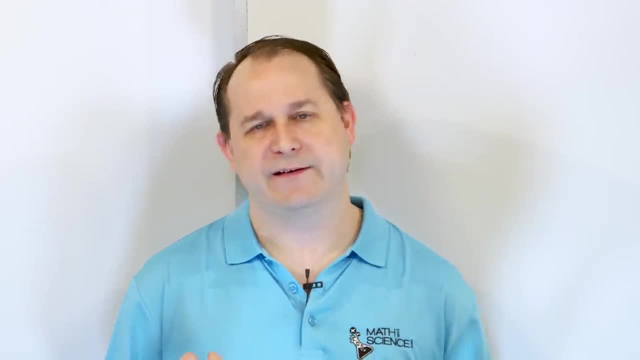 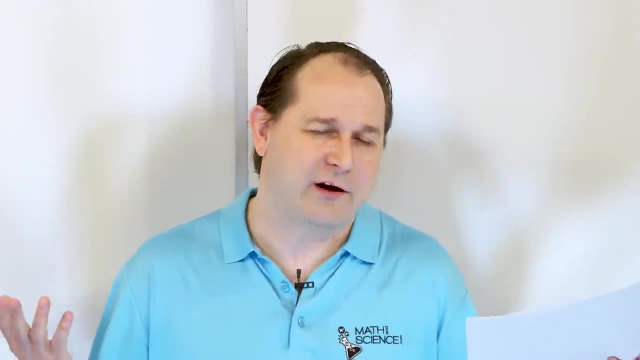 one of the most accessible sciences. You know I love physics. I have a degree in physics. I've done a lot of physics in my life. I really have a lot of passion for understanding advanced physics. And I don't understand all of it, Of course nobody does- But I have a deep appreciation. 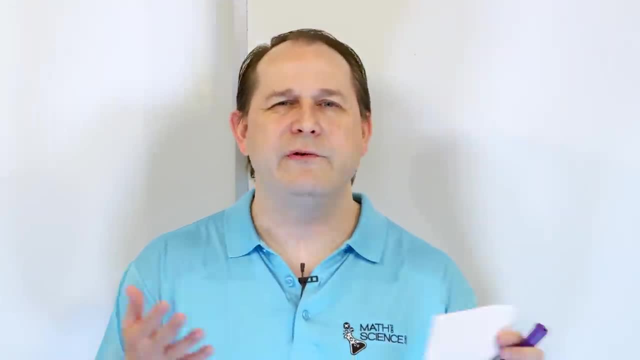 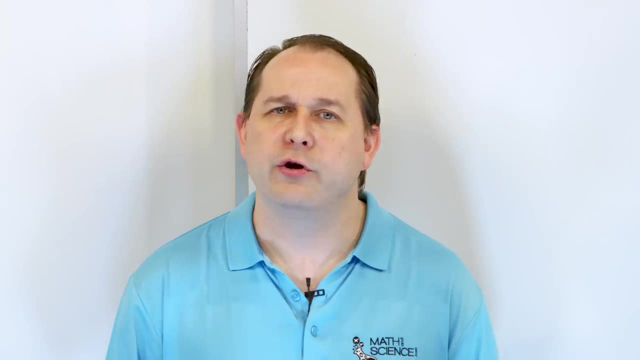 for that And I enjoy that. But the problem with physics is that once you get so far into it- like you study the magnetic field of some situation or an electric field, or you study electromagnetic waves- right, Or you study whatever some entropy of something, right- The 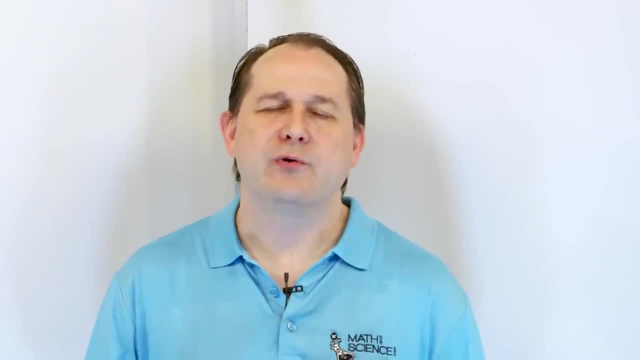 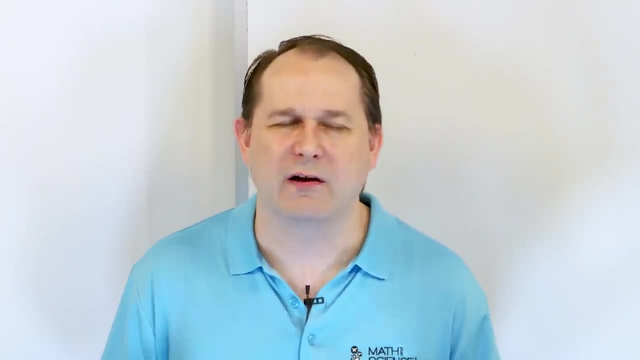 problem is that once you get back past the basic physics, you kind of have a hard time visualizing what you're doing. You start studying black holes or something at this in the center of a star, like stellar fusion or something, And it's hard to visualize what you're doing. Advanced 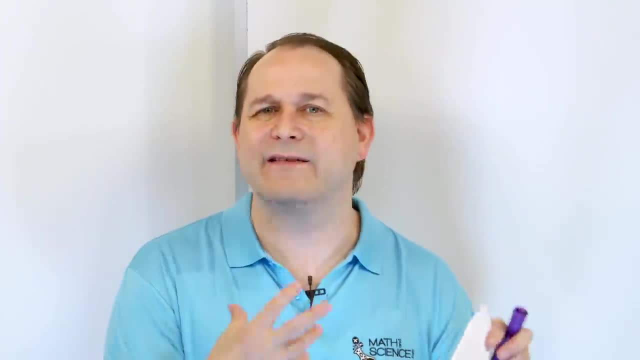 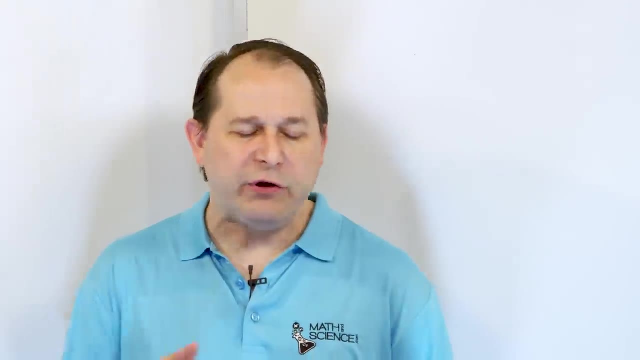 physics is very hard to visualize because you can't see it and you can't touch it and you can't taste it, And so it's hard for us to wrap our brain around. But chemistry it's very nice, Because once you understand the basics of what we're doing in chemistry, 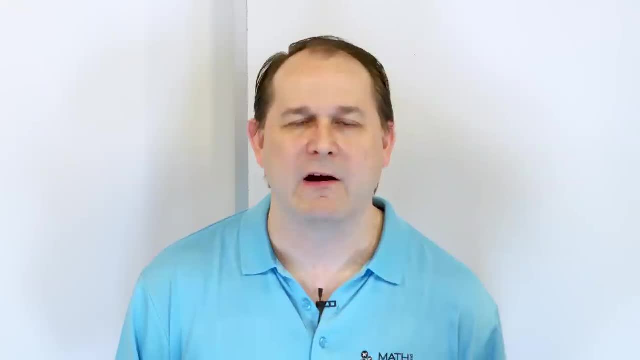 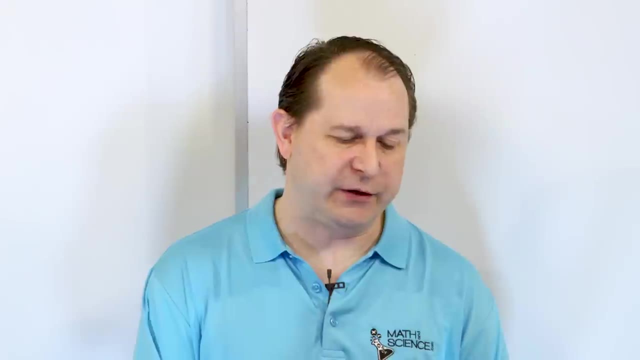 then you can walk around your house and you can see chemistry everywhere, Literally everywhere. you're interacting with something that someone has designed in a chemical way to benefit you and to serve some sort of purpose. For instance, take something simple like a piece of plastic. 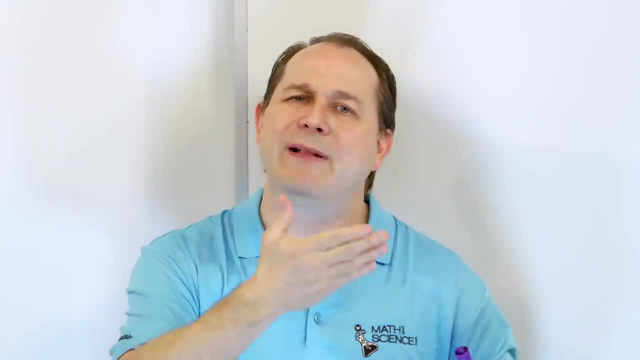 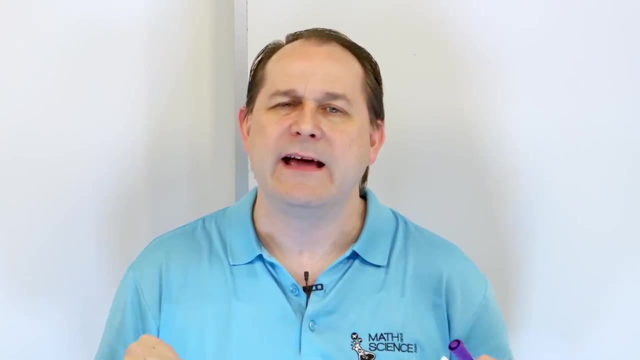 like this pen here, right, It's made of plastic. Or think of a plastic baggie, right, That plastic bag a plastic bag. and just rip it apart. It's very, very strong. Only if it's thin can you break. 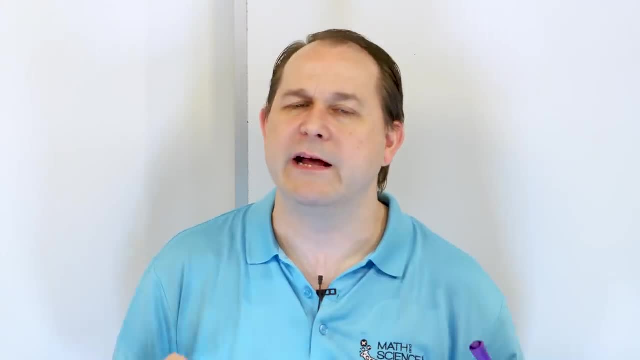 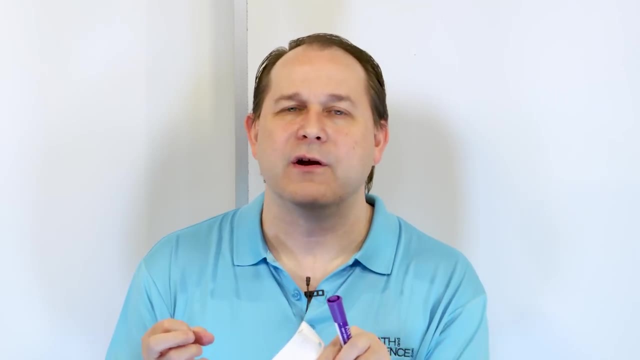 it. If you twist it up into like a twisty and then pull on it, it's very hard to actually break it. Maybe you can't break it at all. That's because the atoms that are joined together to make plastic are what we call polymers, And they are joined in very long chains that are very strong And those 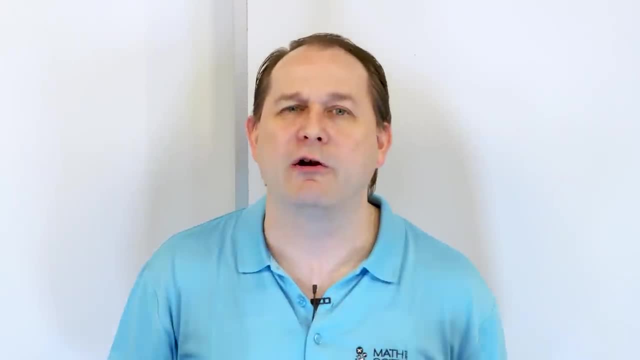 long chains that are strong make it very, very, very hard to break right. It kind of behaves as microscopic kind of rope And it's very, very, very hard to break And it's very, very, very hard to break. 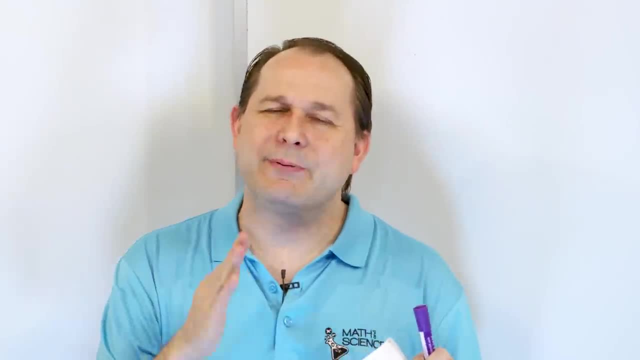 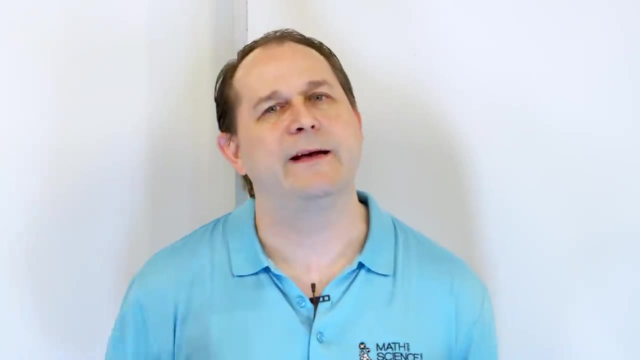 inside there, but also very flexible. See, plastic is very flexible, but yet it's extremely strong if you try to break it. And so we have a ton of uses for plastic, something you may take for granted, right. Other things- you may look around the house. you know even the aluminum foil, the sheets of 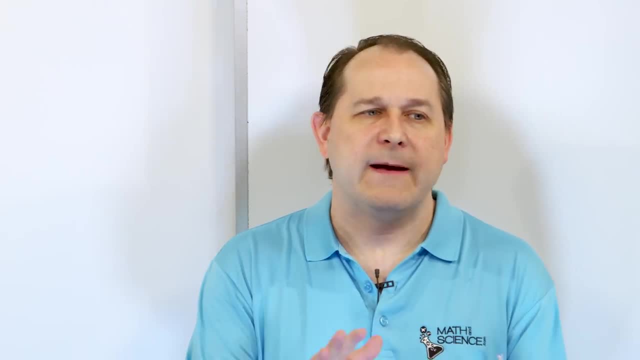 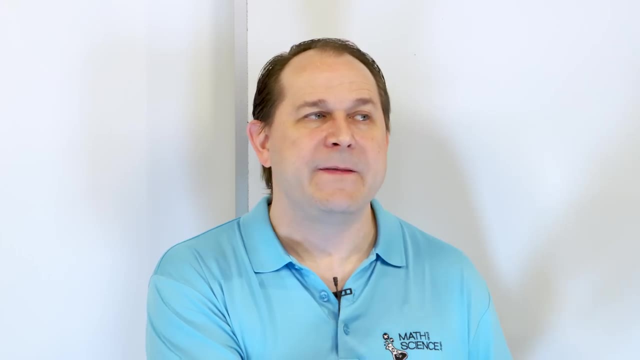 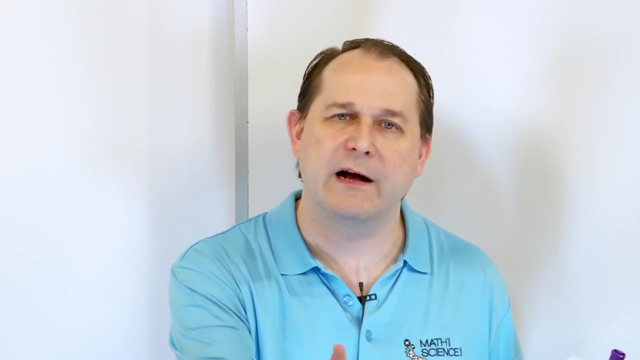 aluminum foil that you have, that maybe you cook with right. That was pressed into a certain shape and there's a certain chemical process to take the ore out of the ground. that is not pure aluminum, by the way. It's aluminum bond. It's something that's bonded to something else, maybe bonded to oxygen or something, And we have to remove the oxygen and get the pure aluminum out of it and make these pure sheets that we can then cook with right. 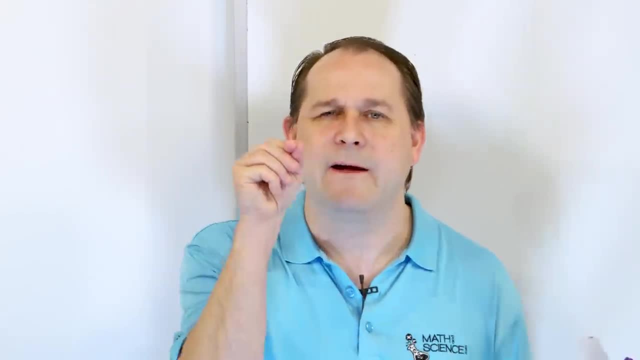 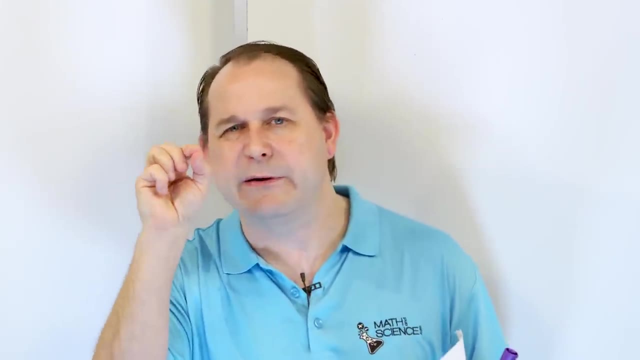 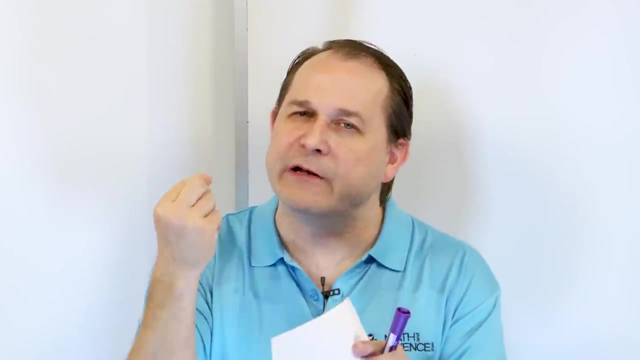 I can go on and on and on, all the way from simple things like this to the tip of the matches. If you take a match from your kitchen and strike it, if you look at the end of the match, there's the material that's on the end of that match. It's got sulfur in it, It's got some other stuff in it And it's designed so that if you give it a little bit of friction and a little bit of heat, then that matches. 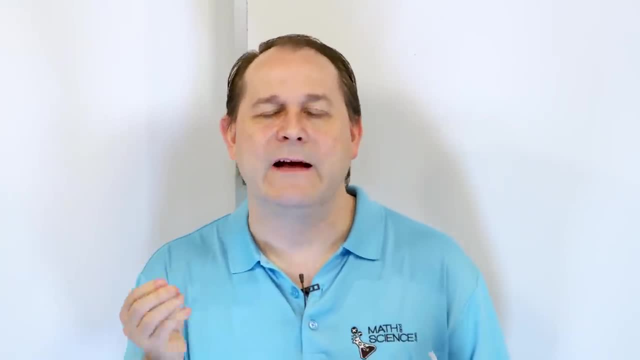 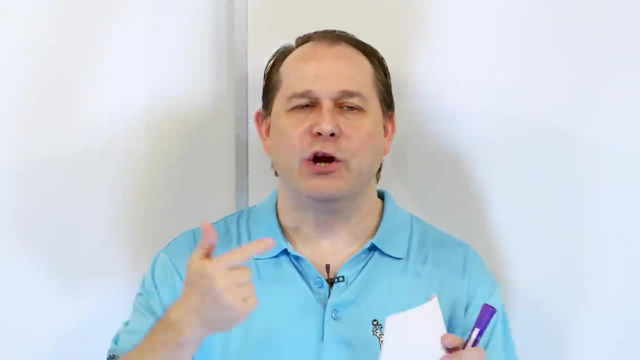 And that wire at the bottom of the match burns. That's a chemical process. someone designed to fit on the tip of a match inexpensively so that we can use it to make fire quickly. So plastic fire, you know. we talked about metals like aluminum, also up to very advanced things like rocket engines, right? 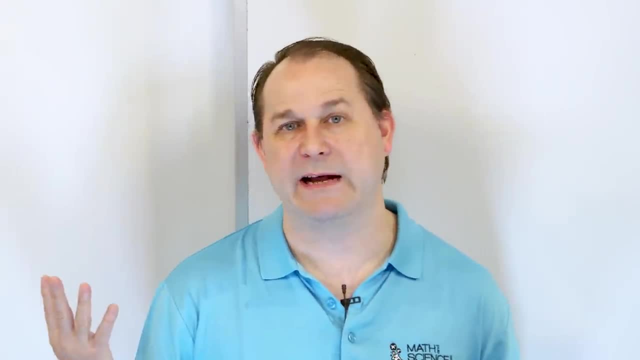 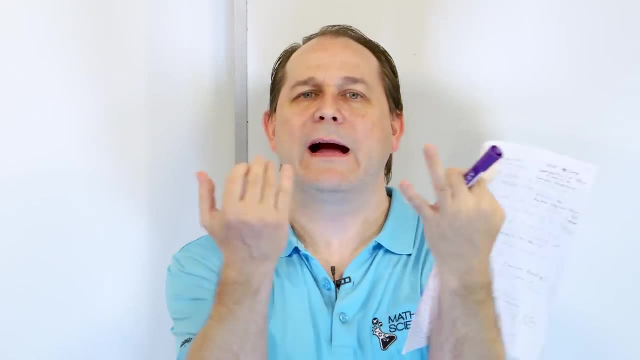 You take hydrogen, which is the lightest, most abundant element in the universe, and you combine it with oxygen, right? So hydrogen is a gas, Oxygen is a gas. You combine it together. What happens? You get a flame, You get an explosion. 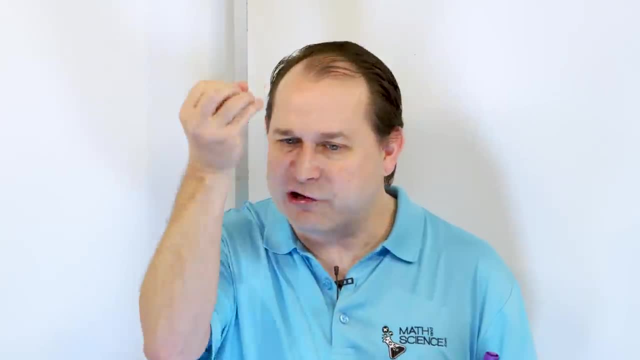 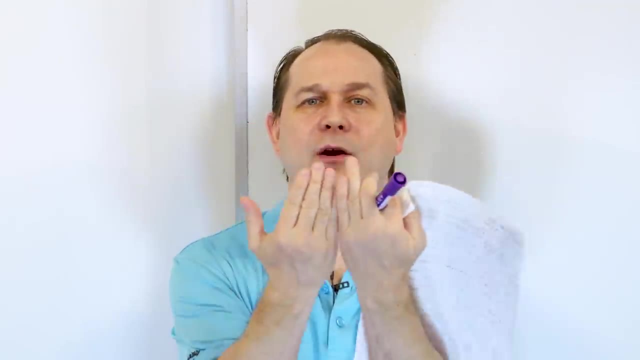 really. and if you put that inside of a rocket engine then you generate thrust because of the heat, you know that's produced in it, all the water that is formed, because hydrogen plus oxygen makes water, h2o right and that flows out the back of the rocket and produces thrust. you know i worked at 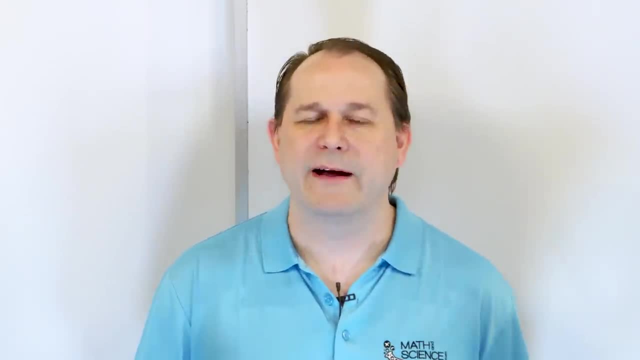 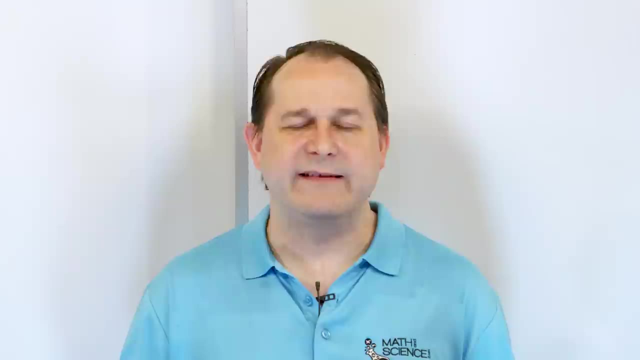 nasa for many years. so that's near and dear to my heart. but you know, chemical processes stretch all into even into space travel, into everyday life around you. so the thing i like about chemistry is that once you understand the basics of what you're doing, you can actually see it in action. 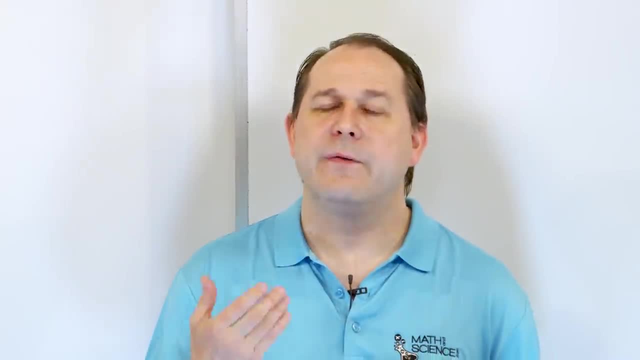 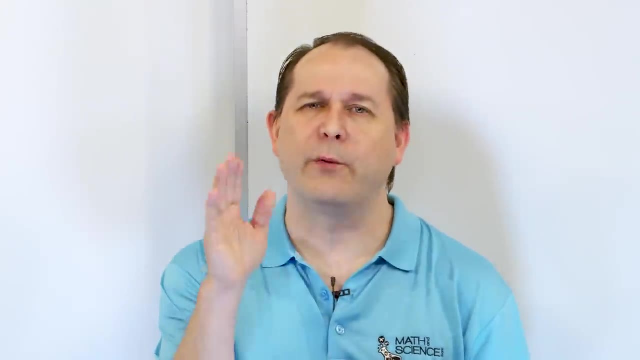 all around you. it's very hands-on, and so that is one thing i really wanted to impress upon you. now we have a ton of stuff to cover, a ton of stuff to cover. but real quick, before we go any farther into definition, just give you a couple more quick examples you may have seen. 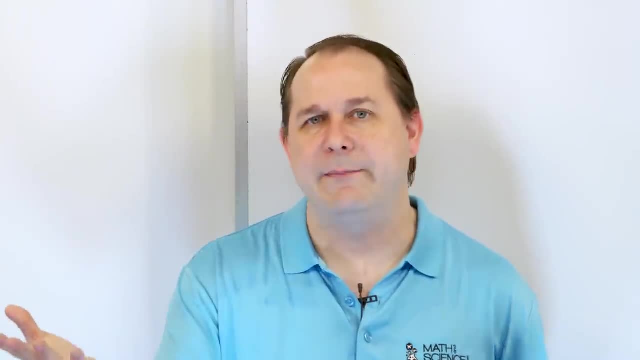 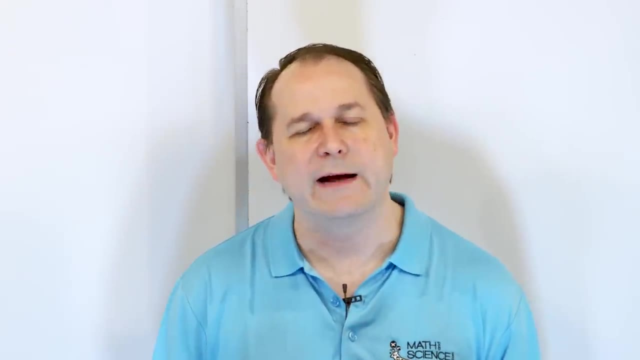 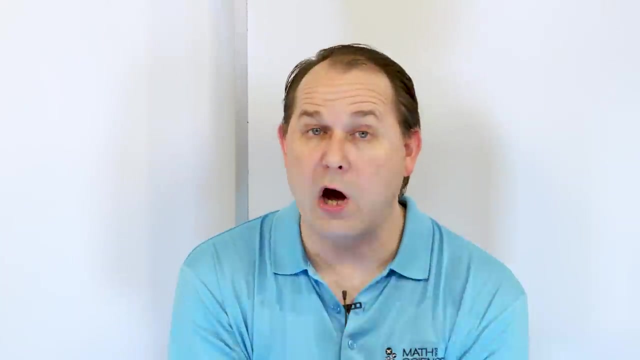 baking soda in your pantry or in your your cabinet, making soda and vinegar. and if you mix baking soda and vinegar, you see the bubbling of the carbon dioxide gas. right, that is a chemical reaction that's going on, just like if you take hydrogen and oxygen and put a flame to it, you get water. that is a chemical reaction where the two different 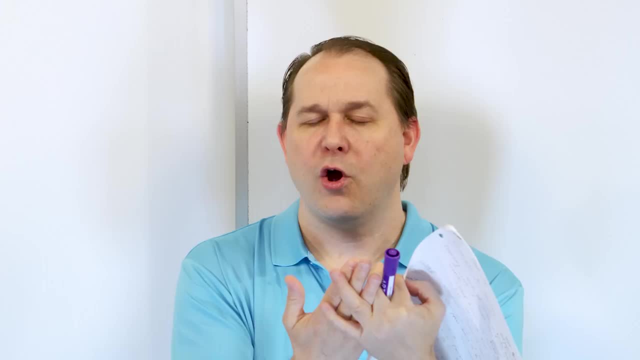 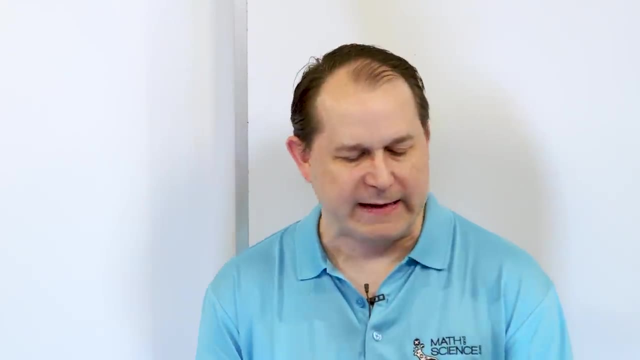 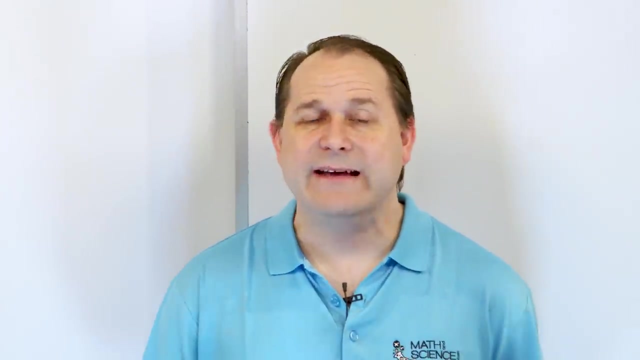 kinds of atoms come together and make a new substance or a rearrangement. in that case it was water, but in the case of baking soda and vinegar you see the bubbling of the carbon dioxide gas. you know, we talked about the uh, the matches in the sulfur and so on. now the good news is that. 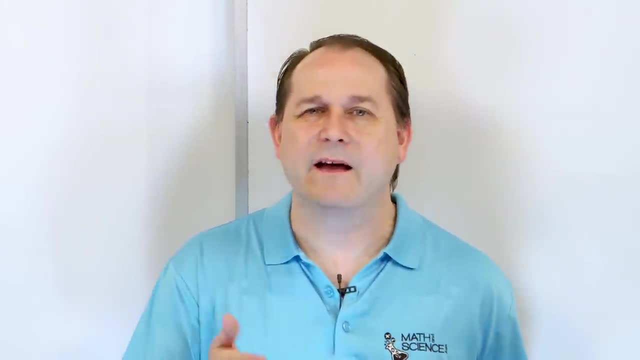 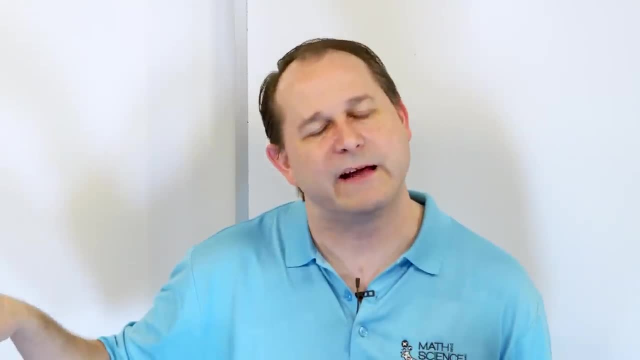 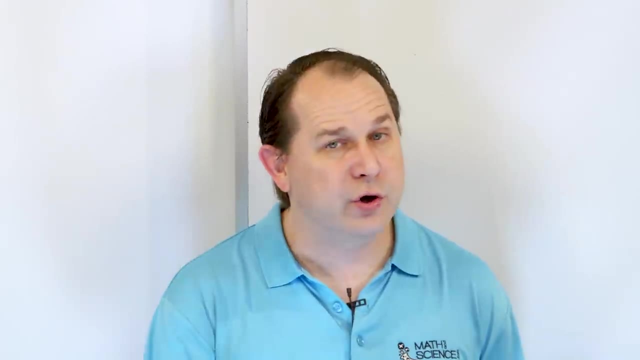 i mean, sometimes you have more advanced equations, of course, when you get into advanced chemistry. most of the time it's it's pretty simple arithmetic though. so the math should never hold you back. what what could hold you back is if you start trying to solve a problem. 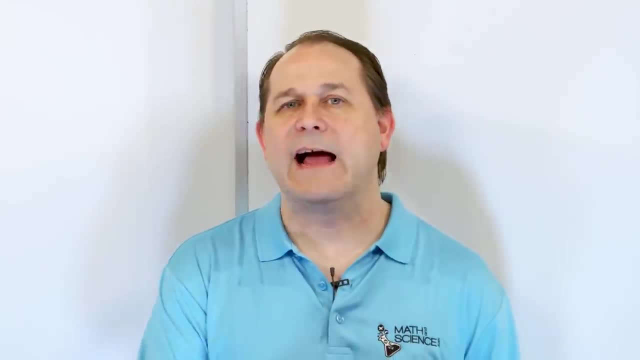 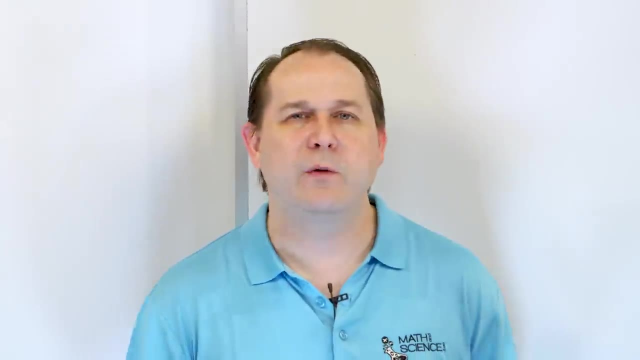 without knowing what the problem is asking. so in this class, we're going to learn how to read a chemistry problem. how to pull out the information that is required. how to read a chemistry problem: how to pull out the information that is required. how to read a chemistry problem. how to read the way in which we should get the solution in the correct way. 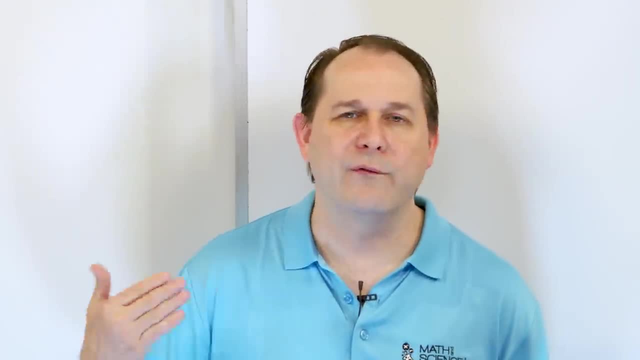 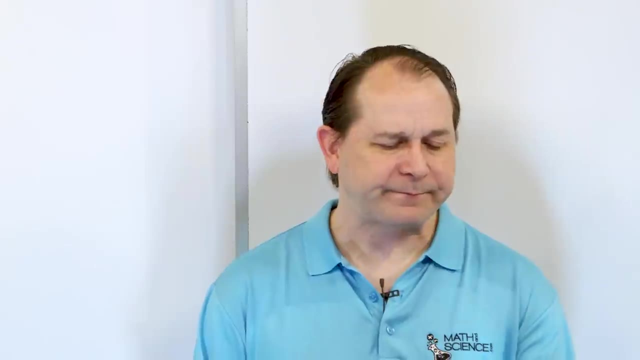 and also how to check our work. and by doing that process over and over and over again, you will get good at solving chemistry problems, and i hope that it will also be enjoyable along the way. all right, so let's jump into the bulk of this. this is just sort of the introduction. now we 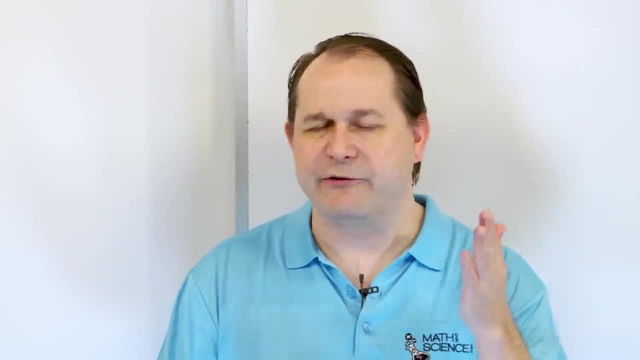 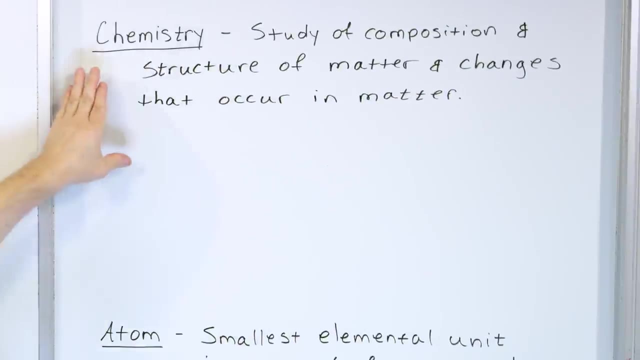 need to really talk about chemistry a little bit more. we talked about why studying chemistry. let's talk about what is chemistry anyway. my definition of chemistry is of what is chemistry. now, this is my definition of chemistry. your definition may be slightly different. if you have a textbook, the definition and the textbook will be slightly different. 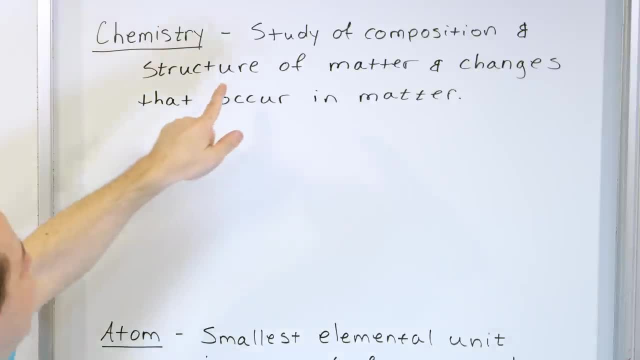 there's different ways to define chemistry. my definition is: chemistry is the study of the composition and the structure of matter and changes that occur in matter. it's a short, little definition, but basically what we're trying to say here is that chemistry is studying the composition of matter and as we react to things together in a chemical relationship. we're going to 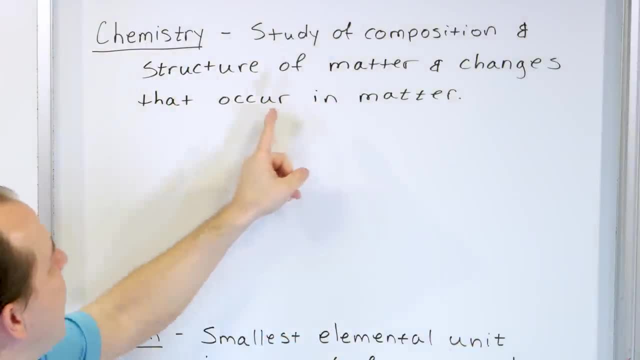 have a reaction. how does that matter? and the structure of matter change because we have the word changes here. so i'll give you a good example. we take sodium right, which is a- uh, a metal on the periodic table. we're going to talk about the periodic table in a minute. it is a metal that. 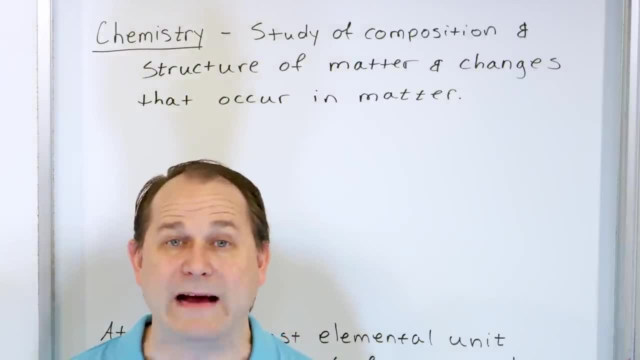 is so reactive that if you drop it into a bowl of ice water it will catch on fire. it will, it will have a chemical reaction with the water and a lot of heat will be created and there will be a flame. that is actually produced, especially if you drop it into a bowl of ice water and it will catch on. 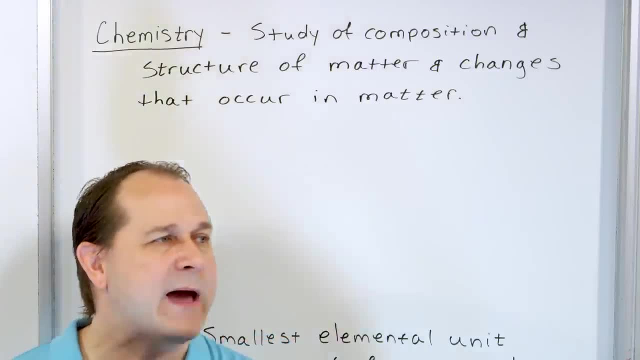 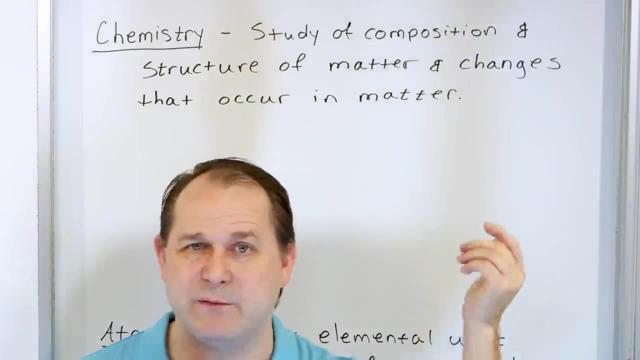 fire. it's part of that. you don't want to be eating any pure sodium. and then you have chlorine, right, chlorine is a uh kind of a yellowish looking gas that will kill you. if you inhale it. you die. okay, sodium and chlorine obviously are two totally different things that are not uh, seemingly. 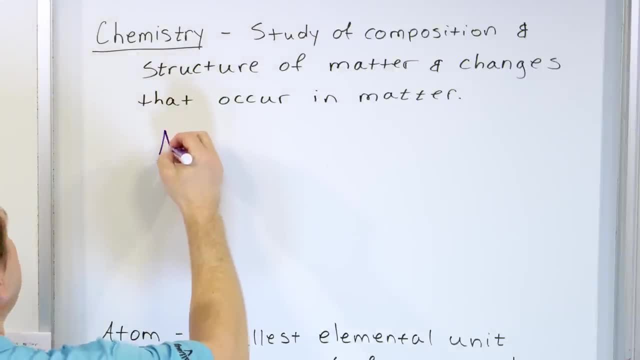 related to each other now. we're going to talk about this in a minute. why does sodium have the symbol in a? we'll talk about that in a little bit. sometimes the symbols don't exactly match up with the letters we use to represent them, but if you take sodium and you put sodium in a bowl of ice, 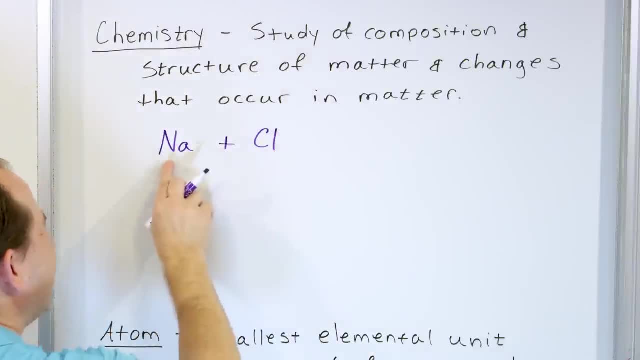 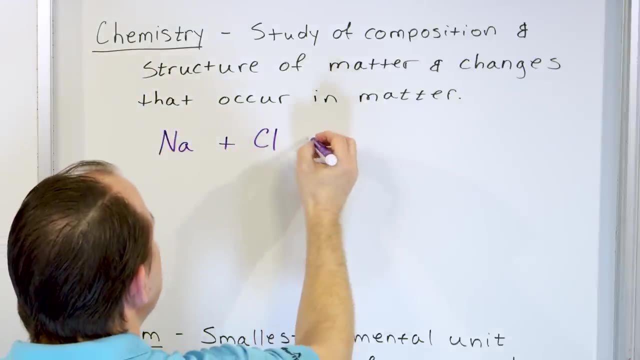 water and you combine it with chlorine. these are two things that basically would kill you. if you swallowed pure sodium, you would have some sort of reaction in your stomach. it wouldn't be pleasant, i promise you. chlorine will kill you, but whenever you mix it together it forms something new, bonded. 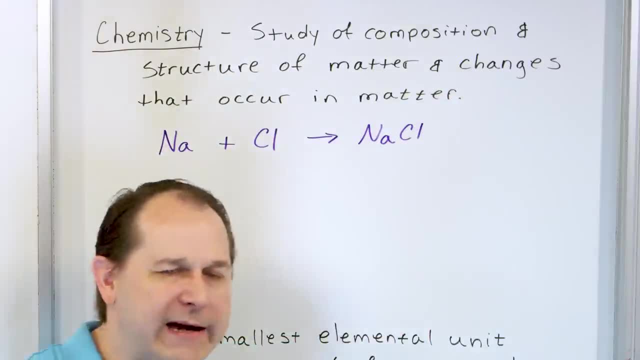 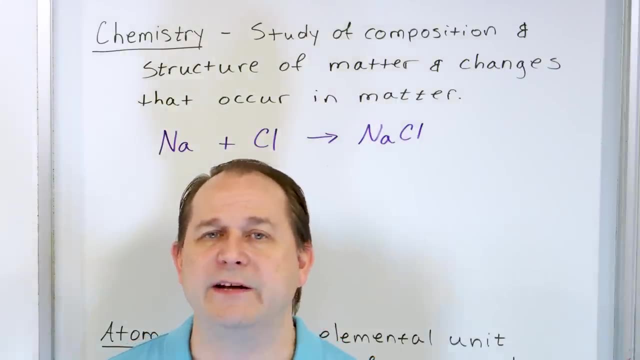 together called sodium chloride, and sodium chloride is what you eat every day in table salt. not only is table salt tasty, but it's actually required for your body to function properly, because when you eat the salt, your body breaks down the sodium and the chlorine in the micro. 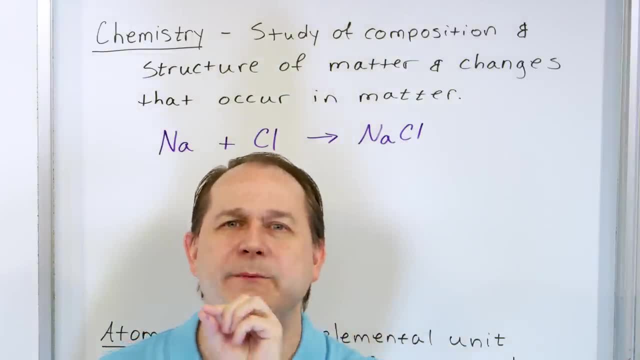 scopic quantities that won't hurt you, but those uh, sodium and chlorine uh entities in your body. they are used in the function of your nerves and your brain and you know all manner of uses inside of your body. but the point i'm trying to get at here is sodium is something you don't want to eat. 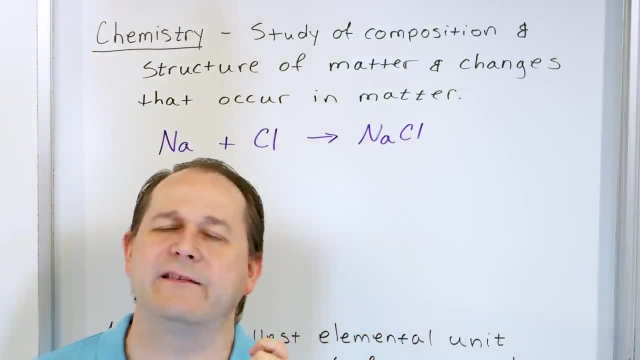 chlorine is something you don't want to eat, but together, sodium chloride, has a totally different character. it is a crystal that is kind of shiny. you've seen what salt looks like under a microscope, right, it's a little shiny little crystal, but it's perfectly fine to eat. in fact, we 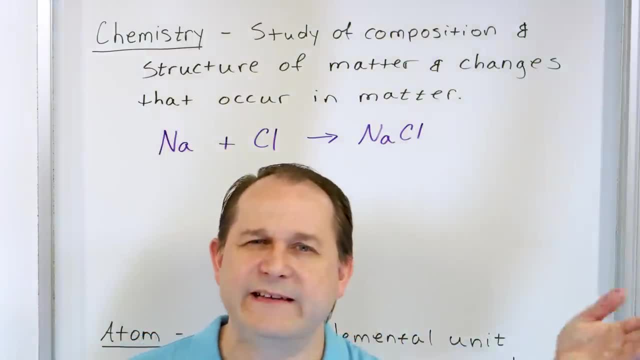 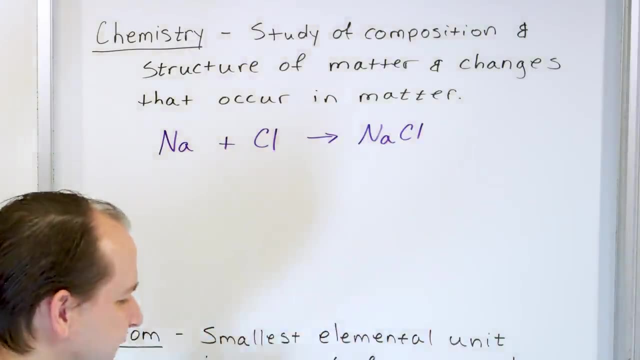 eat it to survive. it's salt, right? so when you put things together, the atoms are rearranged into some product that has a totally different set of characteristics compared to what goes into this guy, right, and this is what i called a chemical reaction, as we recombine things in different ways. 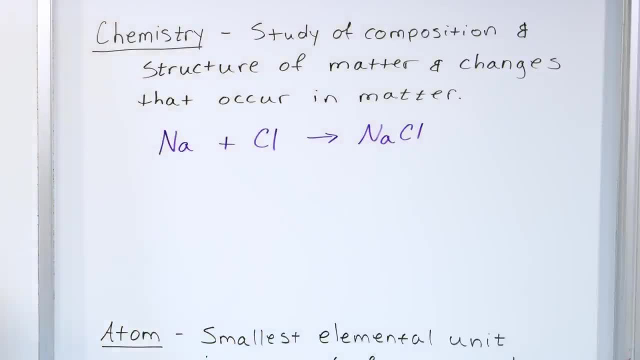 we have new products that are formed which we then can use, and that we that have different properties than what we started with. all right, what about? i'm just going to write it in word words: wood burning, right? so what i mean by wood burning is there. there are chemical, uh, chemical compounds. we'll 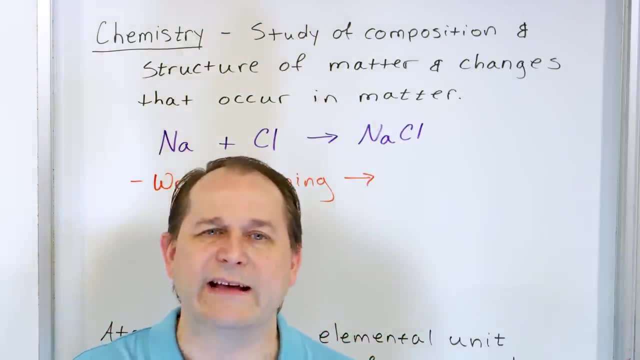 talk exactly what the word compound means in a minute. inside of wood that contain long chains of carbon, right lots of different ones- and whenever you add oxygen to wood, of course we have a atmosphere full of oxygen and you add heat to it, we get the familiar- uh, the familiar- idea of 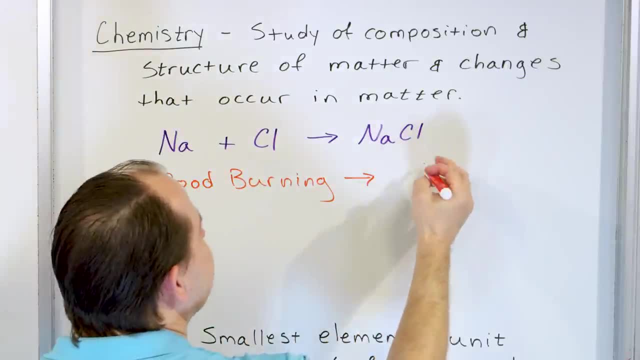 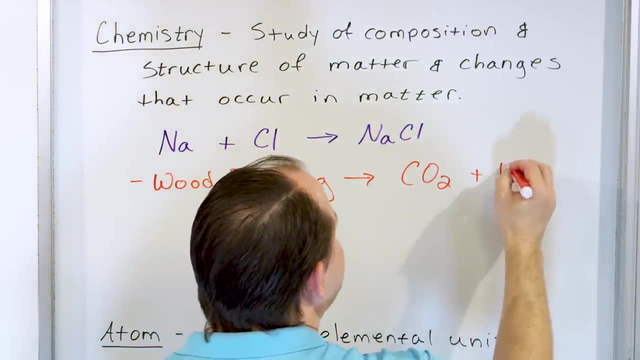 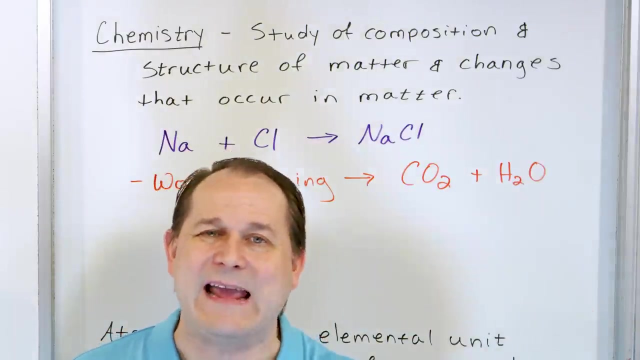 burning wood. right, and what do you get? when you burn wood, you get a new rearrangement of what you started with. you get co2, which is carbon dioxide gas, but you also get h2o, which is water. almost everything that burns that has uh carbon in it is going to produce carbon dioxide and h2o water. 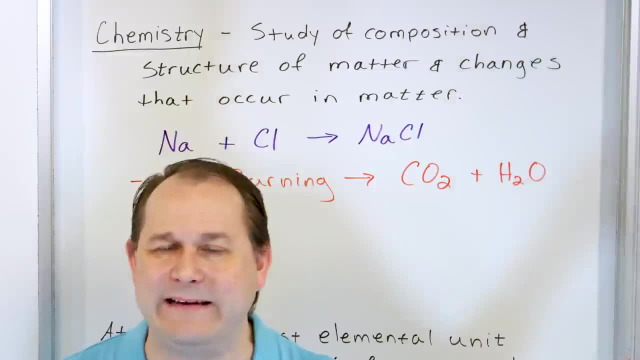 we're going to talk a lot in the future as to why these things are almost always produced, but the point is is wood doesn't look anything like a carbon dioxide, which is a gas. wood doesn't look anything like water, which, as it's floating up from the campfire, is a gas. but when you combine it with 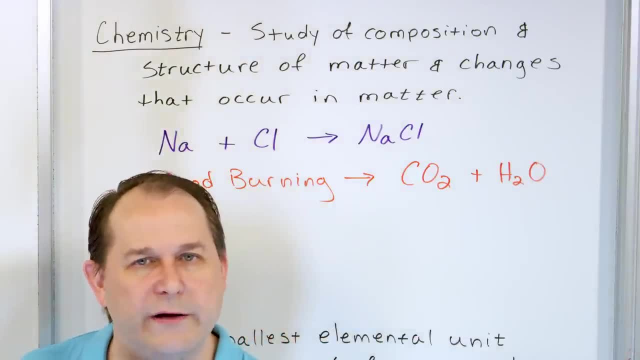 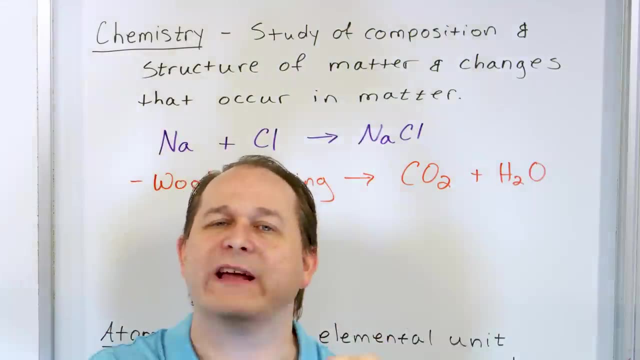 the oxygen and you add a little bit of heat, those atoms that are in the wood, the carbon and the hydrogen and the other things that are in the wood. they can be combined with the oxygen from the air and rearranged in a different structure than what we started with and that has totally different. 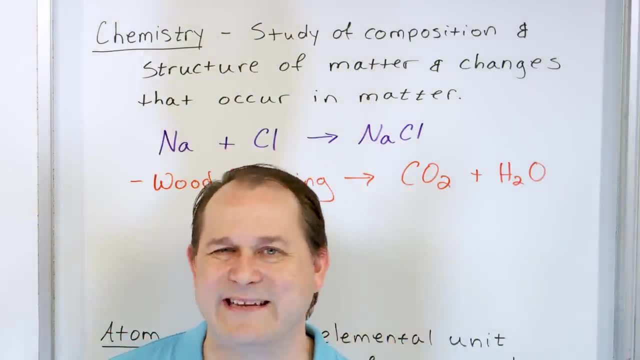 properties. carbon dioxide is a is a colorless gas that floats away. of course, we breathe out carbon dioxide as well from the respiration of our own cells, which produce carbon dioxide as a as a waste product as well. much like wood burning, it also produces water, which, of course, is totally different as well. so these products are a. 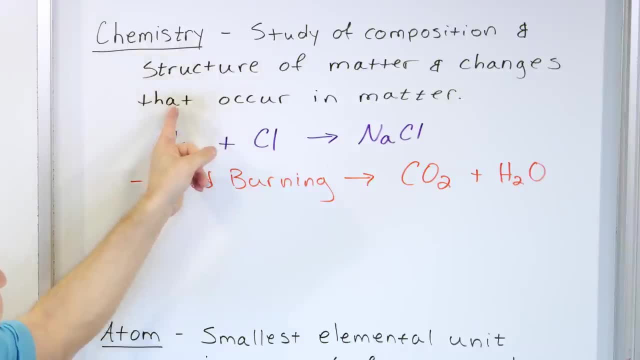 rearrangement. so we say chemistry is the study in the composition of structure of matter and changes that occur in matter. the changes that occur are because the atoms rearrange themselves and form new products with different properties than what we started with. all right, another example would be: 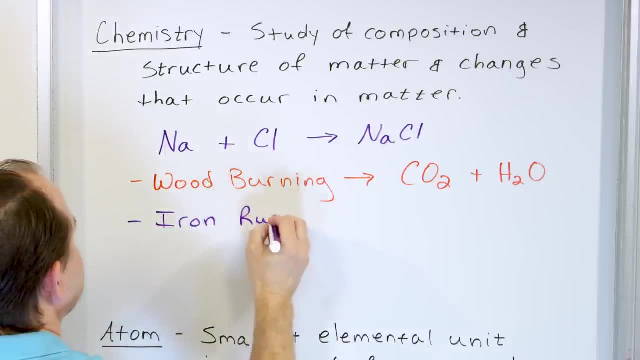 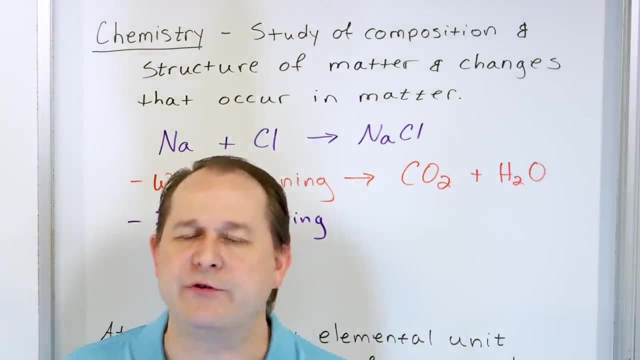 iron rusting right. if you take a, a bar of iron, throw it in the yard, iron might be, you know, shiny when you first get it. if you polish it really good, everything looks great and you throw it in the yard, leave it there for a few weeks and go back, then the iron bar will not look beautiful. 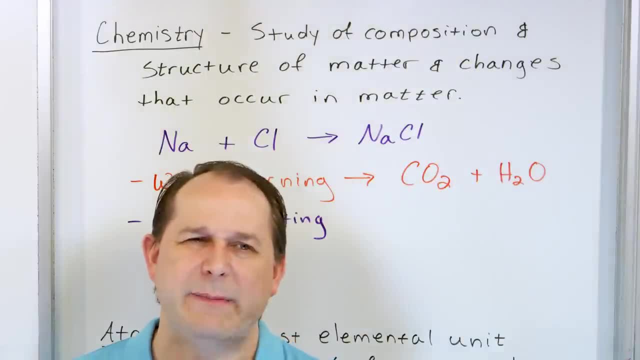 anymore. it'll look a little brownish, a little bit, uh, maybe not as lustrous as it used to be, and if you start scraping at it, that brown substance will kind of flake off. that's iron oxide, right? that's the iron that has now been combined with oxygen to form something new: iron oxide. and that iron. 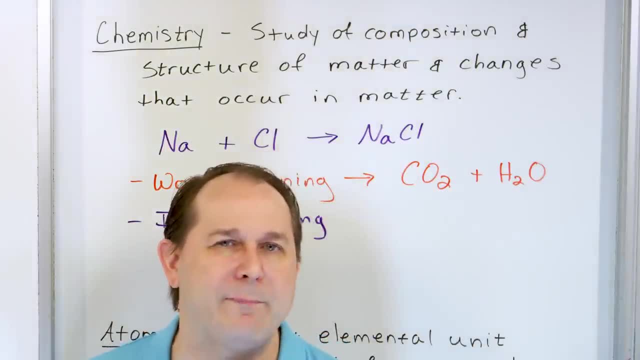 oxide is not strong and doesn't have the same effect on the environment. it's not strong. it's not the same properties as the pure iron. it is different properties because it's now combined with oxygen. so it's a rearrangement of the atoms, right? and then, of course, we have the famous the. 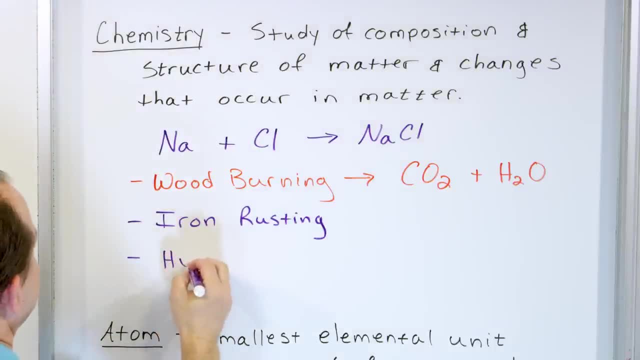 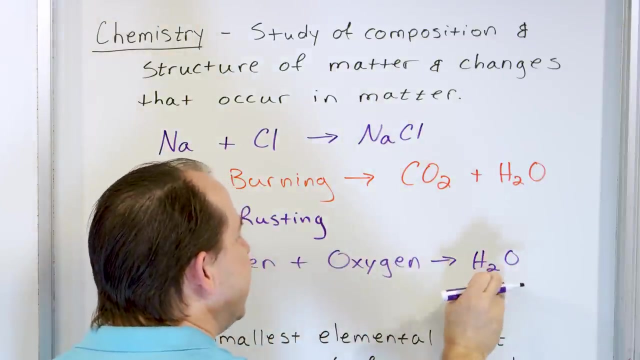 big one, the, the super important one. we have hydrogen right, and then we add to it oxygen, right, and of course we have add a little heat. and what do we get? we get h2o and this is rocket fuel. hydrogen plus oxygen. uh gives you water and you also uh. 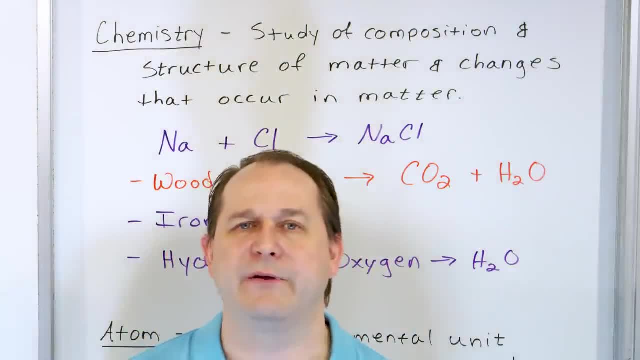 have heat that comes out of there, and the water is expelled out very forcefully, and so you have an explosion. that's basically going on as well. all right, so that is what chemistry is: it's a rearrangement of these, of these things that we haven't talked about yet, but they are atoms, and 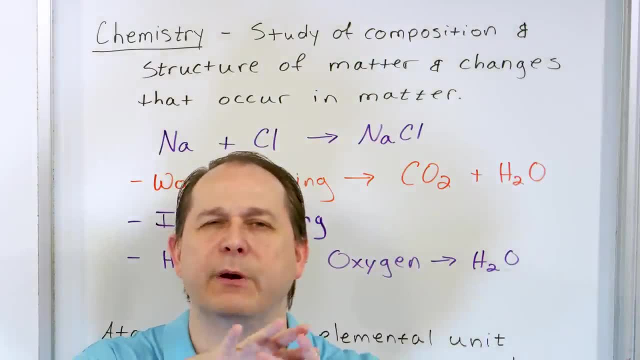 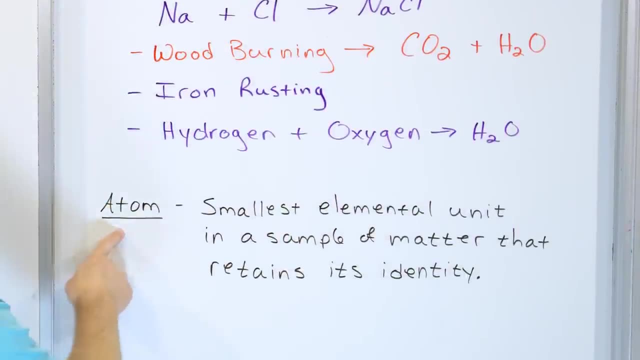 they are the most indivisible- uh, i shouldn't say indivisible- they are the most elemental, fundamental thing that everything around us is made up of. and that brings us to our second definition: what is an atom? anyway, it is the smallest elemental unit in a single atom, and it's 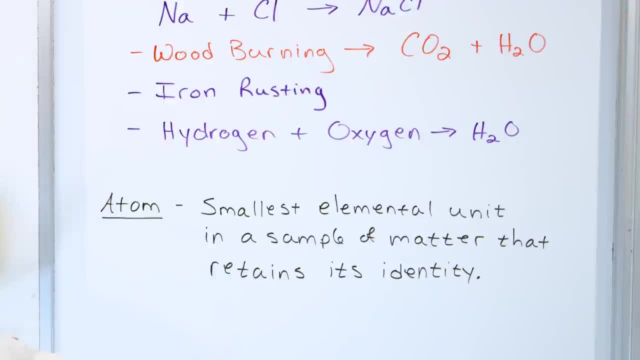 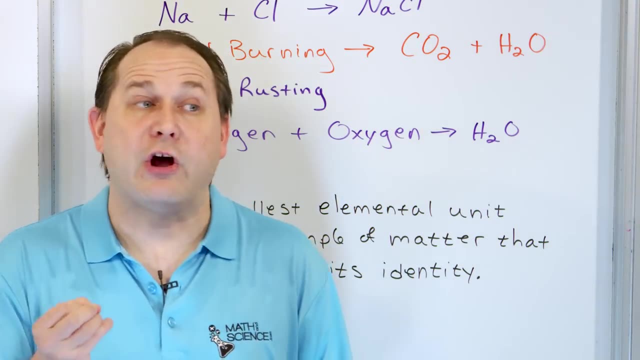 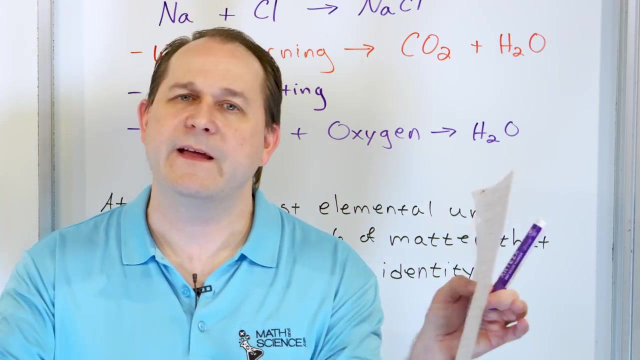 a sample of matter that retains its identity, and that sounds weird. what does it mean to retain your identity? what it is? what i mean by that is a long time ago, people, you know, people- saw carbon dioxide, they saw water, they saw carbon monoxide, they saw sodium chloride, they saw all of the things that. 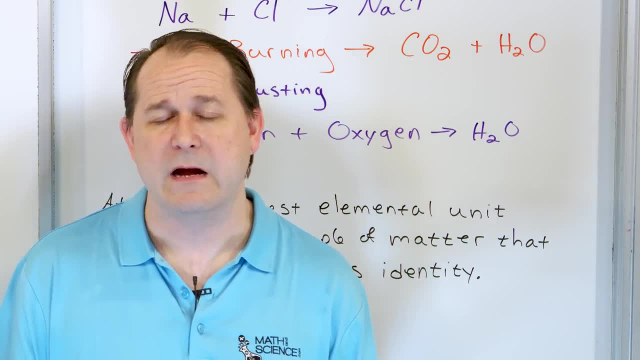 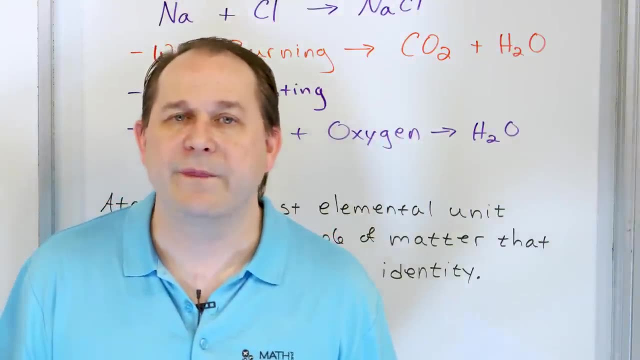 existed in nature and they all look like completely different substances, right, because water looks totally different than hydrogen and oxygen, and so obviously they thought they were totally different things. but after a lot of investment and a lot of research and a lot of research and a lot of. 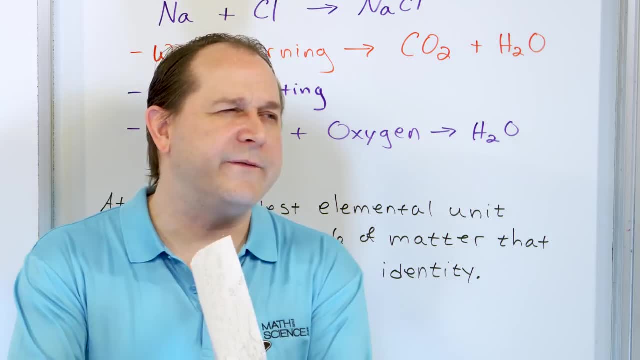 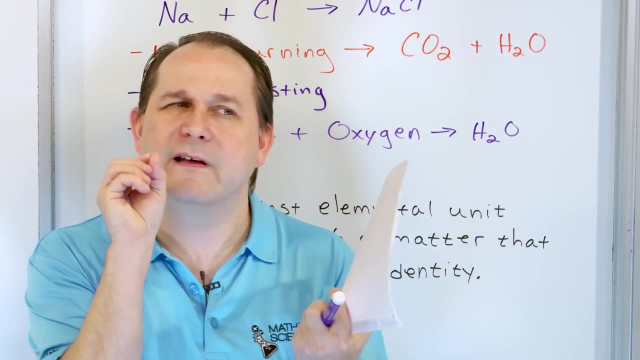 investigation we figured out that everything around you, all of the very different things that we think are so different around us, are really just a rearrangement of these little. at the time they thought they were indivisible. we'll talk about that in a minute. but these small little 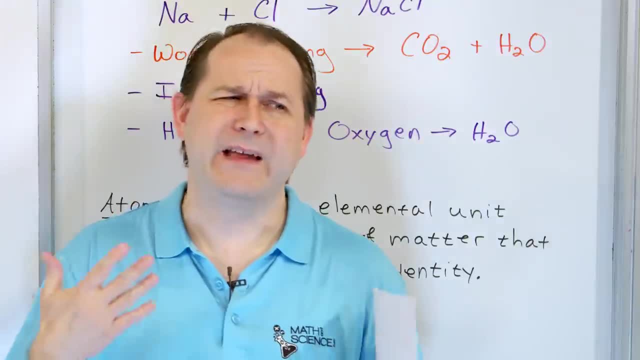 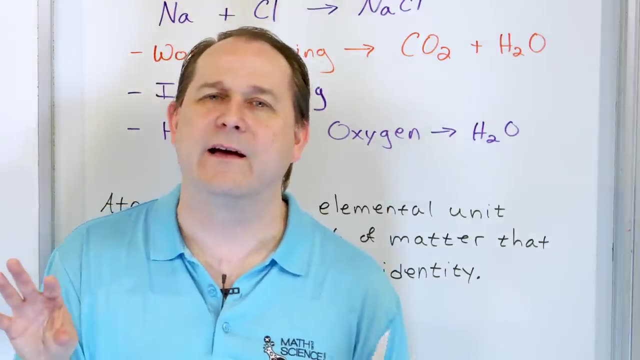 indivisible things, which we call atoms, and now we know that there are about a hundred different types of atoms. in reality, there's about 118 that we have created because the the really heavy uh atoms are, uh, not really naturally occurring. we have to create them in a lot of different ways. 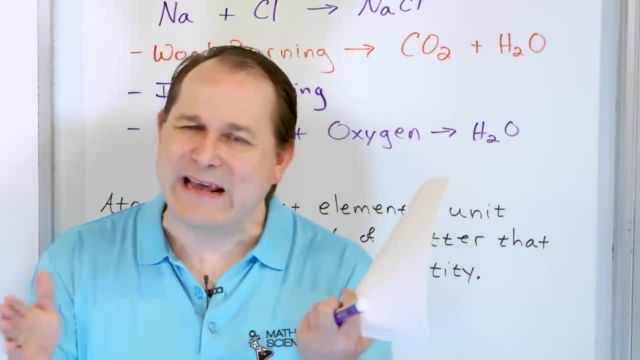 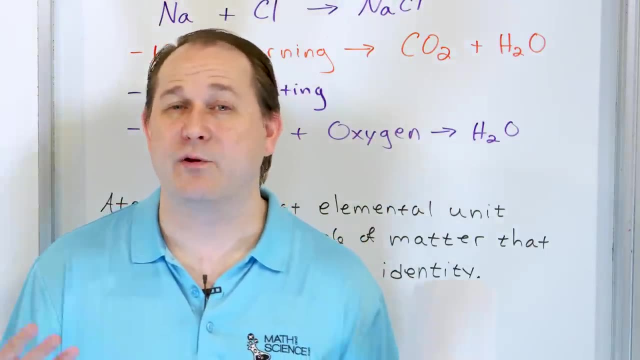 in the laboratory and they don't last very long. so at the very end of the periodic table, the very heaviest atoms are things that are not, uh, really very stable. they don't exist in nature. maybe they're radioactive, so you can count those if you want, but they're not things that we're going to. 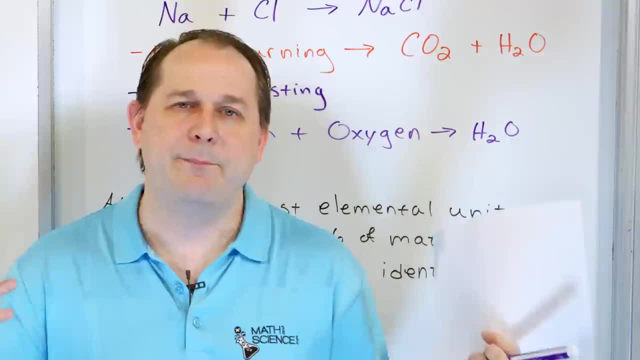 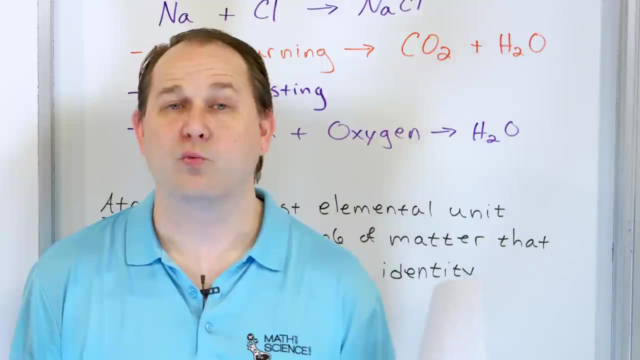 study in this class. in the bulk of the periodic table it exists of about a hundred elements that are natural and stable, and the point i'm trying to make here is that all of the things that look so different around us are really just different combinations of those roughly hundred different. 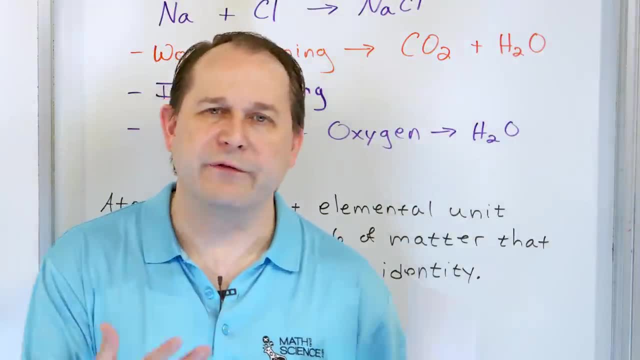 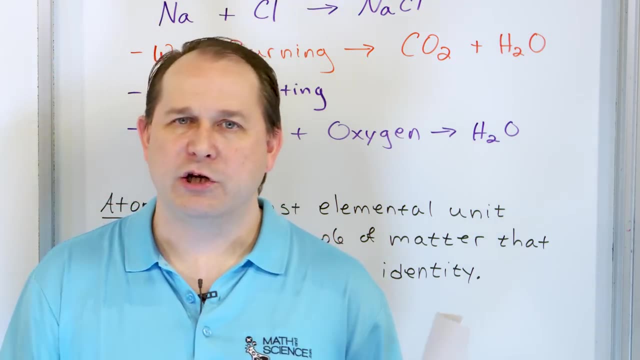 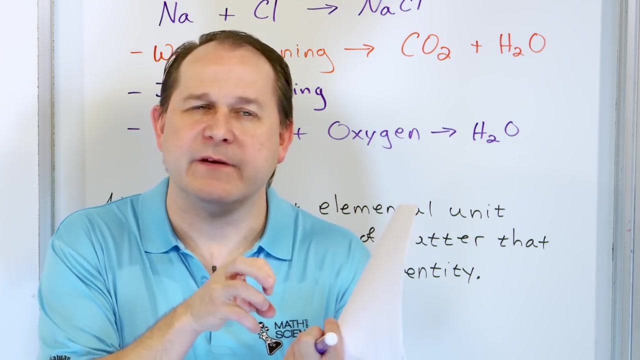 elements. of course there's a few more in reality that we've discovered, but those are the ones that are common, right? nickel, iron, hydrogen oxygen, chlorine. i can go on and on- uh, lead. those are the atoms which were also called elements on the periodic table. those are the fundamental things. 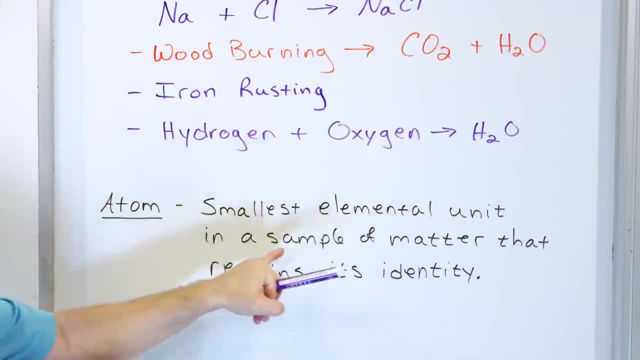 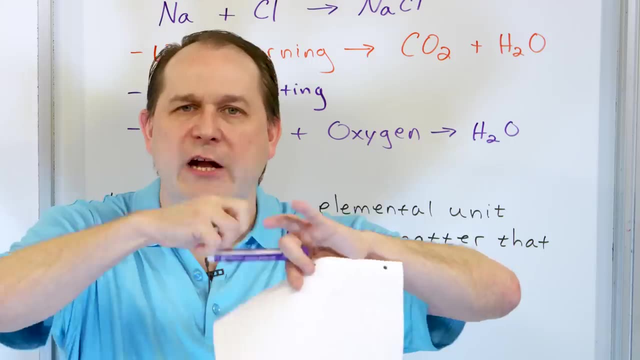 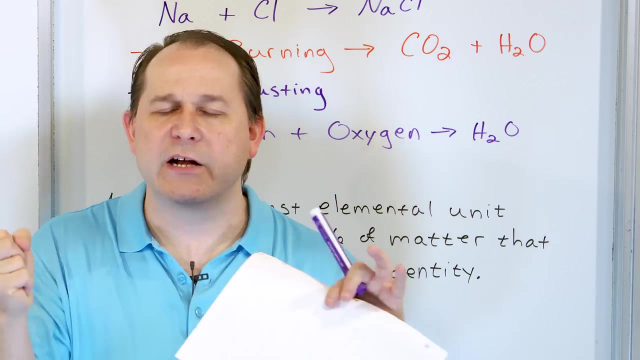 that? what do we say? smallest elemental unit in a sample of matter that retains its identity? what do we mean by that? if i take a sample and start cutting it in half and cutting it in half like a bar of of pure aluminum, let's say i cut it in half and cut it in half, eventually i'm going. 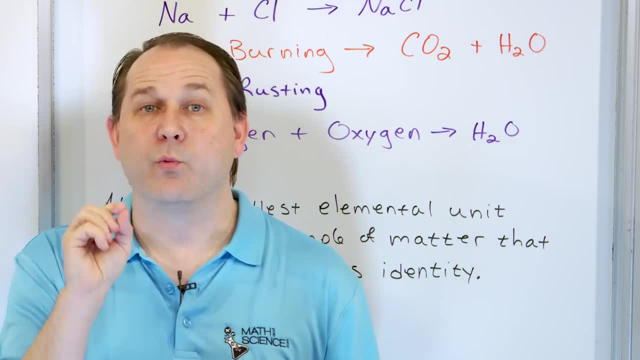 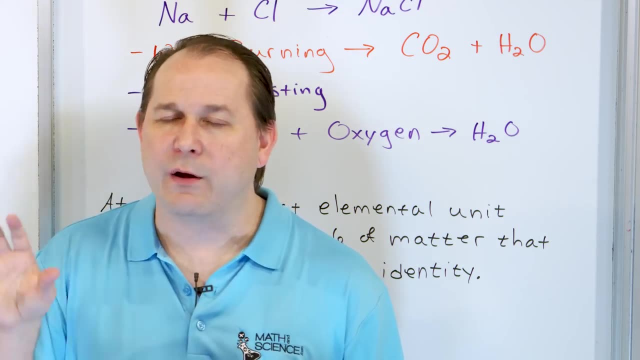 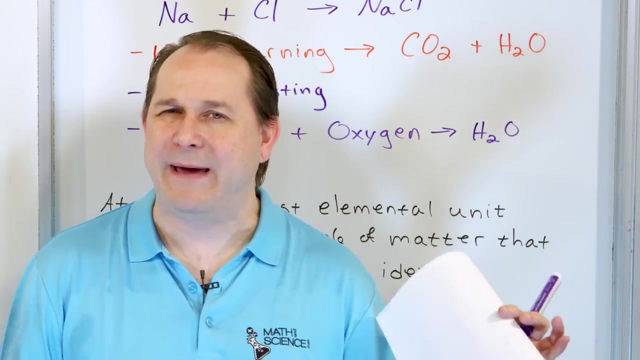 to get down to a single aluminum atom and that atom. we're going to learn a whole lot more about how atoms are, modern theory of how atoms are constructed later, but for now just know that if we try to take that atom of aluminum and break it in half, then we don't have anything that behaves. 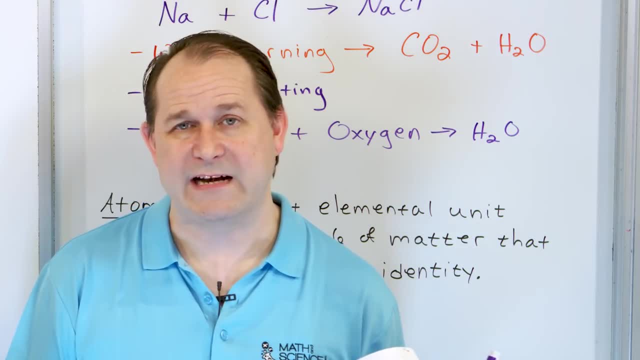 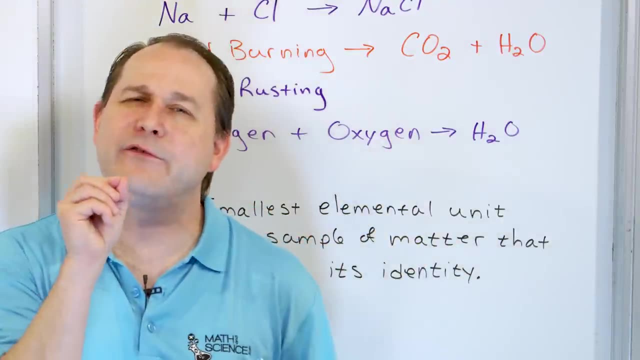 like aluminum anymore, so we have something smaller than an atom in that case. so we say atoms are the smallest elemental unit in a sample of matter that retains its identity, because if you get down to a single aluminum atom it has all the properties of aluminum. it's shiny, you know, maybe. 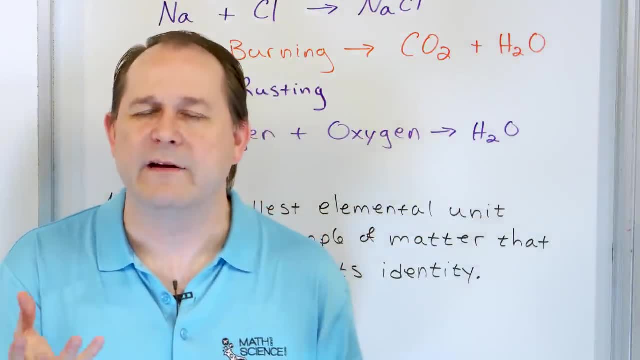 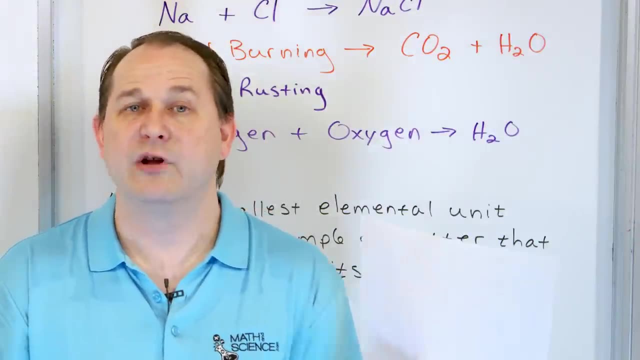 it conducts heat, maybe it doesn't, or whatever the the element is, it has all of the properties of that substance. but if you take a single atom and try to break it in half, then it has no characteristics of aluminum anymore, because you you're now digging inside of the atom. now i'll clue you in, because i 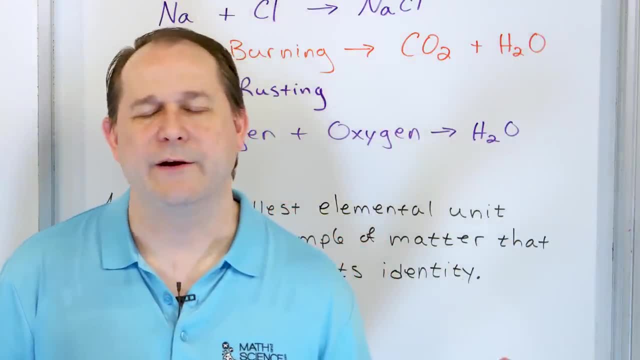 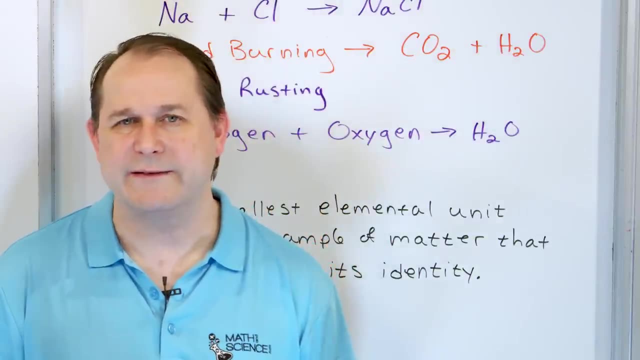 know that you already know anyway, and we're going to get into this a whole lot more in a second, but before we get into this a little bit more later, we now know that most of the mass of the atom is concentrated in the center of the atom, called the nucleus, and those are where we what we call protons. 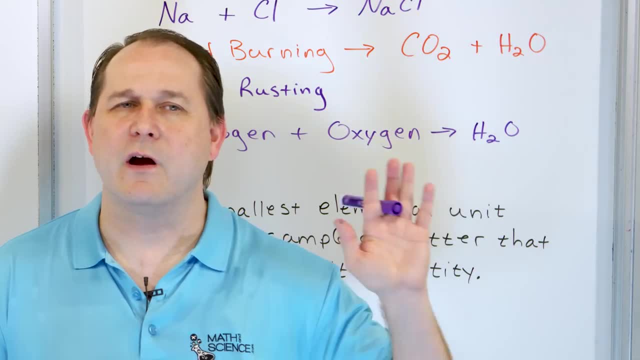 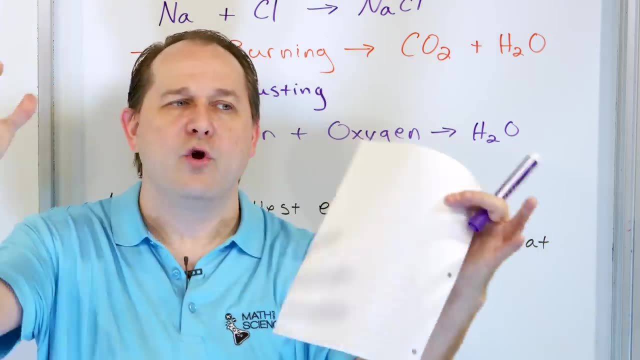 live and neutrons live. we're going to talk about this a lot later on, so let's not get bogged down in it right now. but that is what is in the center of the nucleus right. and then we have the electrons, which are kind of orbiting, and we'll talk a little bit more about orbiting later, but they're in a 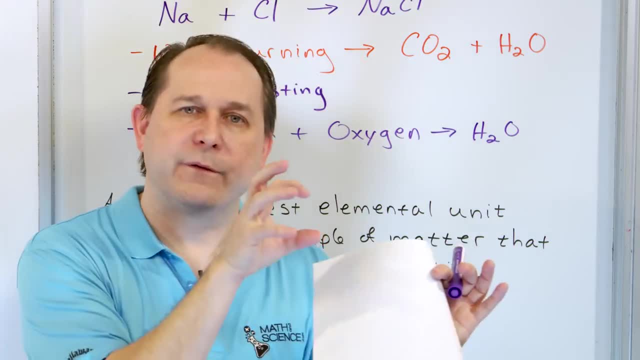 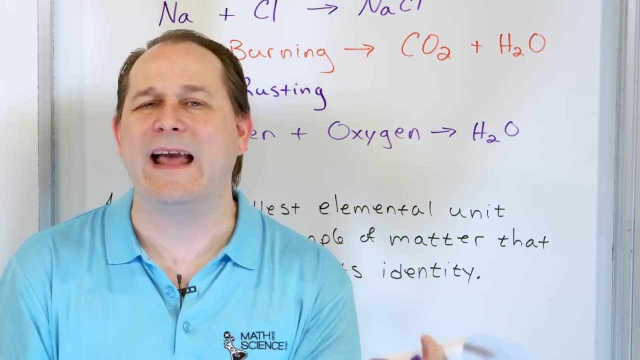 cloud that surrounds the nucleus, and together those, the, the nucleus plus the nucleus and the electrons form the atom. so if you try to split the atom in half, then you don't have aluminum anymore, you have something else, because you now have kind of digging into the nucleus, to the to. 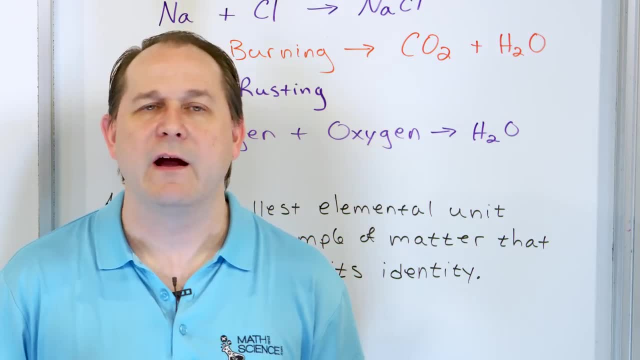 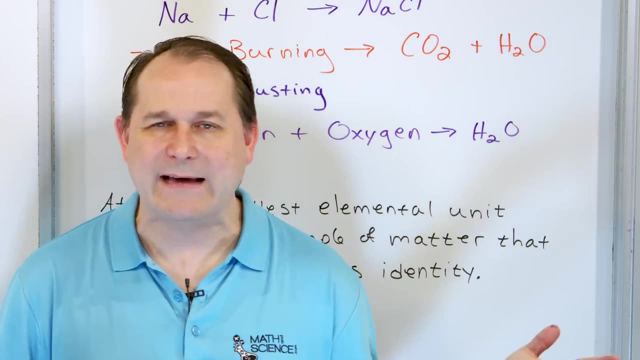 the root of the protons and the neutrons that are in there, and so those are called subatomic particles- protons and neutrons and electrons, because they're smaller than an atom. now, back in the day of early chemistry that we didn't know anything about electrons, we didn't know protons. 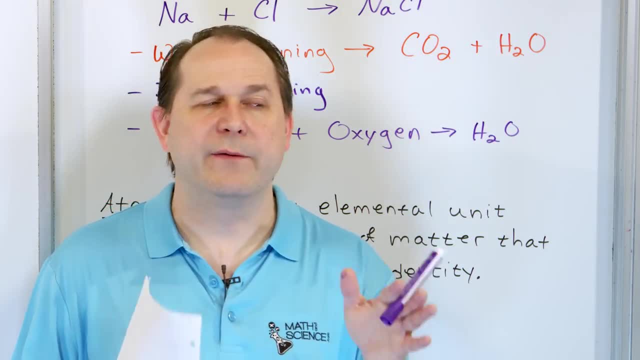 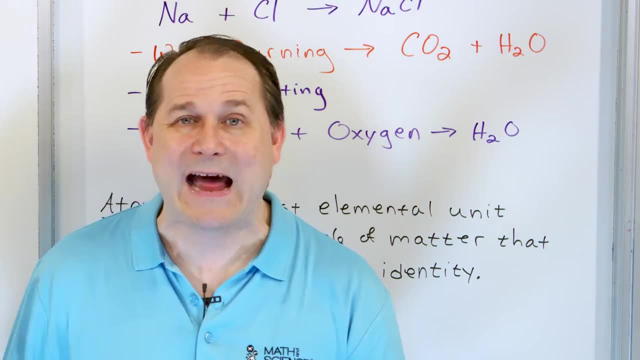 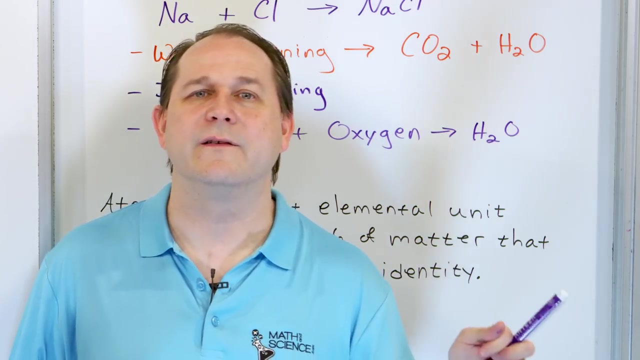 existed or neutrons existed. so the definition they came up with was atoms were the smallest indivisible things that retained its identity. but now of course, we know we can split atoms apart into protons, neutrons, electrons, and we even know now that we can actually even split the neutrons. 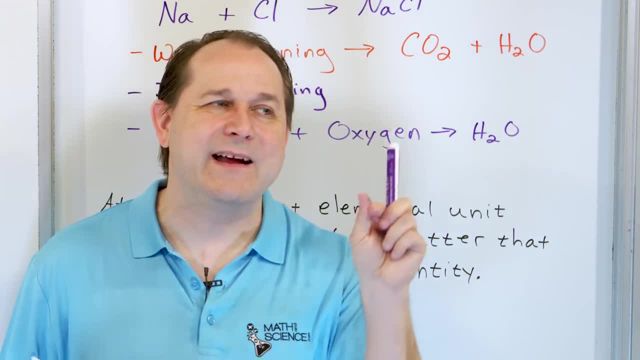 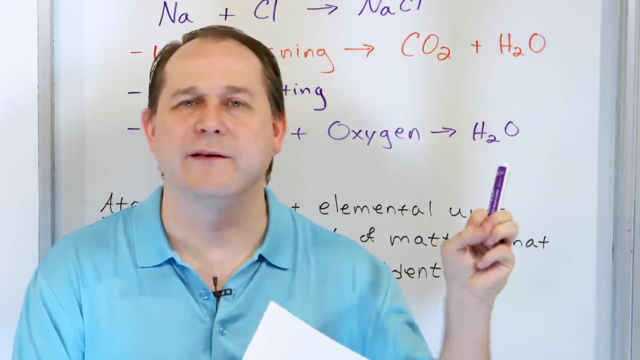 and the protons up into something even smaller than that, and those are called quarks, and i know that sounds weird, but that's a fact. we know that quarks are what make up the neutrons and the protons. it turns out electrons don't seem to be made of anything smaller that we know of they. 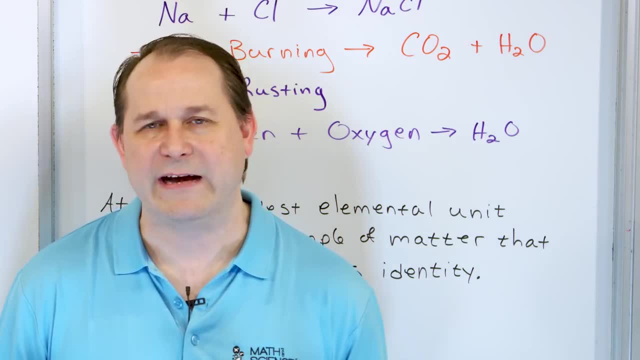 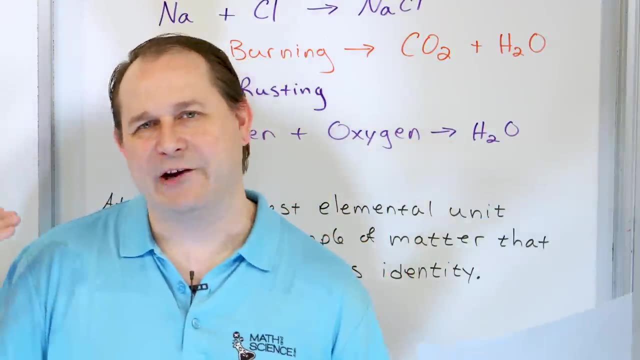 really are indivisible. now i'm going to talk a little bit more about the neutrons and the protons. all of this is our current understanding. it could all change, which leads me to my next point. i want you, as you learn chemistry, as you read your book, as you watch my lectures, i want you to learn, but 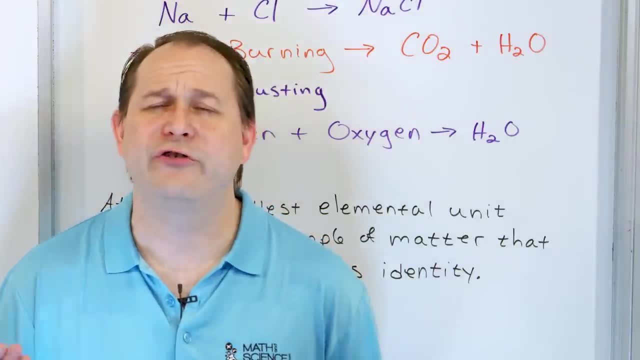 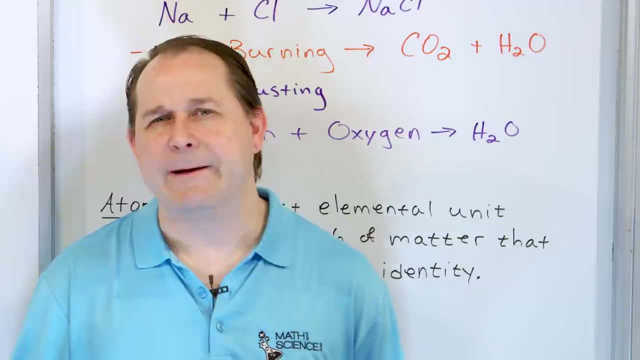 i want you to also realize that we don't know so much about how this stuff works, and i want you to really absorb that, because it's very easy when you read a book to say: well, all this is figured out, i'll just learn it, there's nothing else to learn. 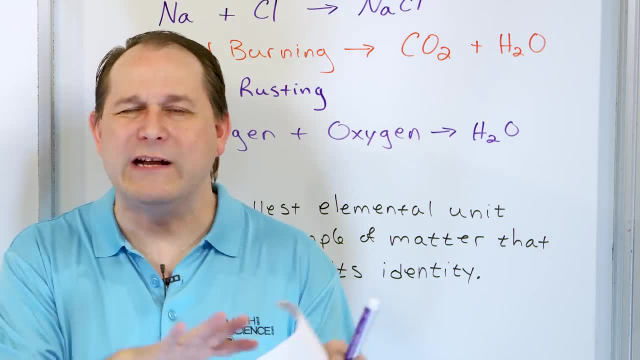 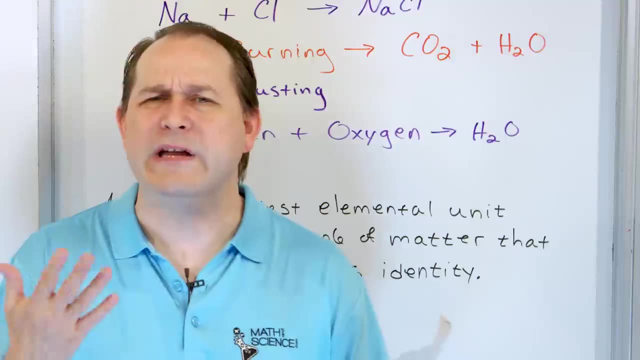 but actually when you dig a little deeper than the surface layer on anything, you will realize that we don't know anything about how this stuff really works. what i mean by that is a little silly. of course we know some stuff, but the details of how the electron behaves in the atom we don't really. 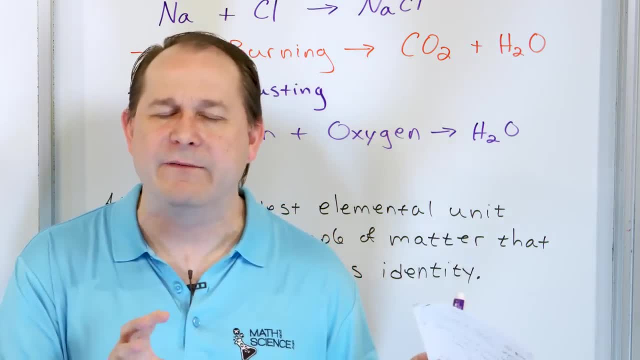 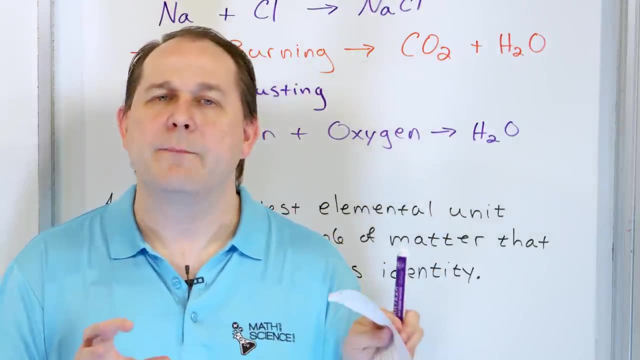 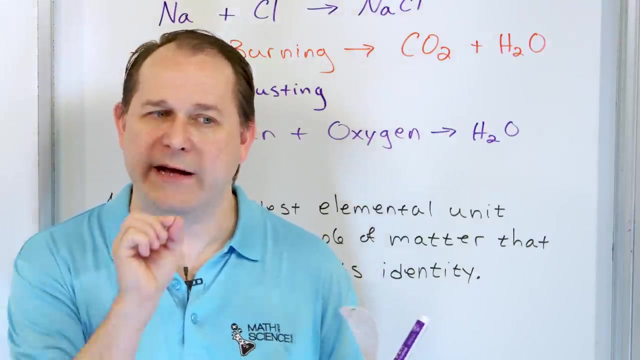 know exactly the details of exactly how things behave, how the chemical bonds work, how they break and how they form. yes, we have theories on how they somewhat work, but we also have situations we don't totally understand. how exactly do the bonds break and form exactly on a nanosecond, by? 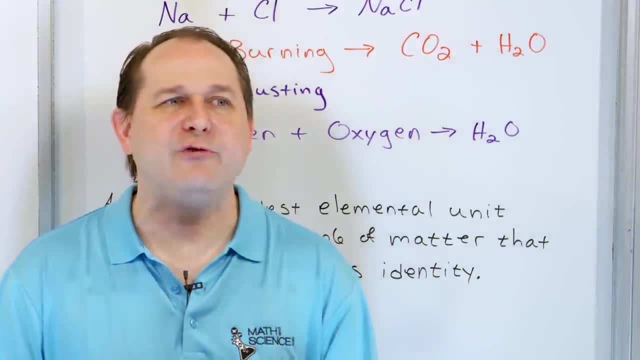 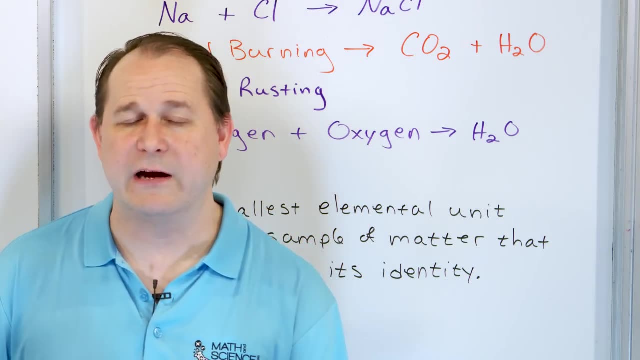 basis. those are areas of active research. how do we make chemical compounds of a certain shape, in a certain size to perform a certain function? those are things people are researching. so when you read this stuff and when you learn this stuff, and when you watch me talk and talk and talk, talk about it. 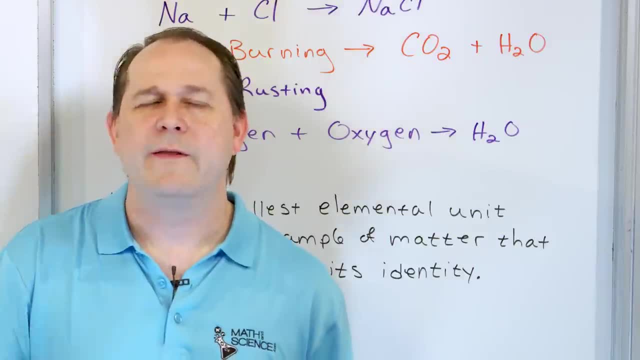 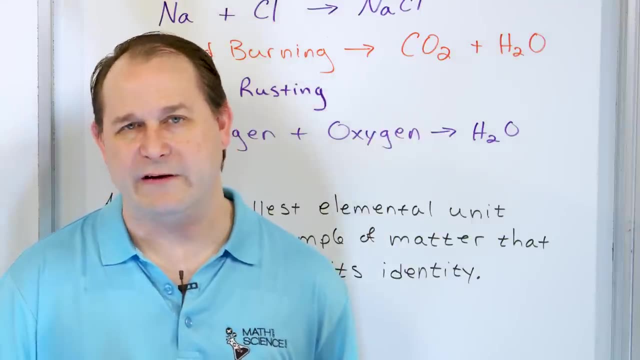 and it seems like we know everything in the back of your mind. i want you to know there's tons we don't know and there's tons of room for you to make that next discovery. that's what i want you to know because i want some people watching this to get excited and get pumped up and learn this stuff and 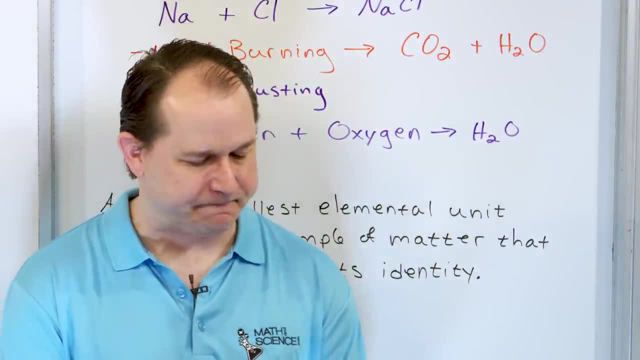 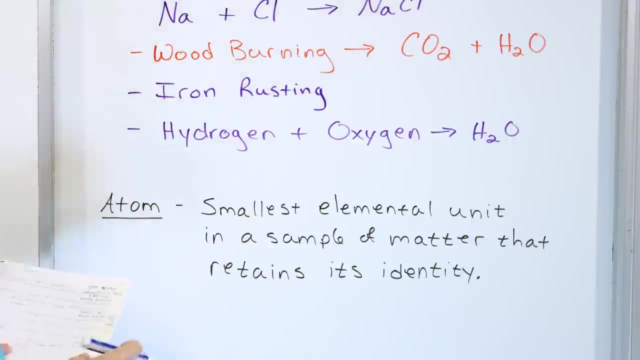 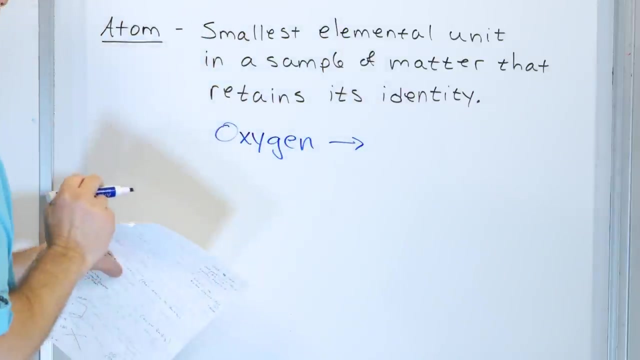 take the tools and then go discover the next big thing. all right, so we've talked about what is chemistry. we've talked about atoms- right. some examples of atoms- right, we've talked about a lot of these already. we know we have oxygen, right, oxygen is on the periodic table and we're going. 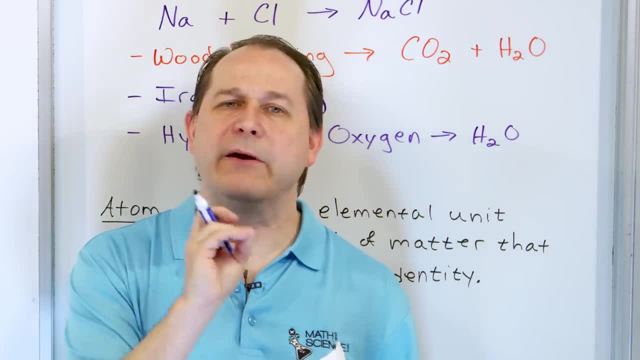 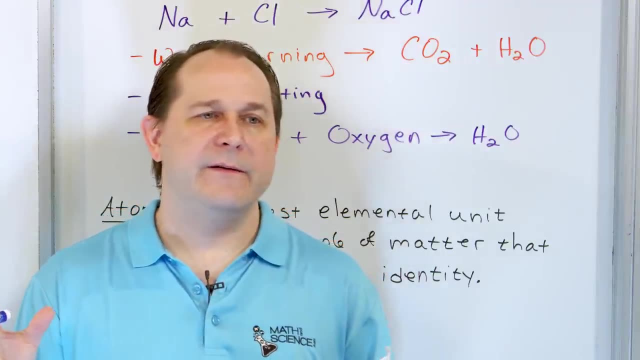 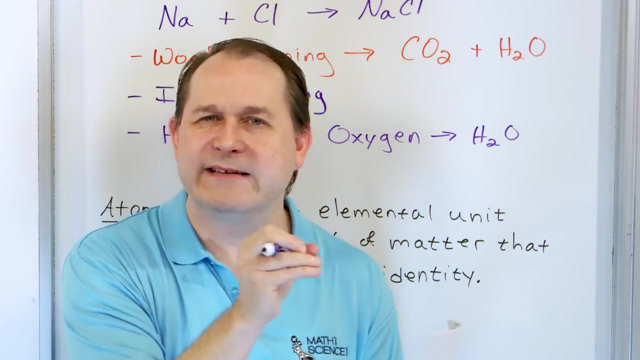 to talk about the periodic table a little bit better, but the period a little bit later. the periodic table is a organizational chart that shows all of the atoms that we know about and, uh, it goes in order of increasing what we call atomic number in the nucleus. so the nucleus contains: 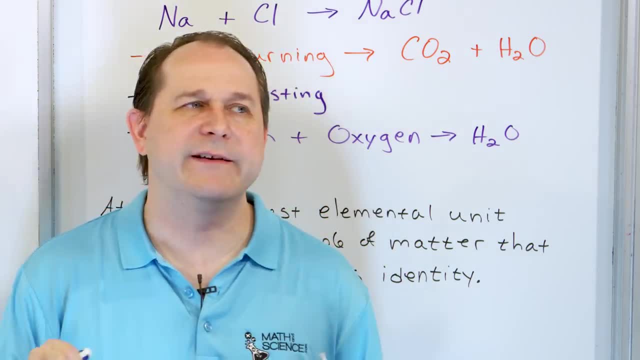 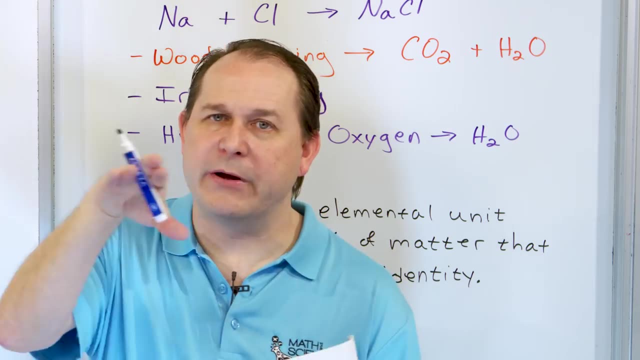 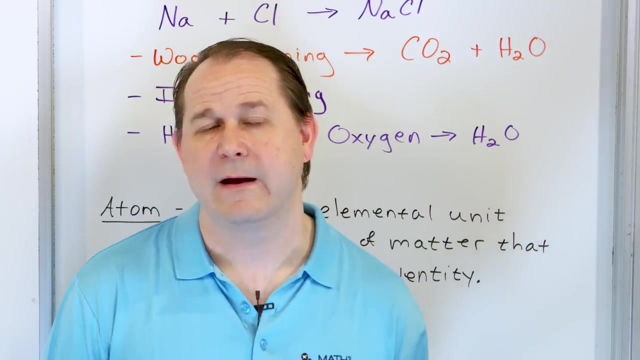 the protons and the neutrons. and as we add protons in the nucleus we get a different element. so hydrogen has one proton, helium has two protons. and you go up the periodic table. as you add protons to the nucleus you get heavier and heavier elements that are totally different characteristics. but 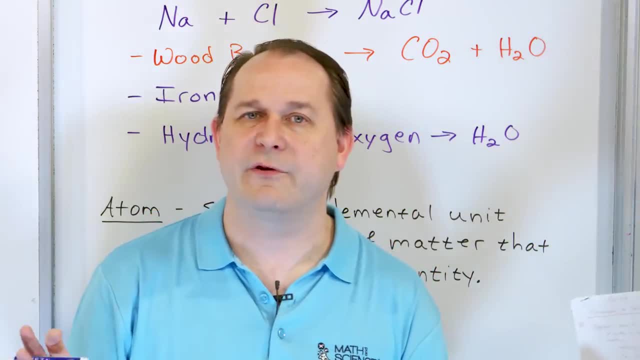 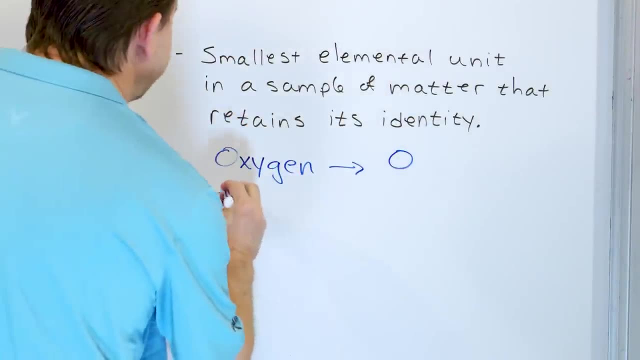 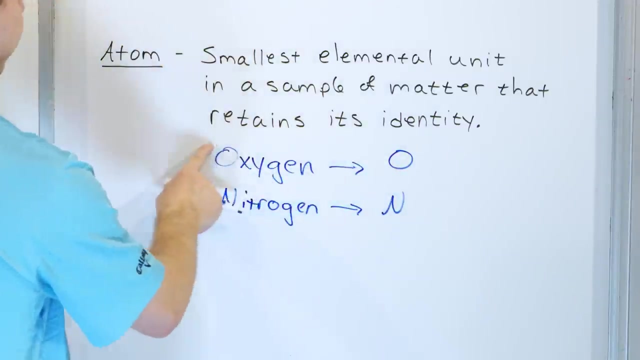 that table is structured in such a way that makes doing chemistry easier and we'll talk a lot more about that in a little bit. but we have oxygen. the chemical symbol of that is just the letter o. we have nitrogen, chemical symbol for this just n. so far it makes sense. right. o goes with o. 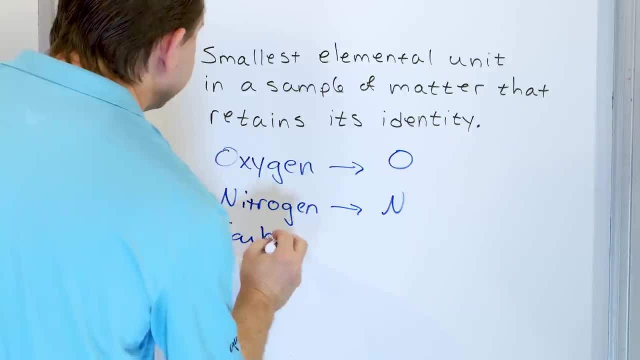 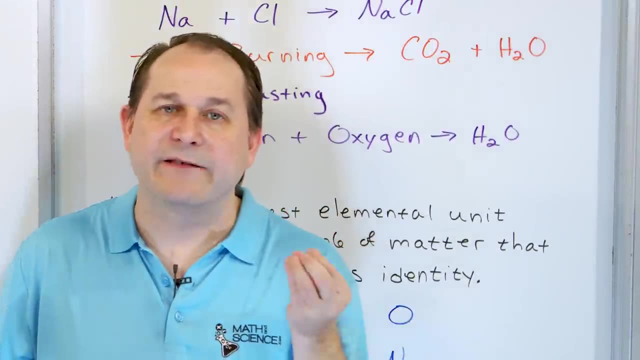 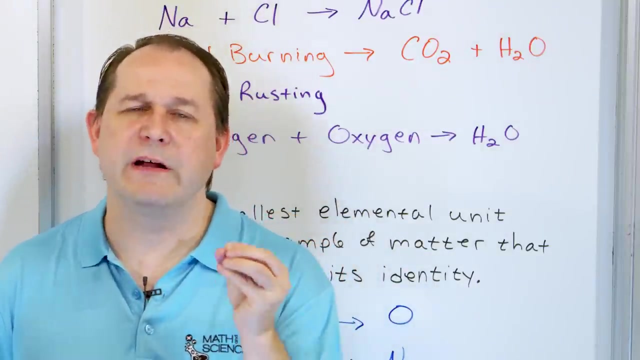 n goes with n. we have carbon, very important c in fact. i want to talk about carbon for a split second. you know, all life that we know about on this planet has carbon as a building block and we're going to learn a lot about that later. the reason life is built on carbon is because carbon 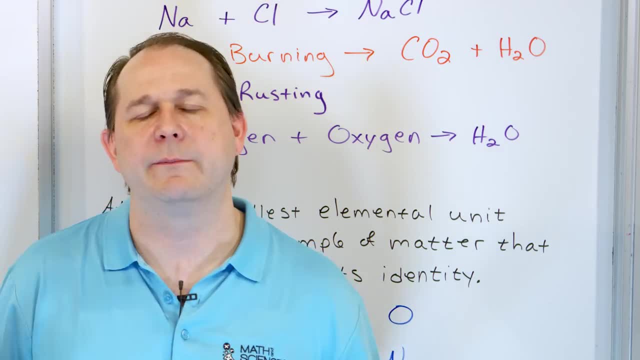 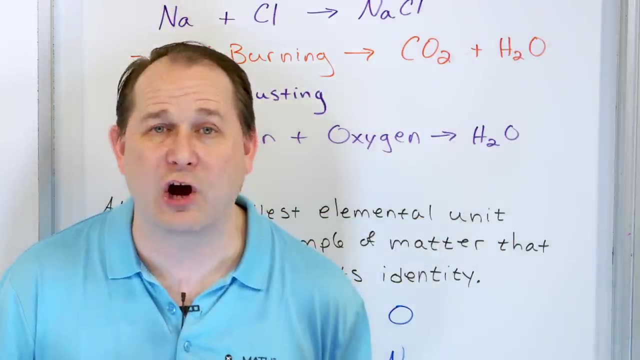 can bond to itself in ways that other elements can't. it can basically form four bonds at once, and that allows you to make very long, complex chains of carbon and other elements can also bond in chains, but not quite as good as carbon can. there's other characteristics of carbon that make 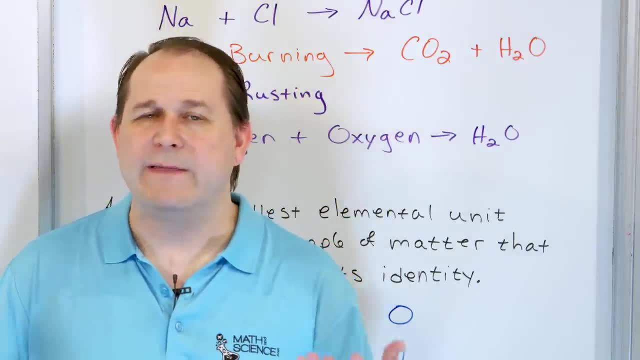 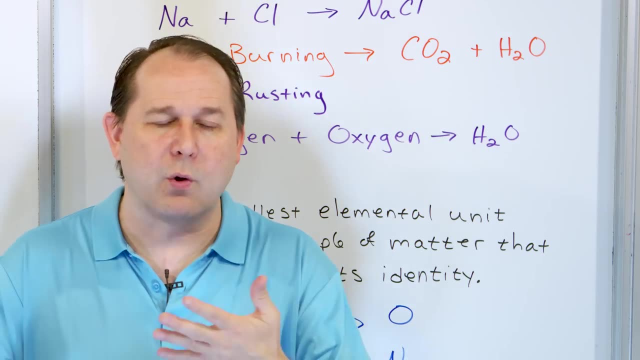 it where life is, it favors it, but that's the big one that carbon can bond in ways other elements can't, and it can make longer chains. now the dna molecule in your body, of course, is a carbon chain with all other things on the other side of your body, and that's what we're going to talk about next. 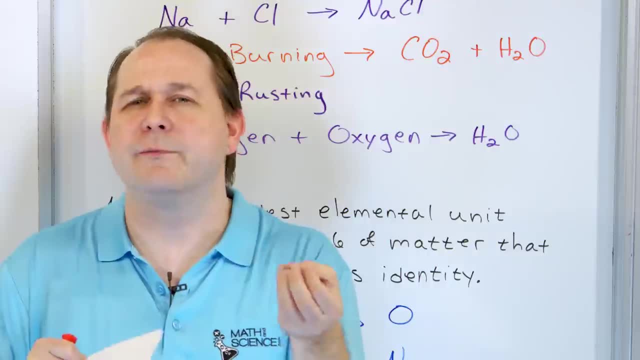 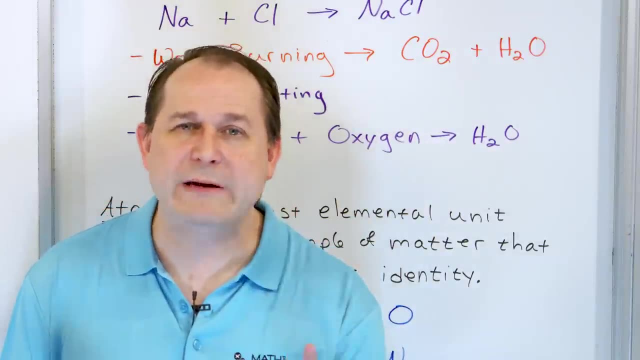 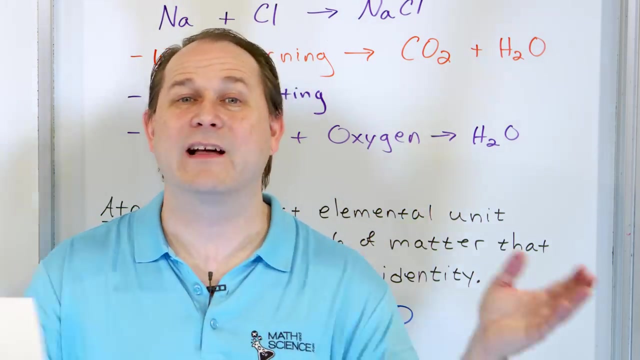 but if carbon couldn't bond the way it could, then we couldn't have long chains of atoms and you wouldn't have dna and then you wouldn't have life. so carbon is extremely important. in fact it's so important that after you finish chemistry 1 and chemistry 2, we have an entire class, in fact two. 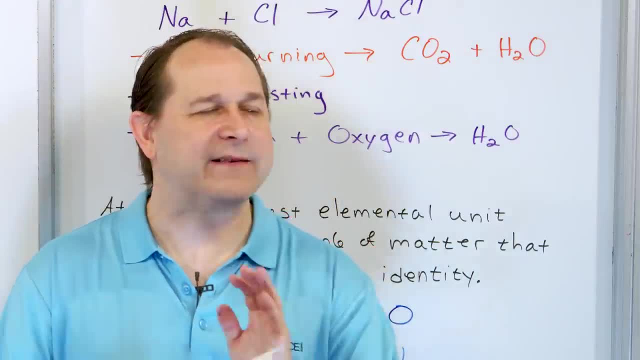 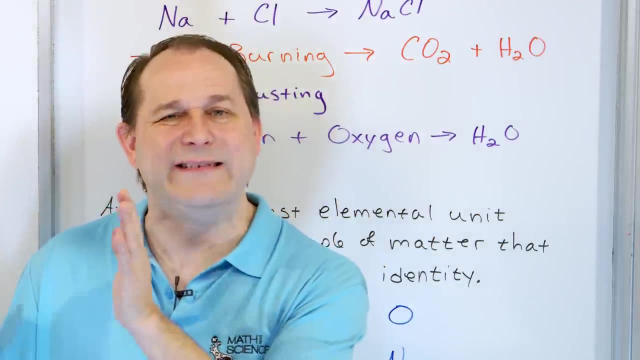 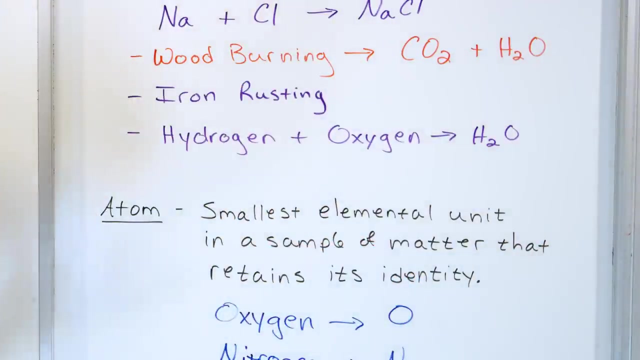 or three classes. that's called organic chemistry. that's only talking about the chemistry of carbon, carbon atoms, carbon molecules. so we have an entire set of learning dedicated to learning about how carbon works, because it's so important for everyday, you know, earth, and for life. uh, as we 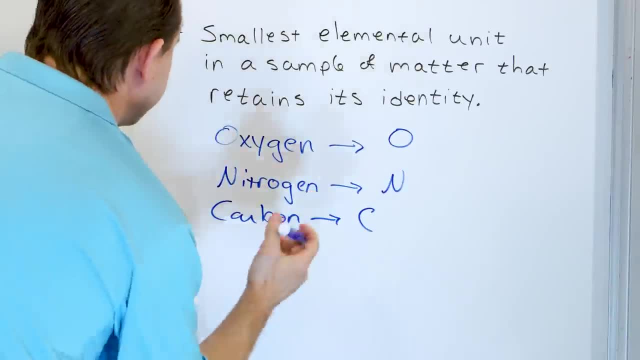 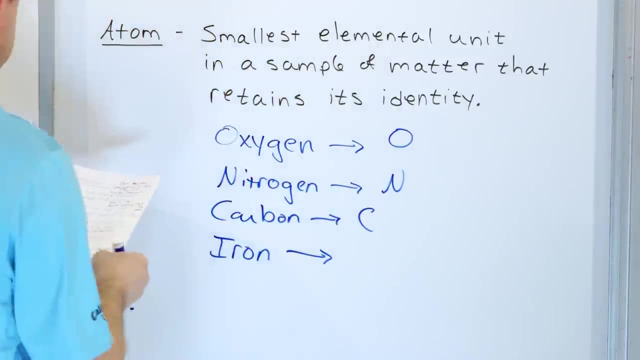 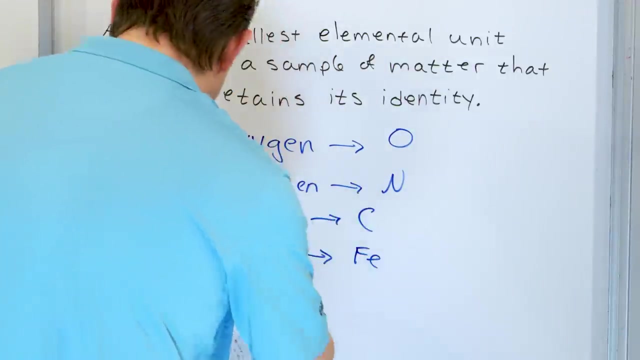 know it, and so on. right now i do want to talk about another one here: iron. now, the chemical symbol for iron you would think would be f? uh, uh, uh here, but actually, or you would think it would be i, sorry, you would think it'd be i, i for iron, but actually it's f? e. now, some of these most 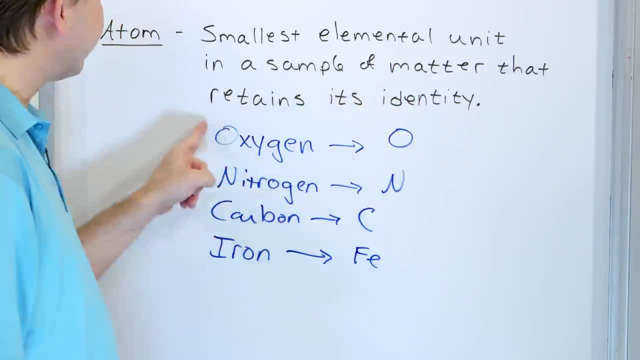 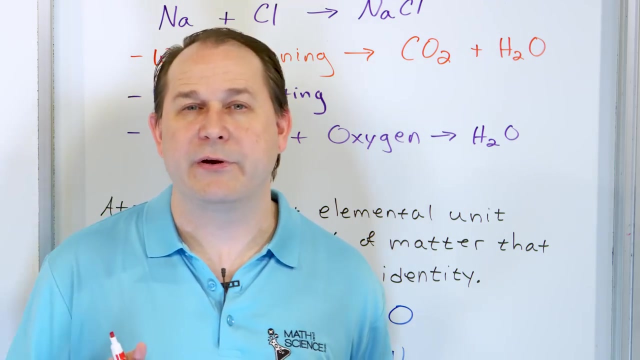 of the elements on the periodic table. we just picked the first letter or the first couple of words to represent them. but sometimes the elements are totally different than the first letter and that's because when they first started doing this stuff they all worked in latin. the scientists worked in latin, so a lot of the the symbols in the periodic table come from the latin. 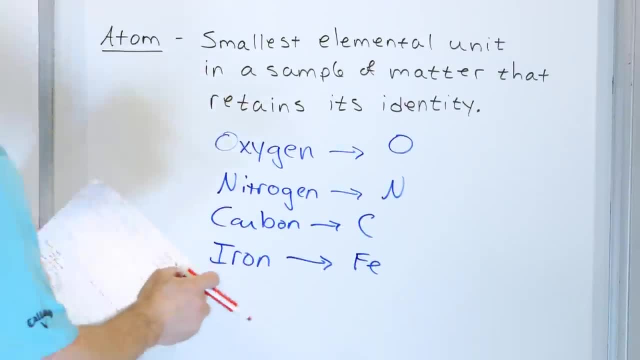 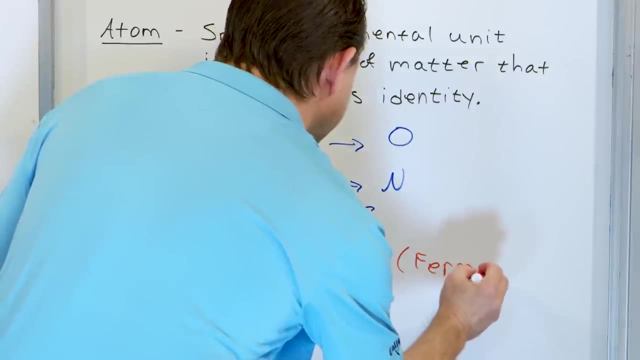 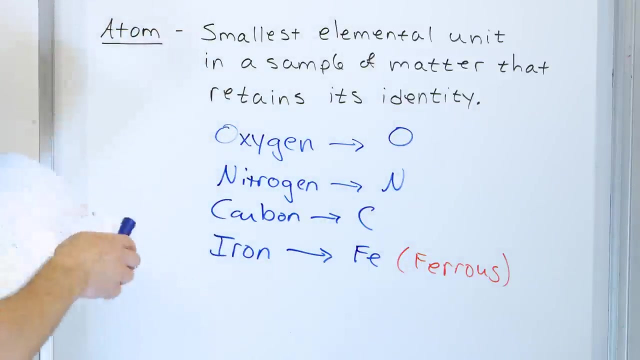 version of that material. so, for instance, iron, uh, f, e comes from the latin, which is ferrous. now i'm not going to ask you or tell you to memorize. you know these latin, letting you know sometimes some of these off the periodic table. they look a little bit weird. 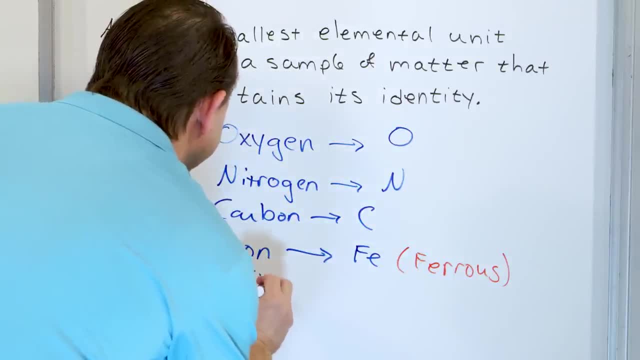 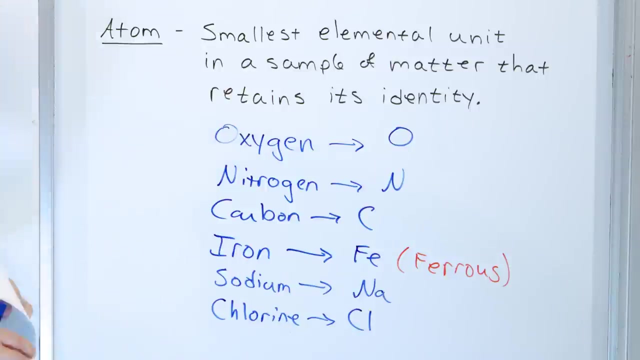 another one would be sodium. you think sodium would be s or so, but actually sodium is na. and you have chlorine. you think chlorine would be ch. it's actually cl, right? so basically, the elements on the periodic table are going to be represented by a symbol, either a single. 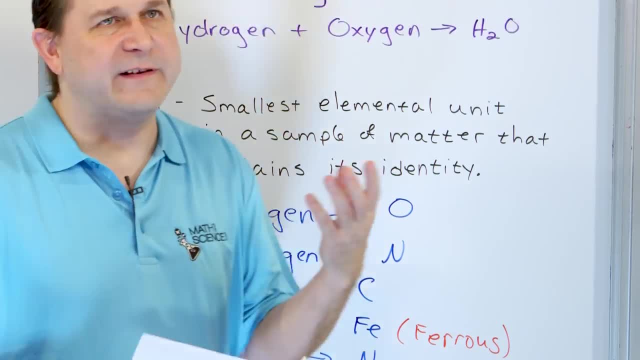 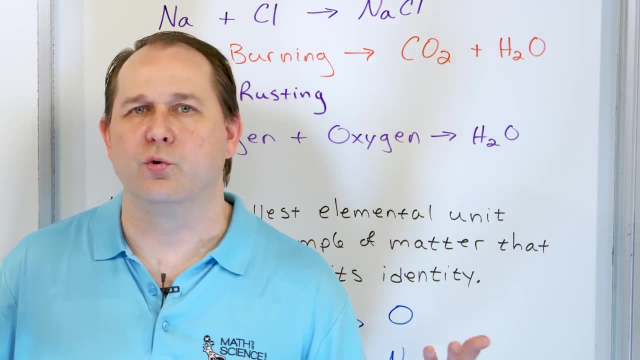 letter or two letters, and sometimes the two letters are correspond to the word, and sometimes the two letters come from latin. so you're just going to have to, eventually, through working with it, you'll you'll remember the ones that are that don't exactly match the word that they come from. 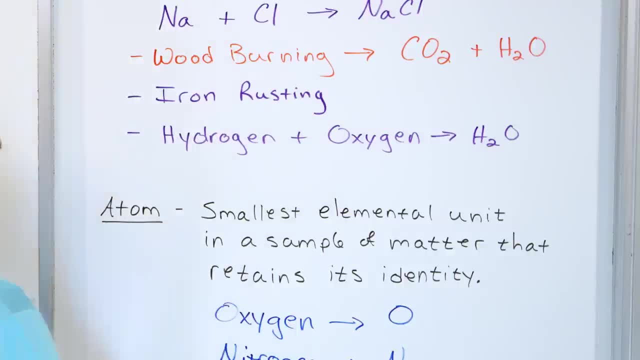 all right. so we talked about atoms, smallest elemental unit in a sample of matter that retains its identity. because if you try to split the atom up, then you're into the things inside, you're breaking it apart into the protons and the neutrons and all protons. look the. 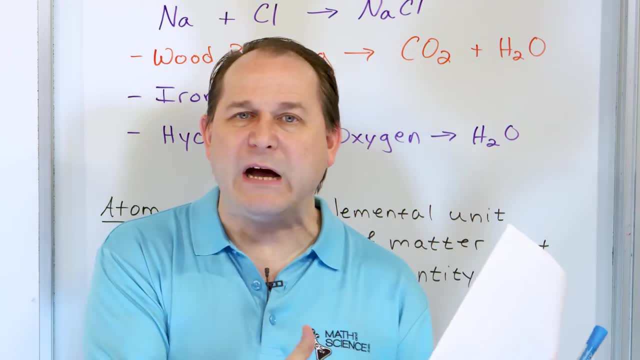 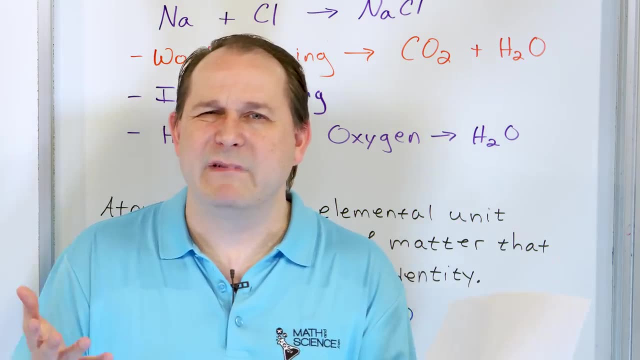 same and you're breaking it apart into the protons and the neutrons. and all protons look same, All neutrons look the same. If you had a bucket of electrons, if you could just put a bucket of electrons here, they would all look the same. They don't have any difference. 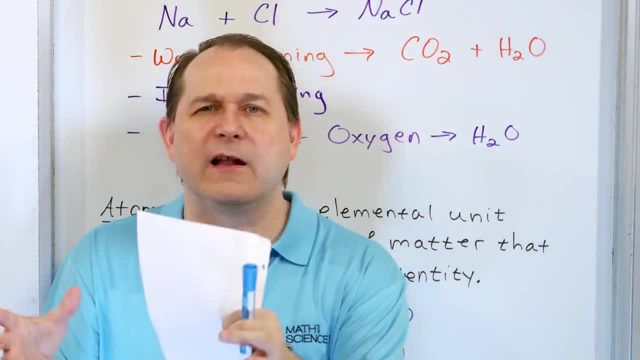 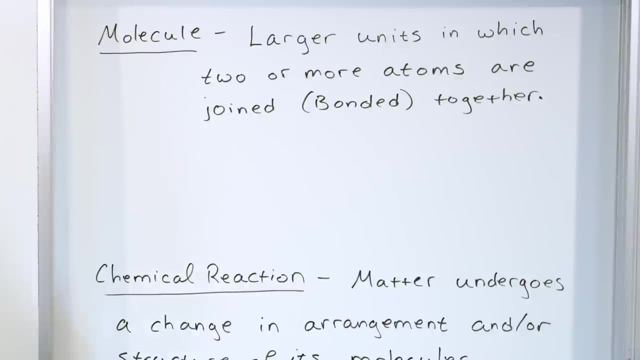 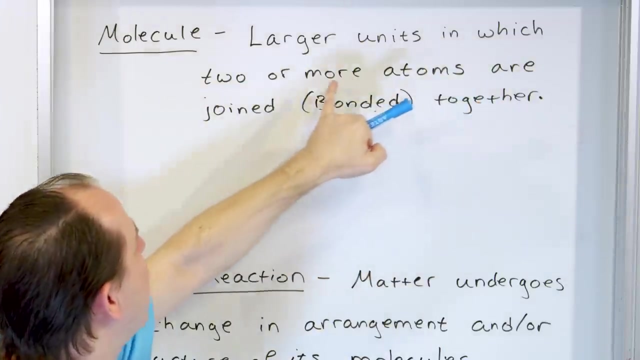 in the character there. Only when they're combined in these ways, these different elements have different characters. Now, the next thing we're going to talk about is the concept of a molecule. A molecule is a larger unit in which two or more atoms are joined, which we call in chemistry, bonded together. 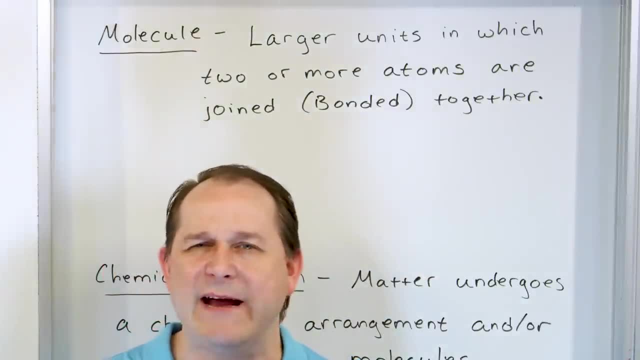 So I know that you all have an idea of what a molecule is. It's kind of, in everyday language, This or that molecule. I know that you have an idea of it because we've all heard it before you take a chemistry class. But we have to make sure we are on the same definition And 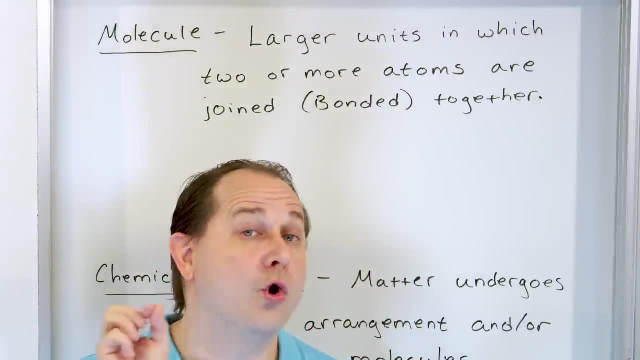 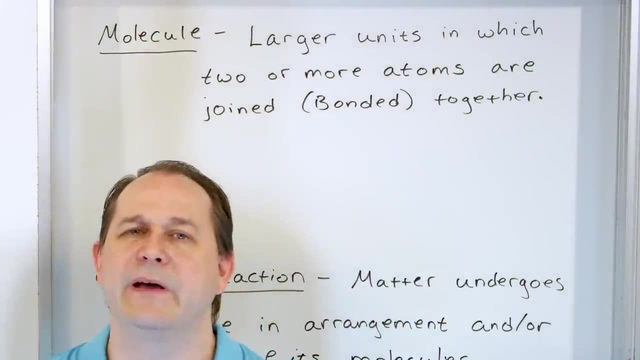 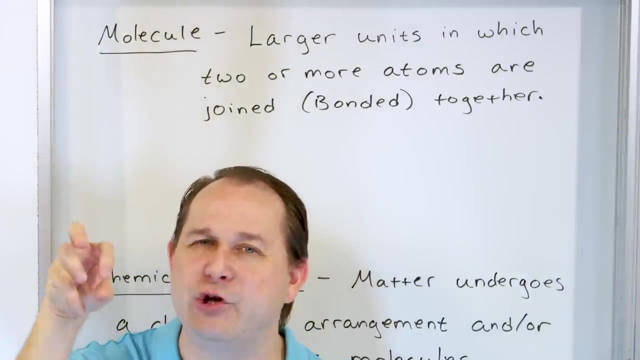 in our definition, a molecule is when you take two or more atoms and you join them together into their own little unit where they float around together. They're kind of hooked together because these things do in some cases like to bond together, like H2O water. They're bonded together in a unit and that unit is called a molecule. 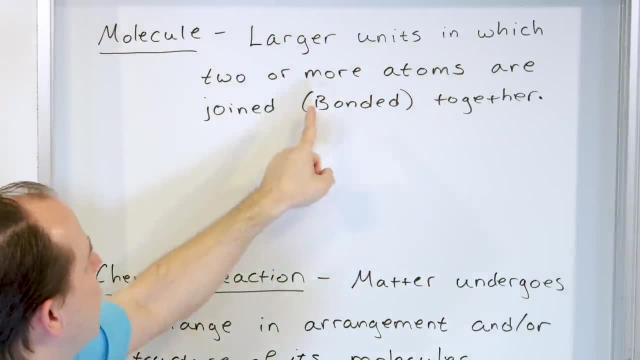 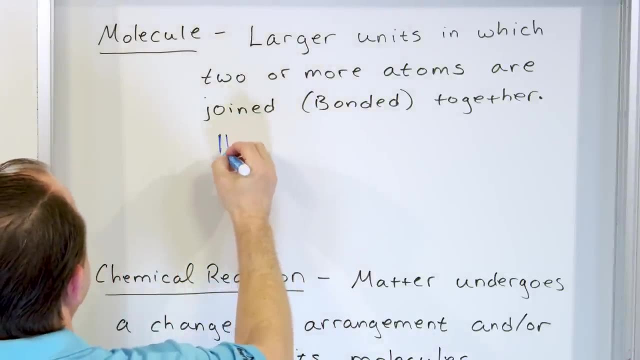 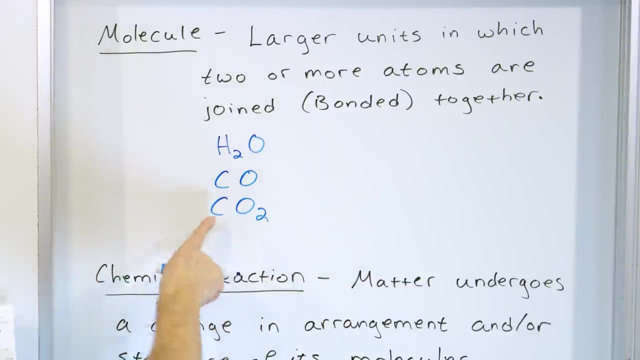 So it's a larger unit in which two or more atoms are joined, which in chemistry we call bonded together. So the most famous of this, of course, is H2O: Two atoms of hydrogen and one atom of oxygen. Other examples: Carbon monoxide, carbon dioxide, CO2.. So one atom of carbon, two atoms of oxygen joined. 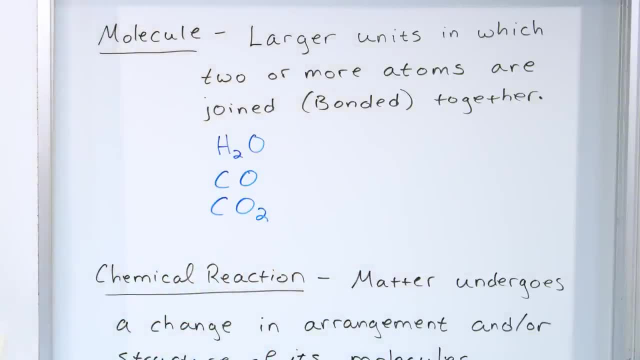 together as a unit which can free float around by itself, which we call a molecule. Now, molecules do not have to be different elements like this. Actually, we can have sometimes the same molecule bonded to itself. For example, if you take two atoms of oxygen, 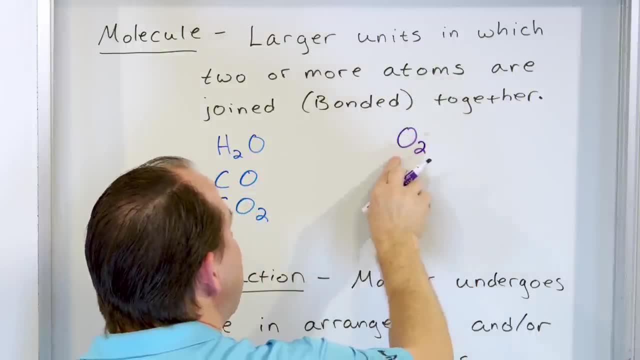 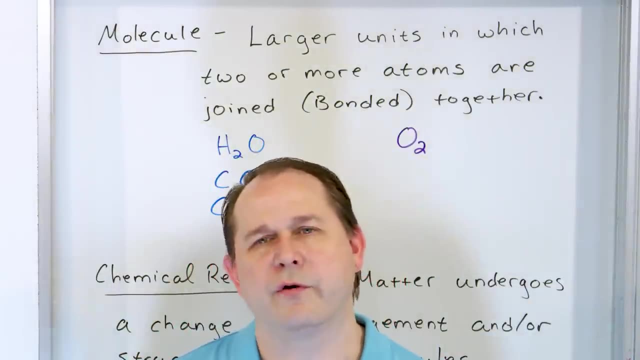 and bring them together, They actually form a molecule called O2, oxygen gas. right, You may have heard in the movies: in the hospital they'll say: turn on the O2.. The patient needs O2.. Or sometimes if you watch NASA and rocket launches, they'll say: you know the O2, we're 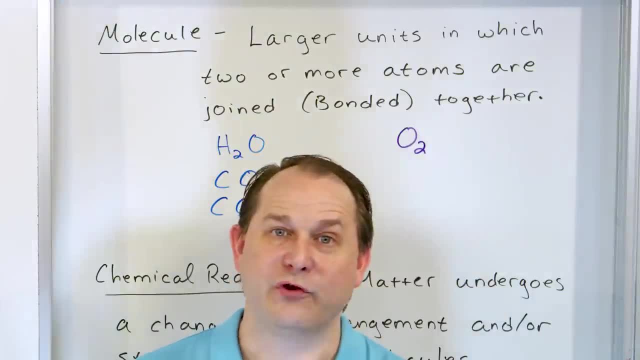 ready to go with the O2 for launching the rocket, because the O2 is part of the rocket fuels, It's actually what we call the oxidizer. But in any case it's part of what goes into the engine to burn to make the rocket fuel. It turns out that atoms of oxygen really don't. 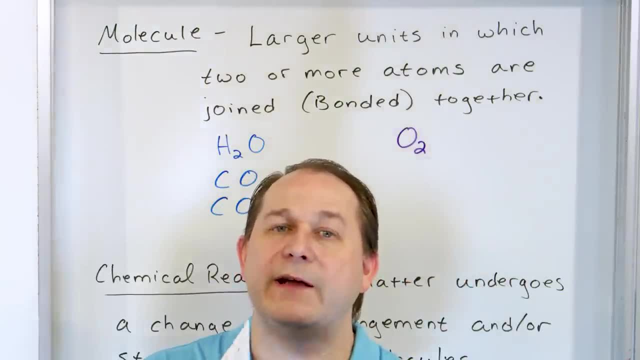 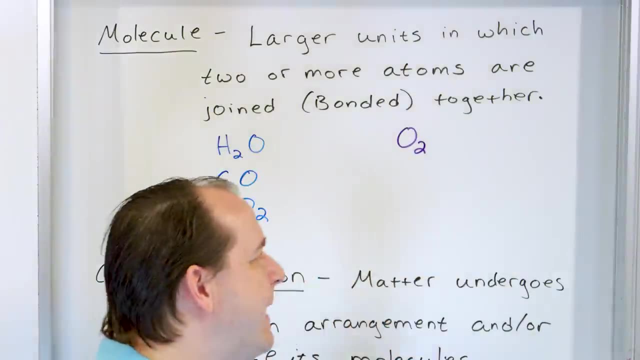 like to stay separated. They actually join up together and they form a molecule. They bond together in pairs And that's why we have O2.. So if you've ever heard of O2 gas, that is what that means, because they are not usually separated, they're bonded together. 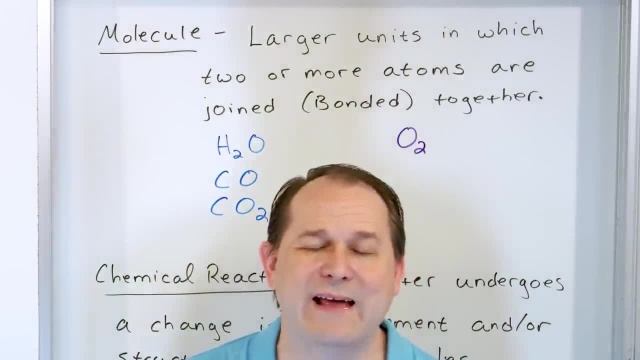 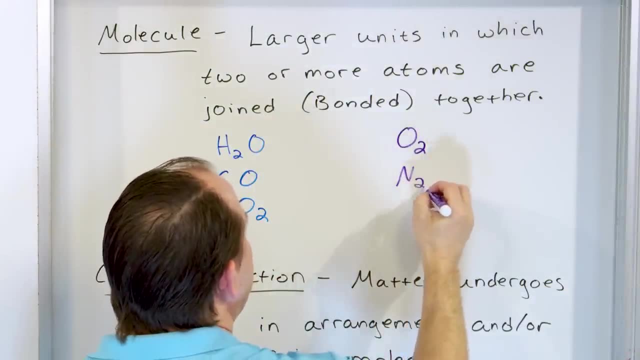 And we're going to learn exactly why oxygen likes to do that later. Not all atoms do it, but some do. This, of course, is a molecule. You can also have nitrogen, which also likes to bond with itself- N2.. 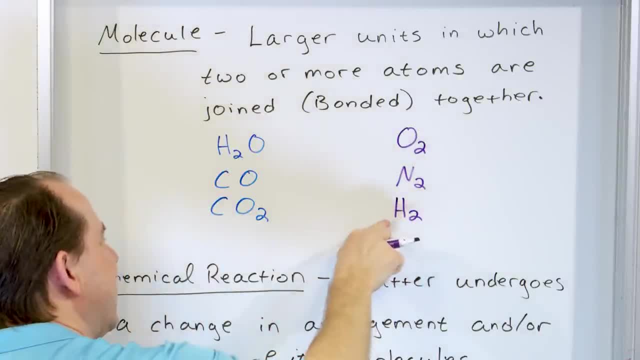 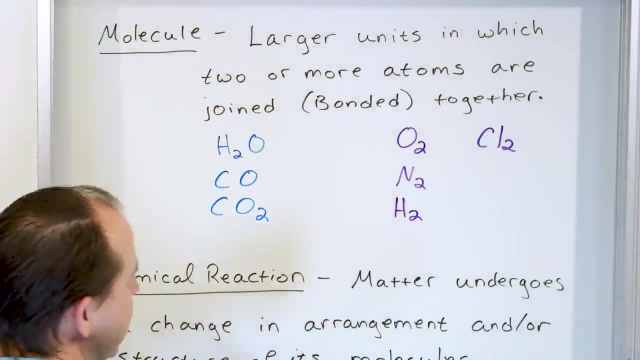 Hydrogen, Hydrogen. Hydrogen, Hydrogen to bond with itself. So it actually forms a molecule of two hydrogen atoms which are clumped together, bonded together. Chlorine is another example. Chlorine likes to bond to itself as well. 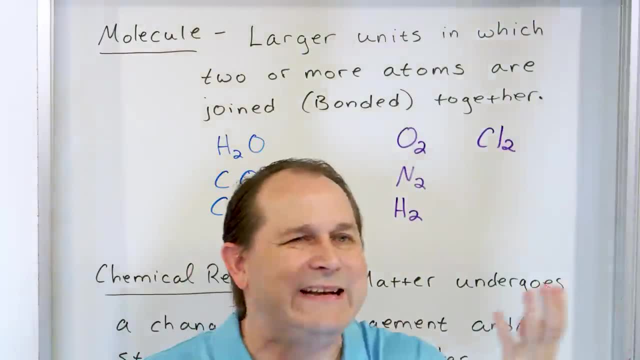 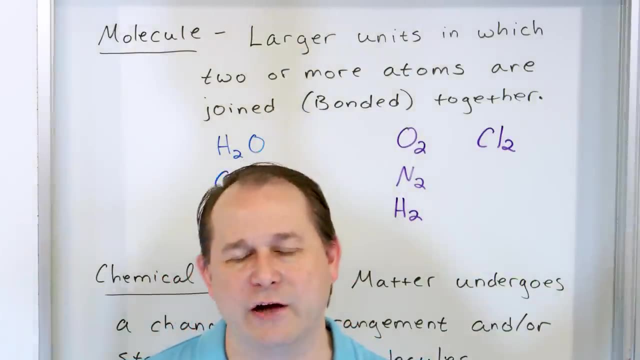 So these are all molecules? right, They're all molecules because a molecule is any time two atoms really come together and hook together like this and bond together. The whole concept of bonding we need to have a whole lesson on, because that's a whole bag of worms we've got to talk. 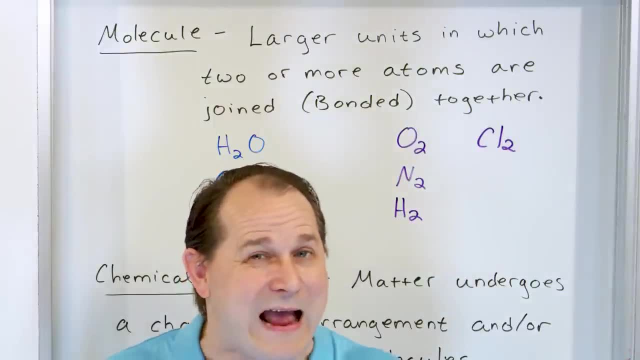 about. There's a lot to understand about bonding. We don't even totally understand exactly how bonding works. right now, If a chemist tells you, oh yeah, I know how bonding works, they're lying to you because really we have our theories. It goes into quantum mechanics, right? Quantum. 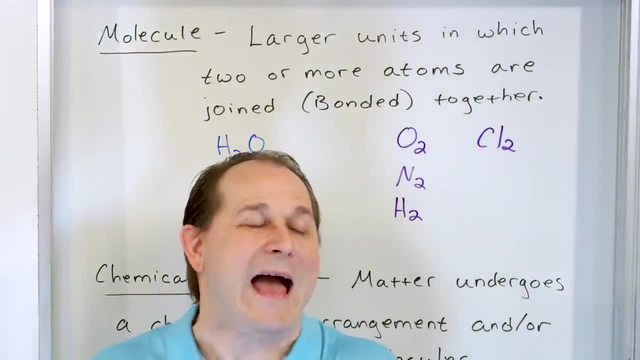 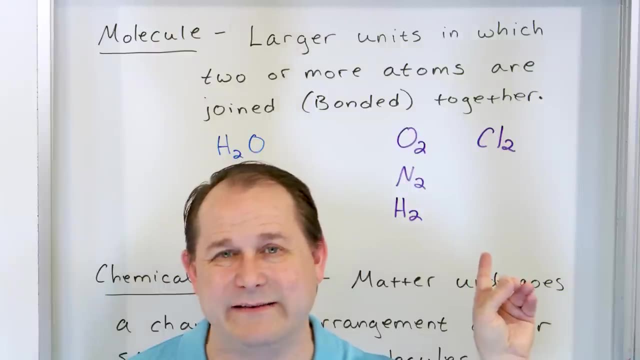 chemistry And we have equations that predict bonding, but the actual details of exactly how it happens. we don't understand all of those details, especially for more complicated molecules than these. That's why I'm saying there's always opportunities for someone else to make the next. 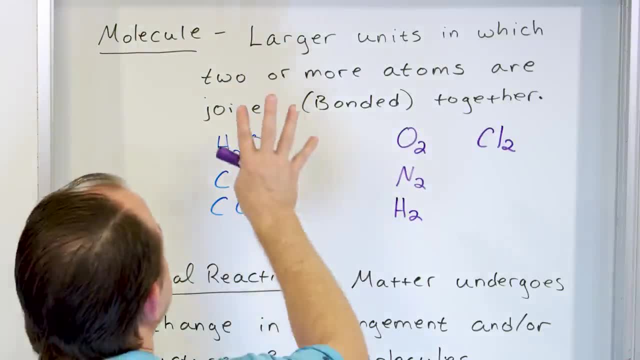 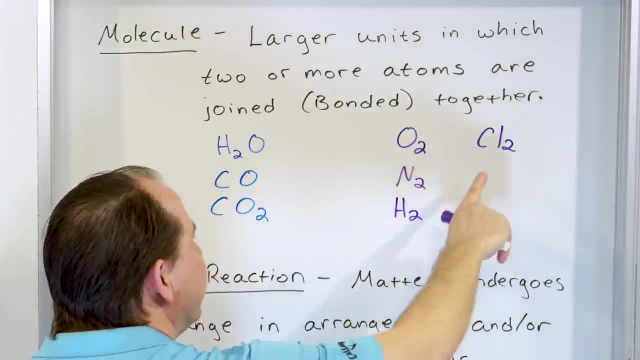 big discovery. All right, So we have molecules. These are when multiple atoms join together And we can have the same atom bond to itself. These are still molecules. We can have different atoms come together And these are just very simple molecules. 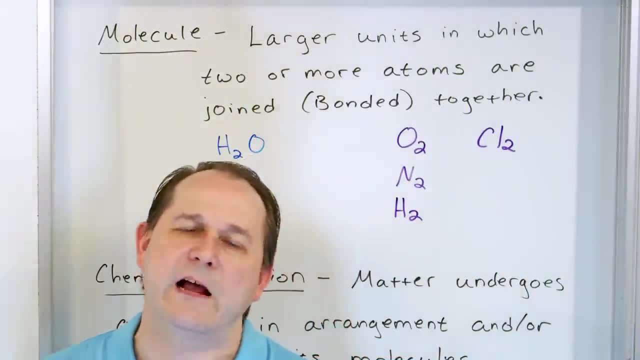 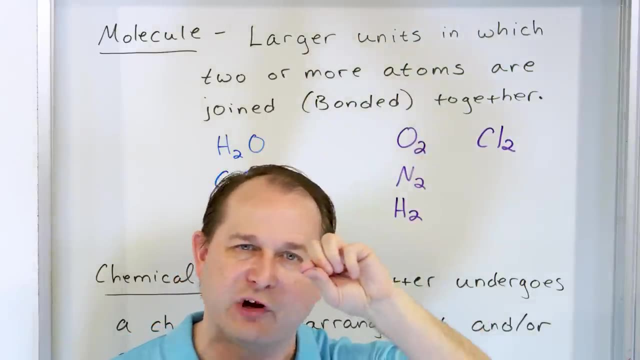 but we can have molecules with five or ten different atoms. We can actually even have molecules form a chain or even a ring. We can actually form a circle. I told you, carbon can bond in very neat ways. Carbon can actually take and bond itself into a circle Different size. 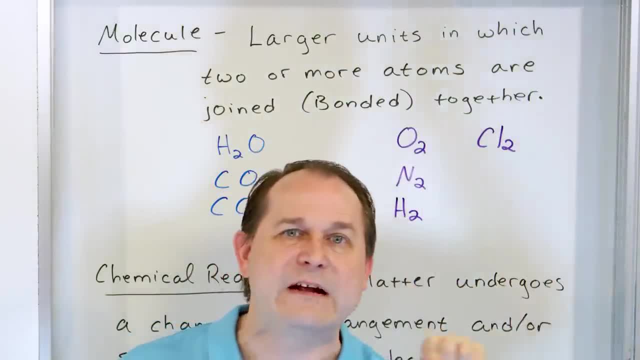 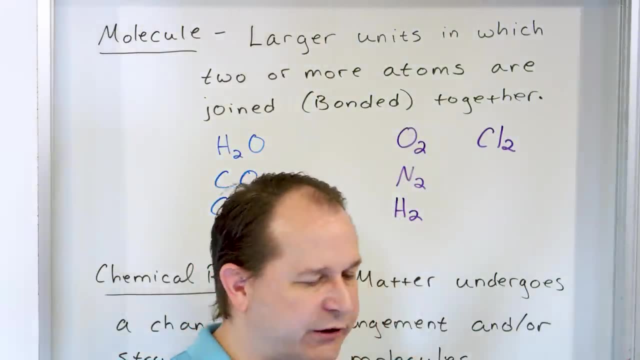 circles, Small circles with five or six Atoms in ten or twenty circles. We're going to talk a lot about that later, especially if you take an organic chemistry class. So that is what a molecule is And I think I want to talk just as an. 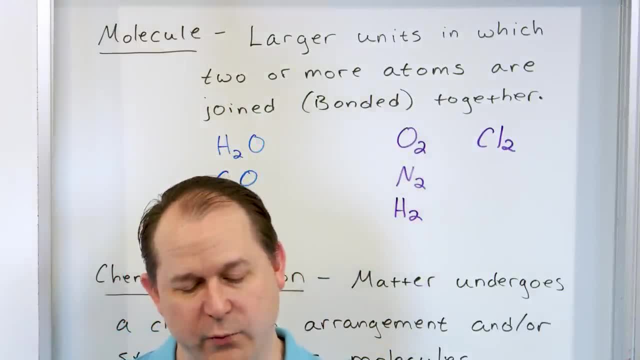 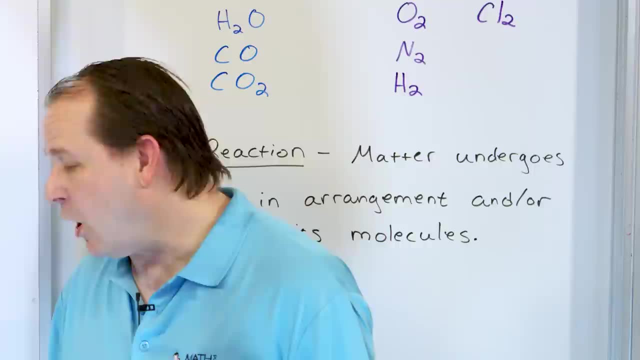 aside for a second before I jump into the next part of this, because after we talk about molecules, I want to talk about chemical reactions. right, And chemical reactions are really what all of chemistry is actually about. But before we get into this, I want to impress upon you something. 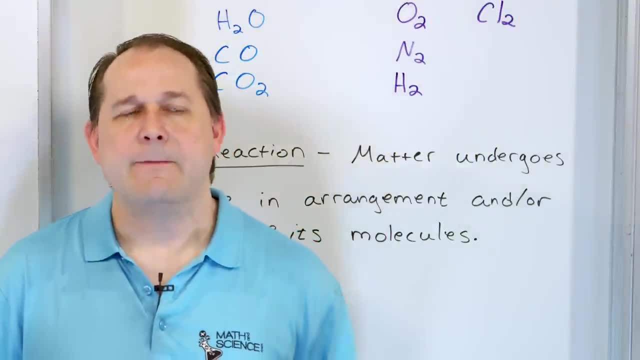 that I really wish someone had told me, And that's what I'm going to talk about today. I'm going to talk about what's going to make chemistry understandable when I learn chemistry, Because it's really the number one thing that's going to make chemistry understandable for you, right as. 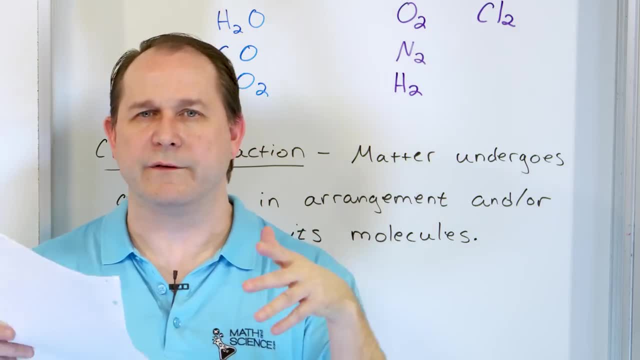 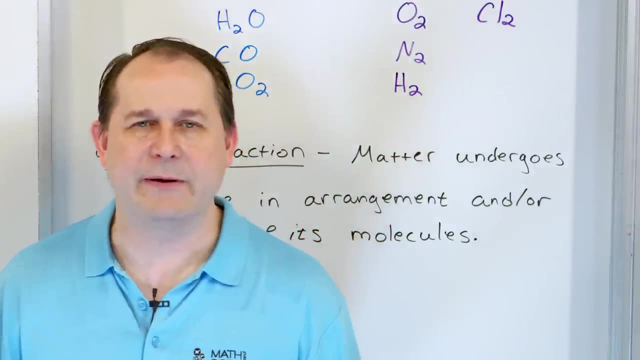 you get past the surface layer, Most people can understand atoms and molecules, But when you get into reactions you start trying to understand why they're happening and why they're not happening. Why should the reaction happen? Or maybe sometimes the reaction doesn't happen And 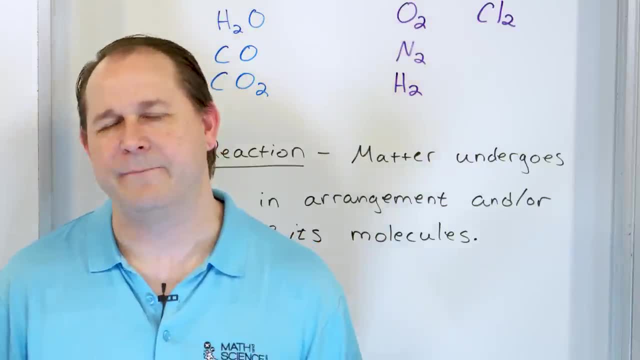 you start to kind of wonder why sometimes it happens and sometimes it doesn't happen. Well, let me tell you the punchline to this. right now I can't give you all the answers, but I can give you a big piece of the puzzle. So let's get started. 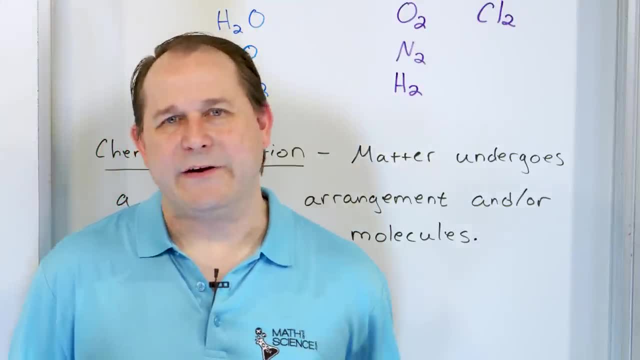 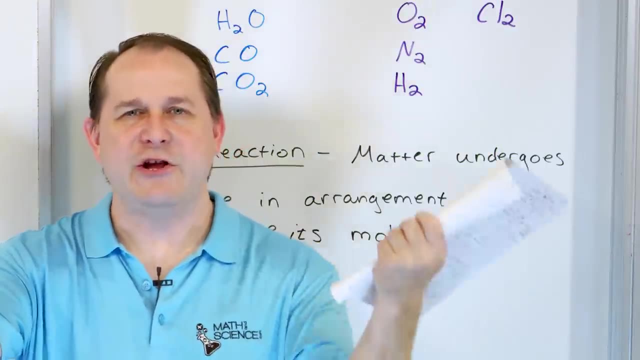 puzzle and I can give it to you right now, in lesson number one. All right, here it is. So you know that you have protons which are positive, right, And you have electrons which are negative, And you know that opposites attract. So by now you should have learned that protons and electrons 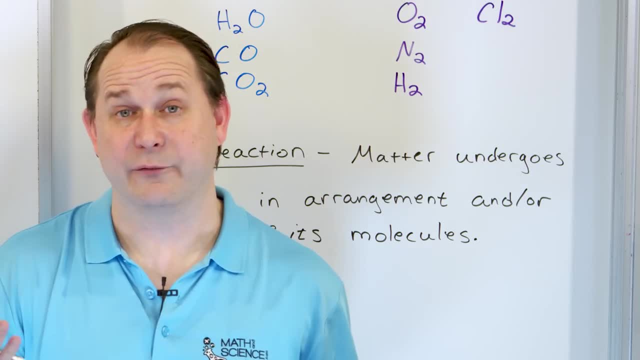 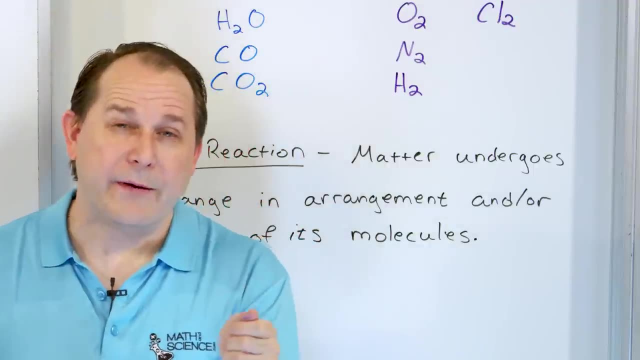 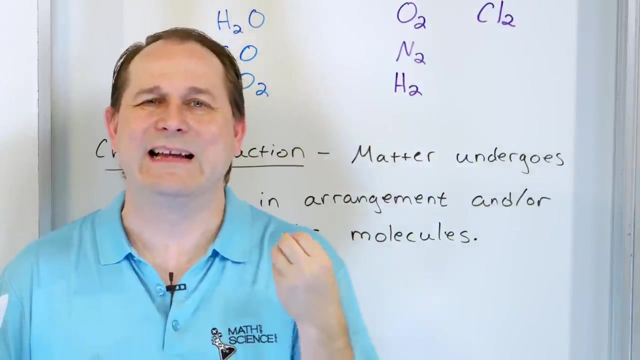 attract each other And, like signs, repel. So two electrons push apart and two protons also push apart. All right, I hope that I'm going to blow your mind in a second when I tell you that this force of attraction between protons and electrons, we call it the electrostatic force, Electro 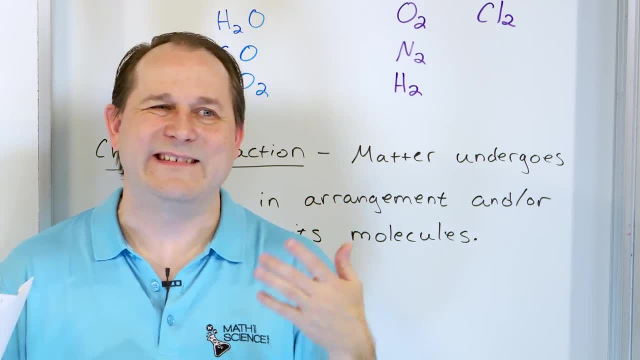 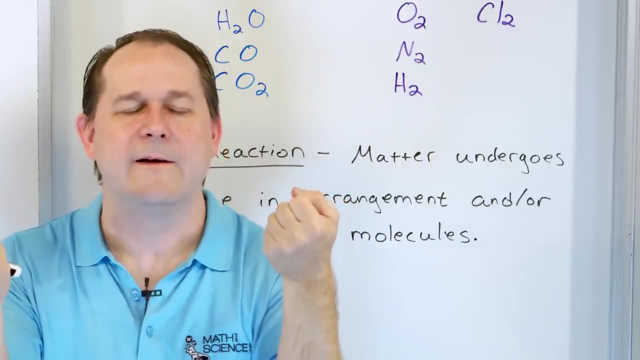 because it's related to electricity, because of charges, Static because there's no current flowing, but it's called electrostatic. So they're just sitting there and nothing's really happening, but they're attracting each other right? So that big word electrostatic, don't let it scare you. 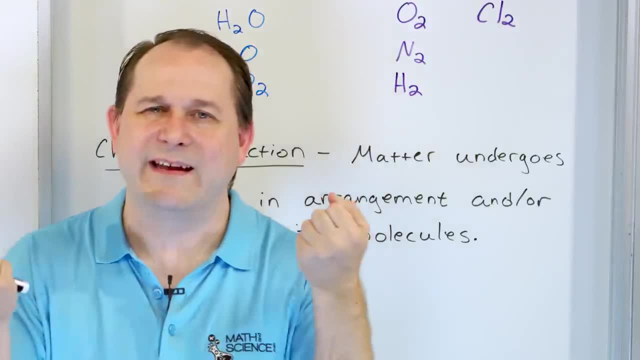 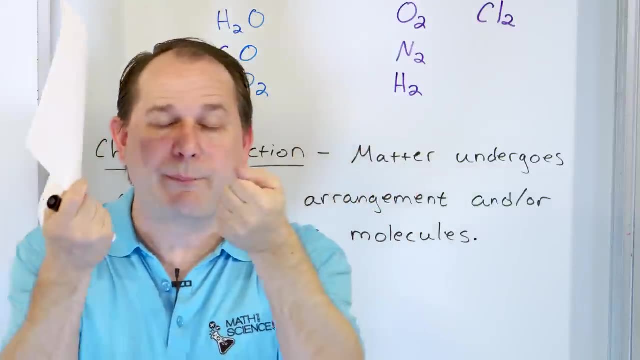 It just means electric force, right? The electric force that exists between two charged particles, like two protons or two electrons, or a proton and an electron, or a repulsive force between two electrons, or a repulsive force between two electrons or a repulsive force between two electrons. 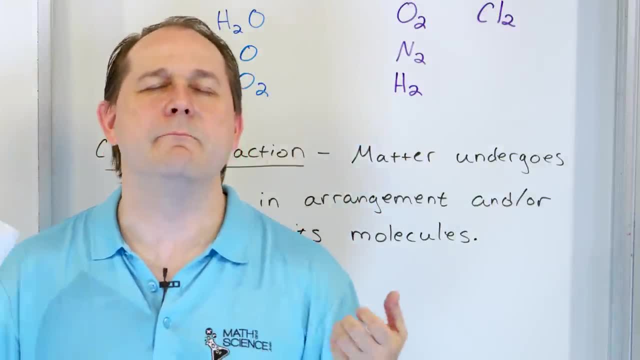 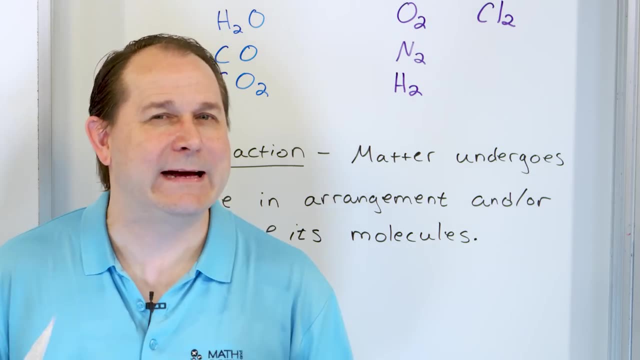 that kind of thing. The electric force is millions of times stronger than the gravitational force holding me to the ground right now. I'm going to say that again because it isn't something that makes sense and you need to absorb it because it really does govern all of chemistry, All of 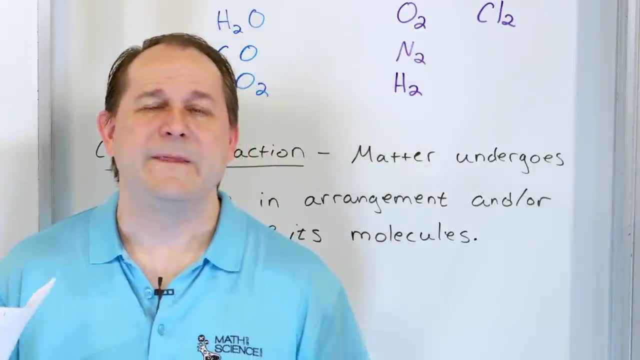 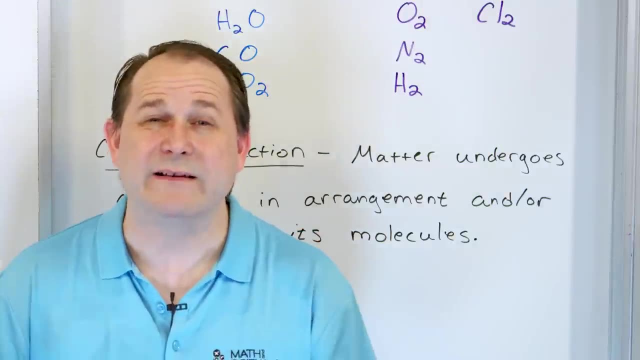 chemistry- And I do mean it governs all of chemistry: The electric force, the force between an electron and a proton, the attractive force that happens there. right, It's millions and millions and millions of times stronger than the electron, And that's because it's a force that 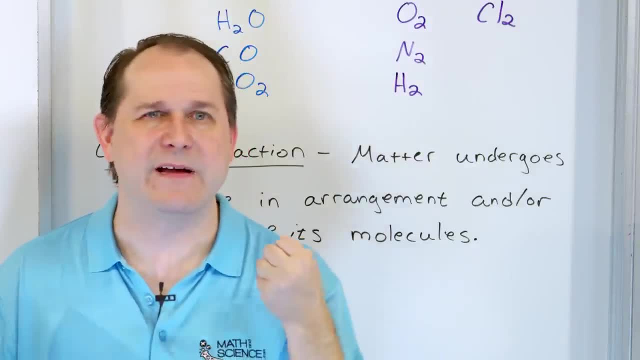 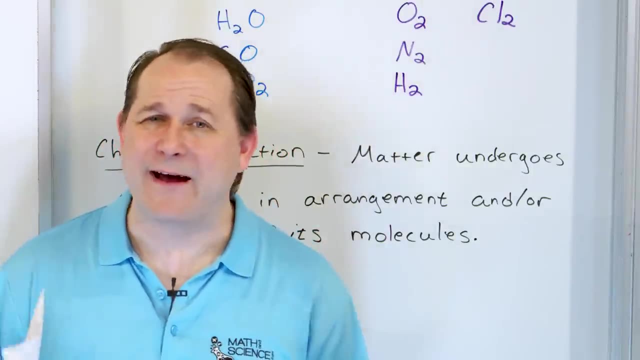 is stronger than gravity. It is way stronger than we think of in our everyday life. And because it is so incredibly strong, then that is what is driving pretty much everything in chemistry, right, When you mix two things together, sometimes they don't react, And sometimes 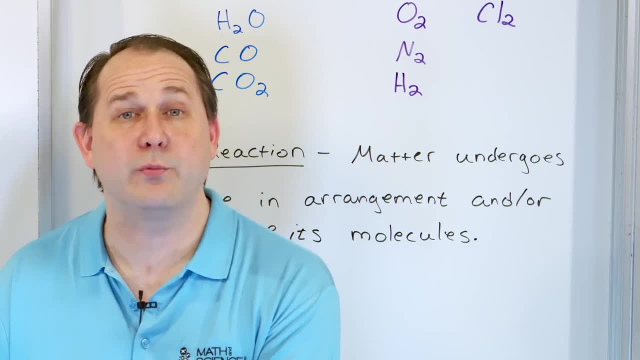 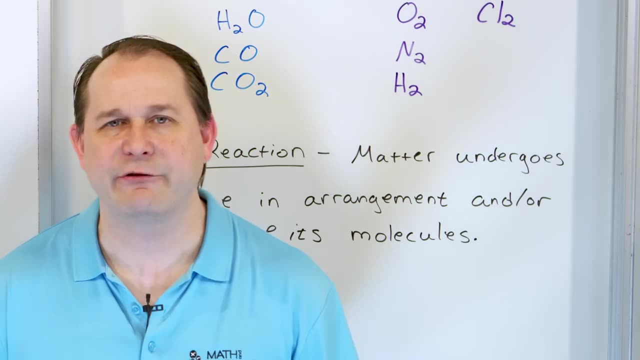 in a different situation, different set of things you mix together. they do react to form something new. But what governs, what determines if the thing reacts or if it doesn't? It's the electric force. If the situation that you put those things together, if the situation that you put those, 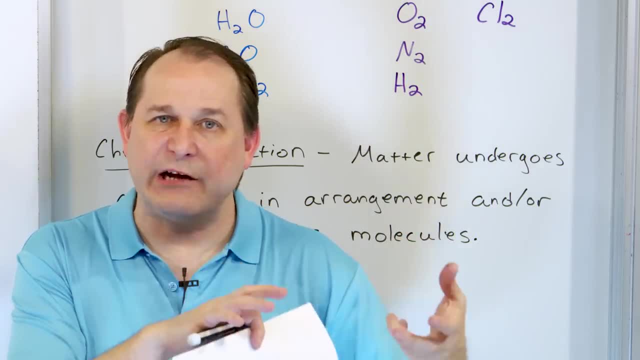 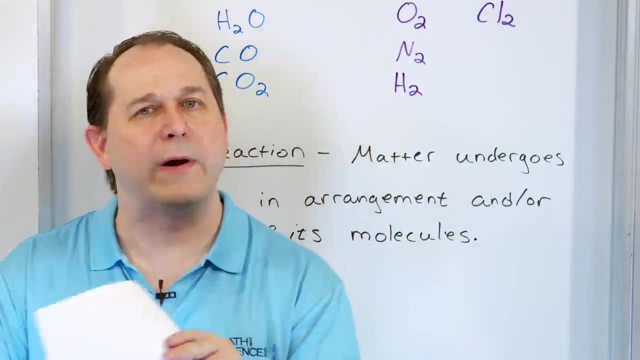 atoms in are in such a way that the electric force is strong enough, then it's going to rearrange what's going on and it's going to come together and everything's going to stick together in a way to rearrange, to form the products right, Because the electric force is what's governing all of the 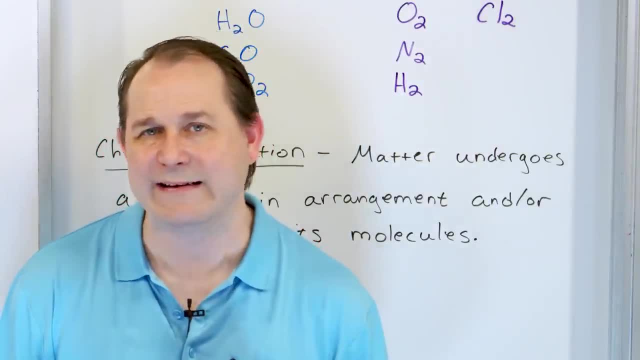 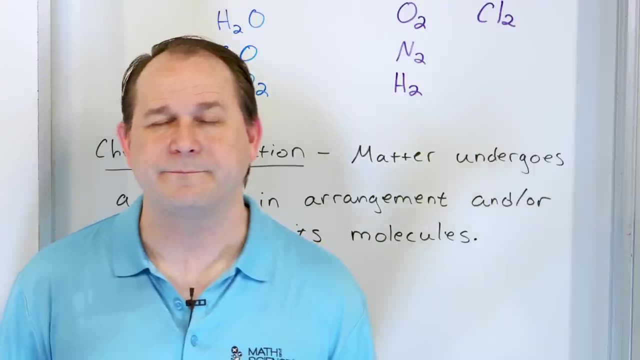 chemistry- that's happening. the electric or the chemical reaction, that's happening, right. But if you mix two things together and nothing chemically occurs, there's plenty of things you mix together and nothing will happen at all, right. Well, why doesn't anything happen? Well, 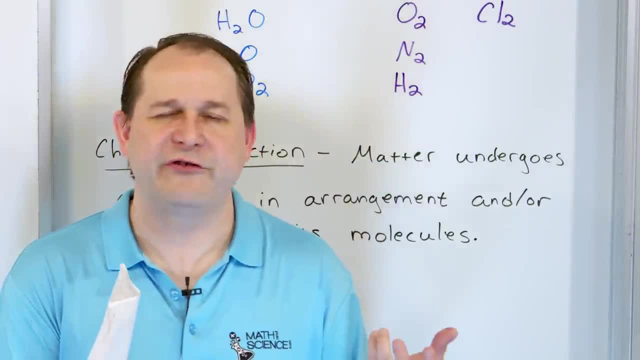 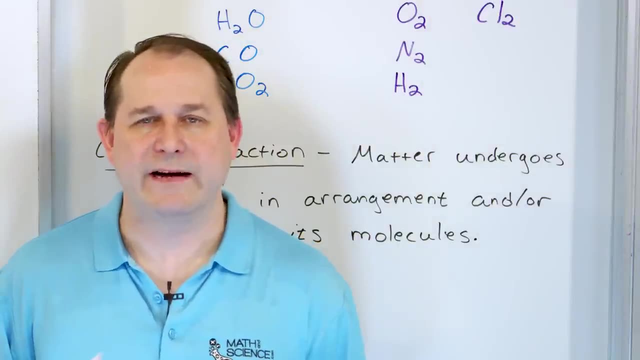 everything was already stable and the electric forces that were present were just not strong enough to overcome that and rearrange the things into something new. so nothing happens. It literally boils down to that. In a few chapters from now we're going to talk about properties of the 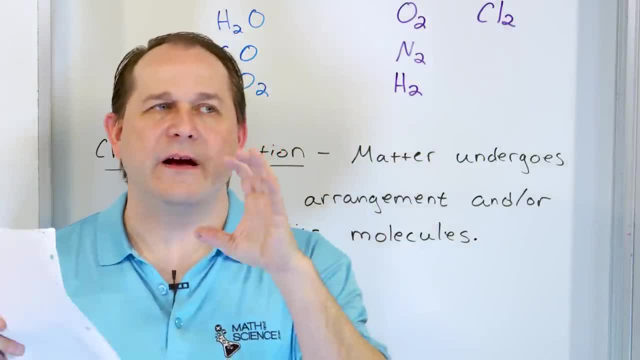 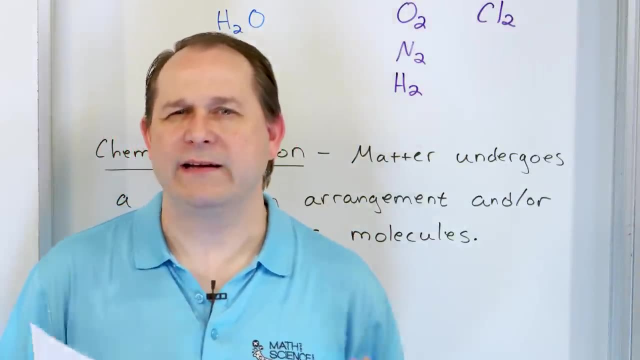 periodic table. We're going to talk about how readily does an element donate an electron or give up an electron or take an electron right. When does that happen? How readily does that happen? We're going to talk about the boiling point and the melting point of substances. 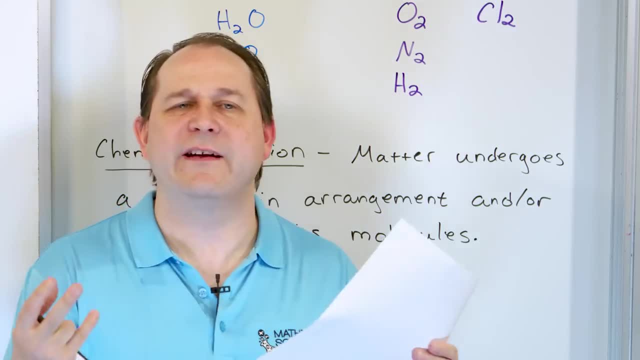 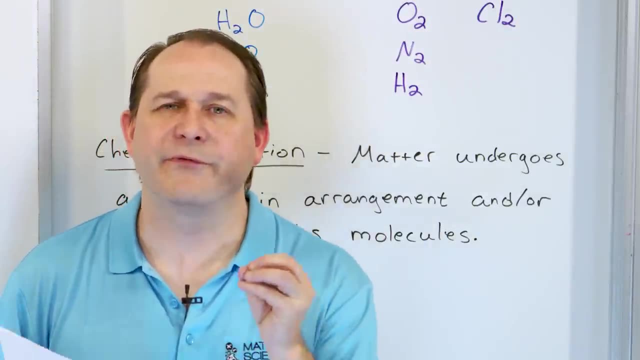 We're going to talk about. how often or how much energy does it take to take an electron from one atom and move it over to another atom? right? All of that stuff comes from the strength of the electric force, right? The strength of the electric force governs everything. It governs the properties. 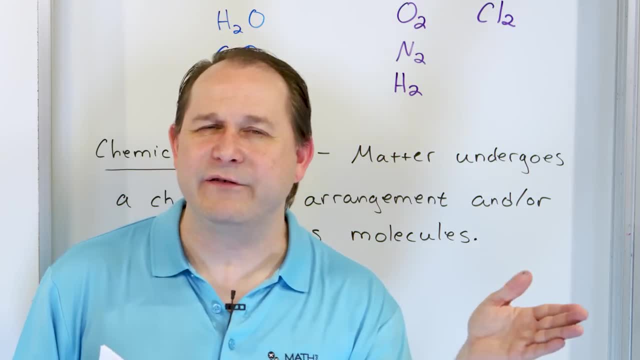 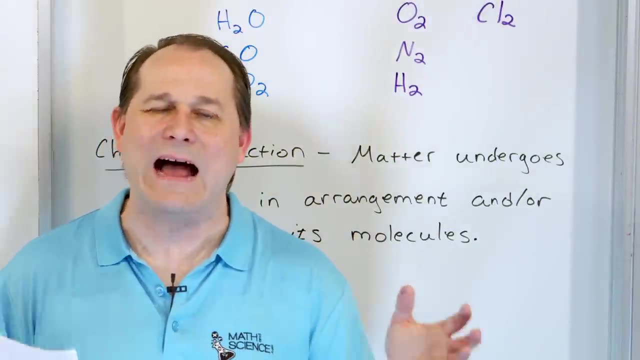 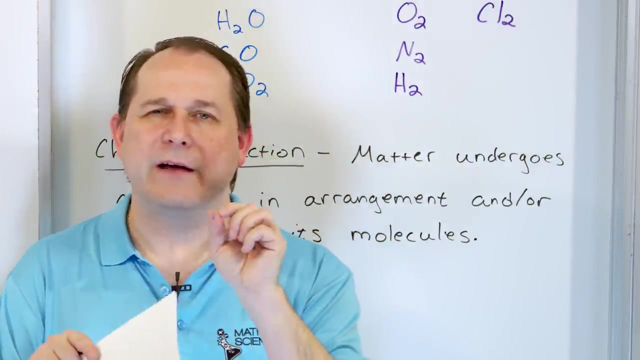 of the atoms on the periodic table. How easily do they give an electron away? How much do they want to take an electron from someone else? All of that stuff is coming from, how strong that electric force is. Later on, when we tell you the rules to try to figure out what's going to happen, because 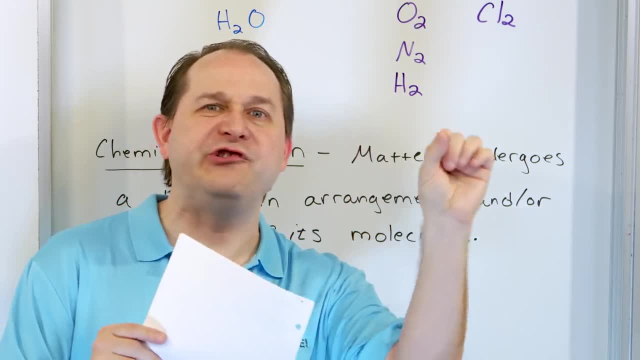 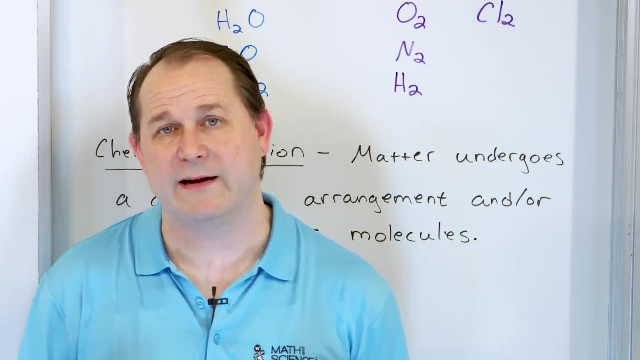 all of this chemistry is happening because electrons are being shared or transferred between the two things you're mixing together and then things can be rearranged into a new set of products, right, But that transfer of electrons, the sharing of electrons, that might happen. the 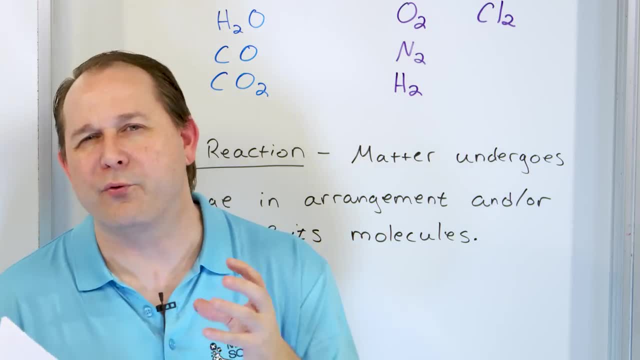 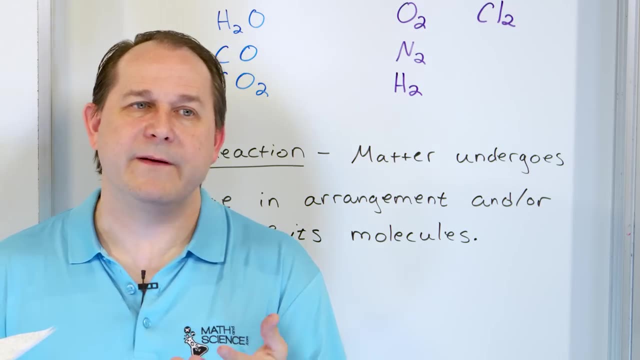 rearrangement that might be happening to give you the product. it's all predicated on that electric force being strong enough to make it happen, And when it is strong enough to make it happen, then it happens. But if the situation was already so stable so that the electric forces there are not going to make, 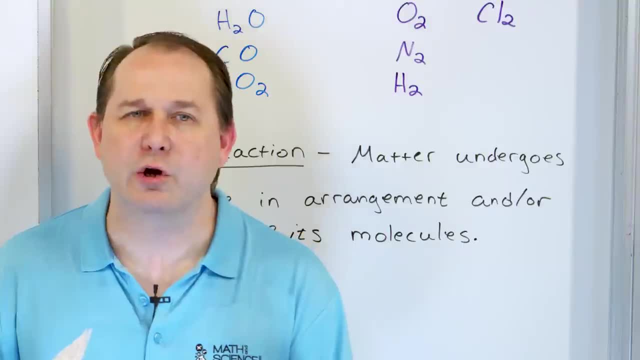 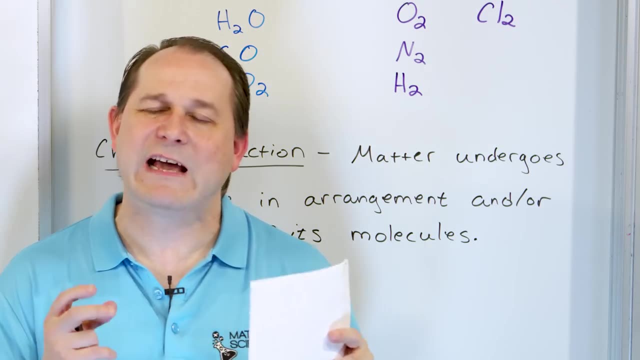 any changes, then nothing happens. And all of those properties that we learn about a little bit later in the periodic table, they all come from understanding the strength of the electric forces, Because you've got to remember, and I know we haven't gotten into it yet, but I know- 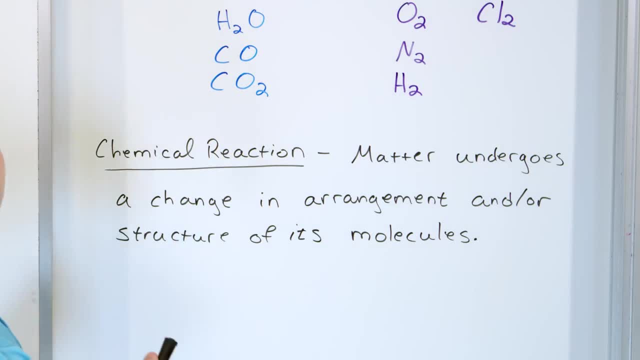 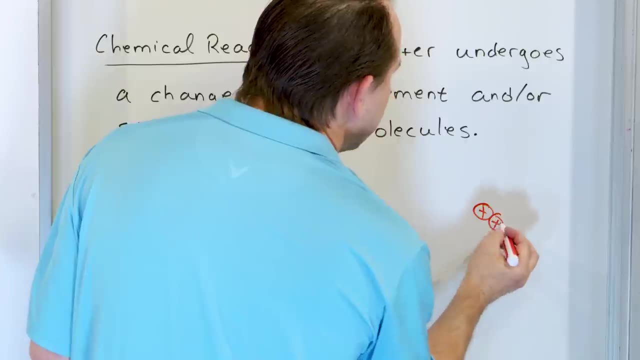 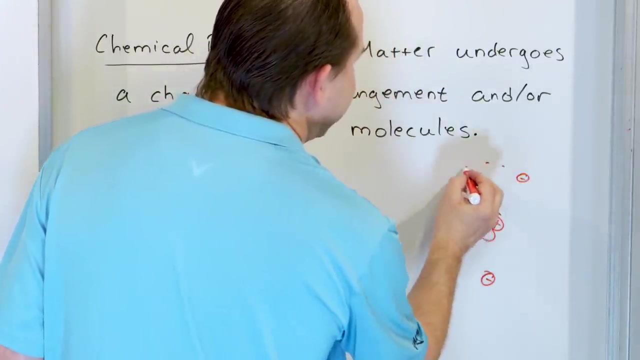 that you all know that in the center of all of these atoms we have little protons, right, Maybe you have more than one right- And then you have maybe a couple neutrons that really don't have any charge at all. And then on the outside maybe there's a couple of electrons And we say that 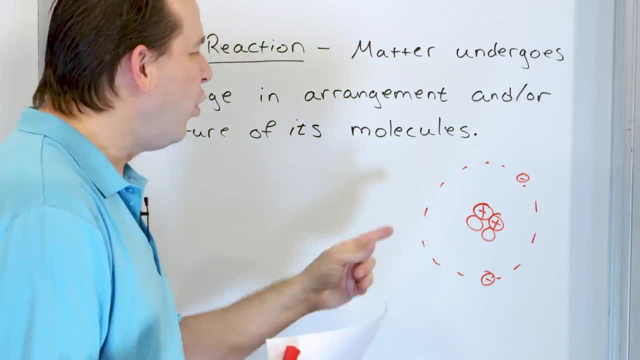 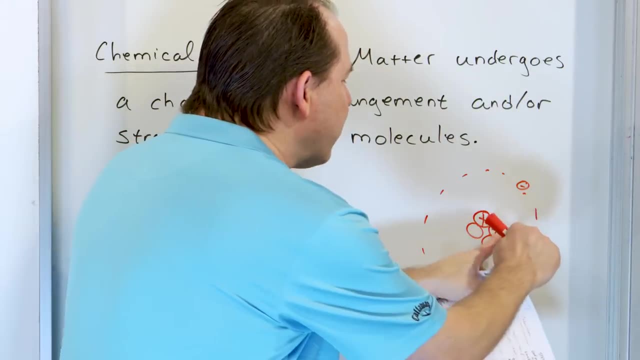 the electrons kind of go around and they kind of orbit. Now there's a whole lot more to this. It doesn't really really look like that, but that's the picture that we tell everyone to understand, And so we know that the protons and the electrons are attracting each other, And once you understand, 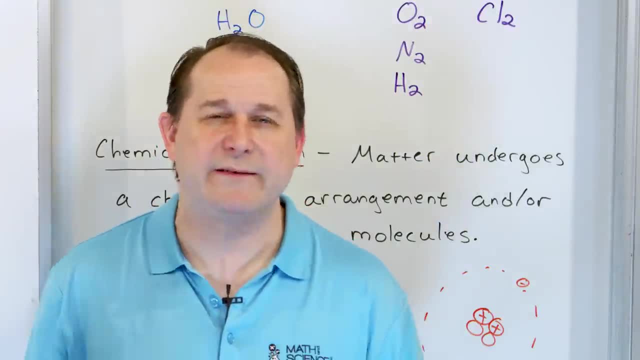 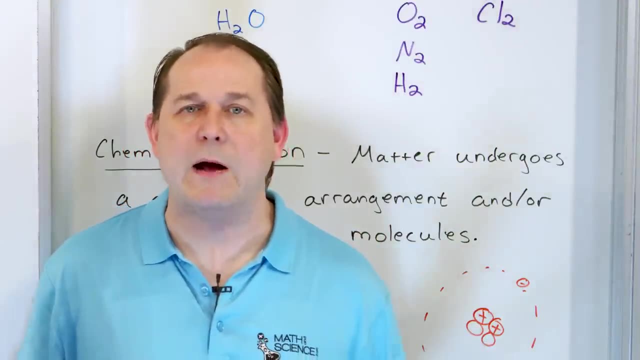 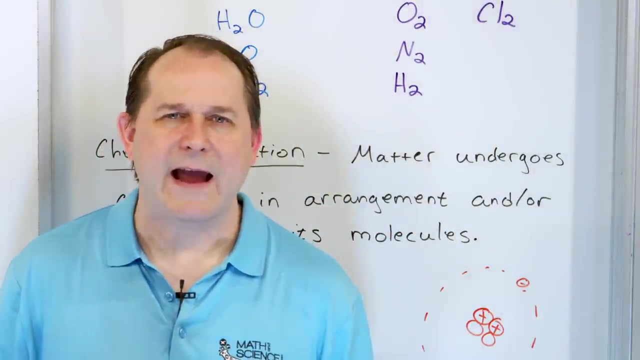 that the strength of that attraction is millions and millions of times stronger than gravity, then you can understand how all of the chemistry that you learn in this class is dominated by what that force is going to do. Now you might say: if it's so strong, why don't I feel it every day? I mean, I don't feel anybody. 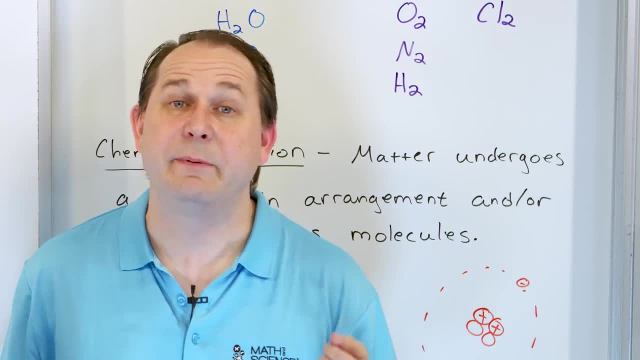 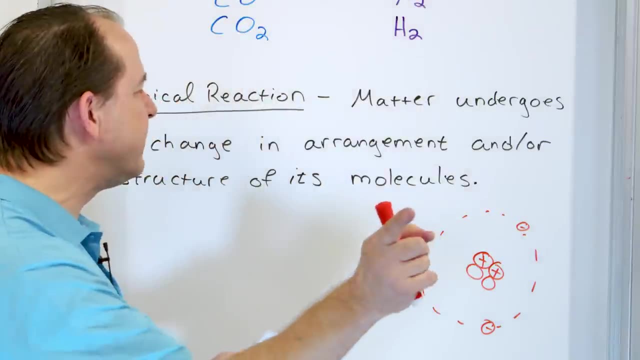 pulling on me okay. Well, the reason you don't feel it is because if you look at this atom and you zoom out, you're going to see two protons and you're seeing two electrons. So from a million miles away then you're going to see an equal and opposite amount of charge. And when you have an 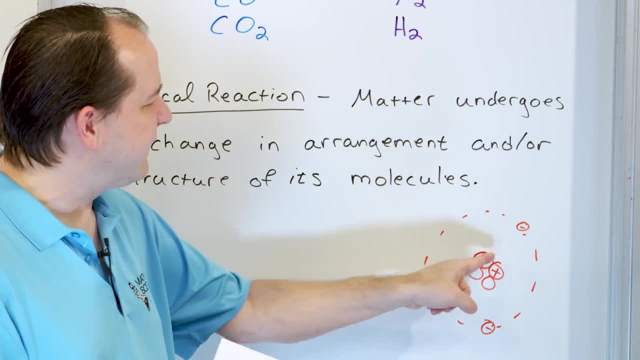 equal and opposite amount of charge. you're going to see an equal and opposite amount of charge. What happens if you add- Just think from algebra- Plus two, and this is negative two, because these are negative. What do you have when you have plus two and you add to it a negative two? 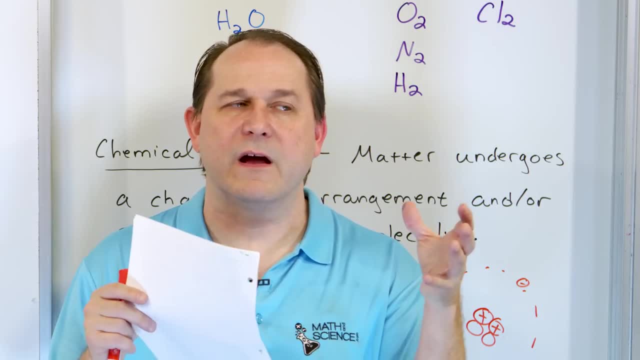 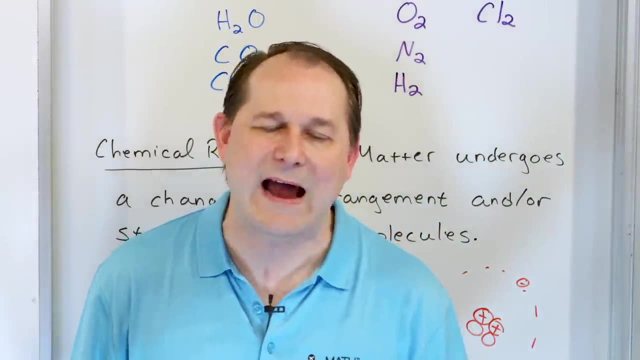 You get zero. So anytime you have an equal and opposite amount of charges, then from a distance, far away, it looks completely neutral, It looks like zero charge because everything cancels out. But you see, in chemistry things don't cancel out, Because in chemistry if you bring two things, 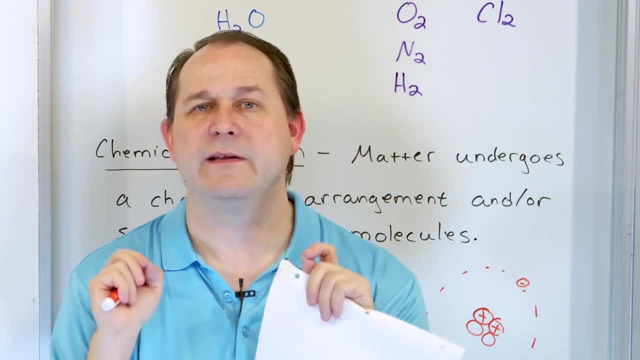 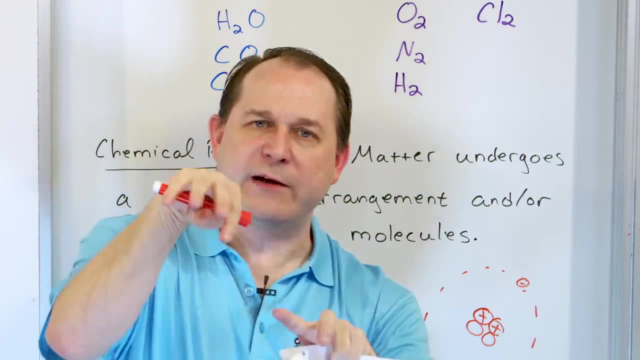 together. one electron may get shared between the molecules, Or maybe it's just a matter of jumping from one atom to another. Then you have a charge imbalance. Then things start moving around and try to attract and rearrange themselves into a more stable configuration. That's what's. 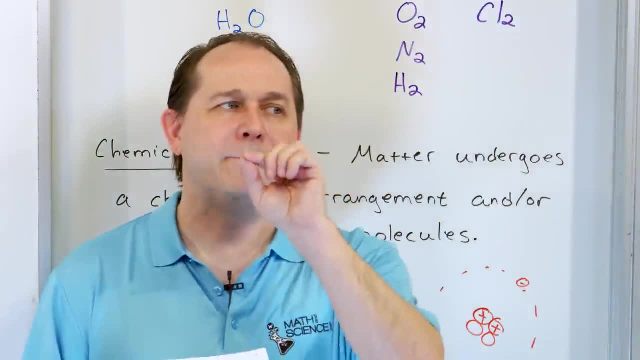 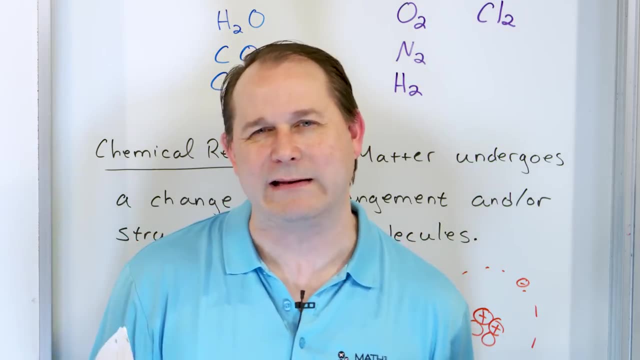 called a chemical reaction. But that chemical reaction is driven by the electrons that are moving and the forces that come about when electrons start becoming unbalanced and start moving around like that. And I know I went on and on and on about it, but I just I got to tell you. 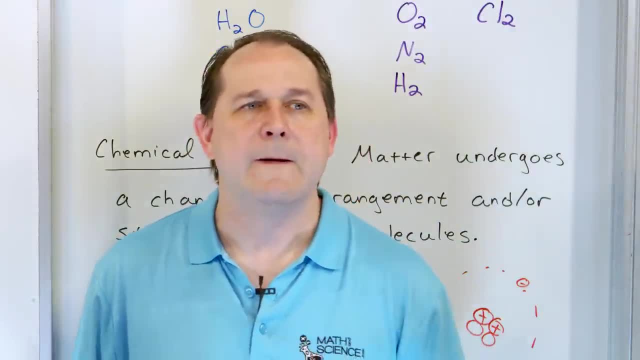 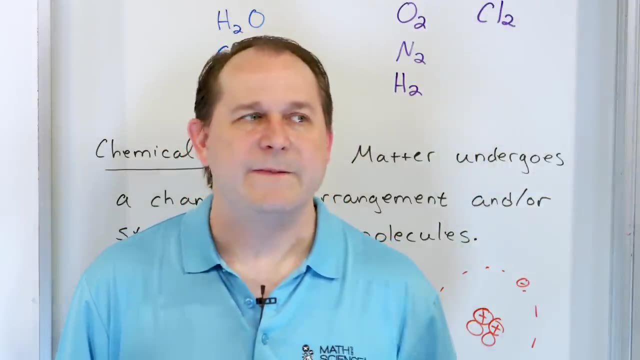 this early on because I could go six chapters in and then explain it to you. But I'm not going to. But then it's like man. that would be a wasted opportunity for you to understand that this electric force is millions of times stronger than gravity. I'll leave you with one final thing before. 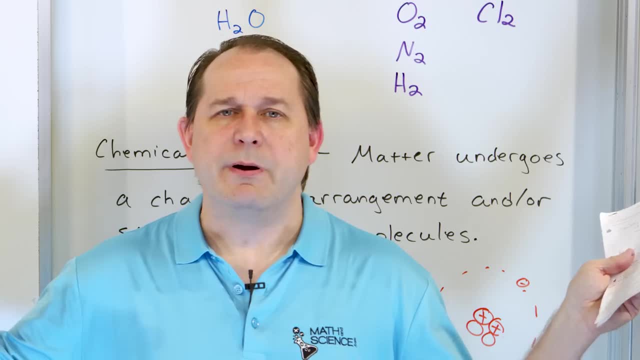 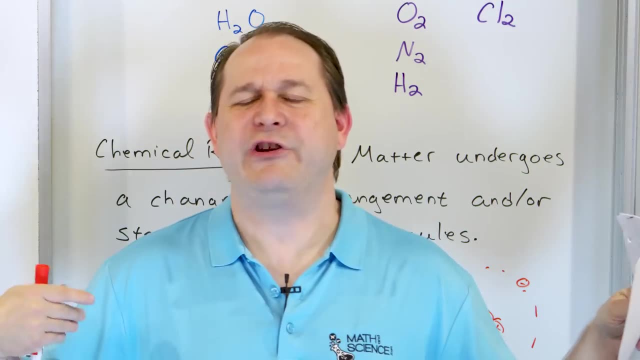 we move on. I'm standing here in front of this camera but with the but the energy in my muscles, right, just standing here, I can jump off the ground. just with the energy in my little tiny puny body, I can lift myself and remove myself from this planet. But consider that every atom. 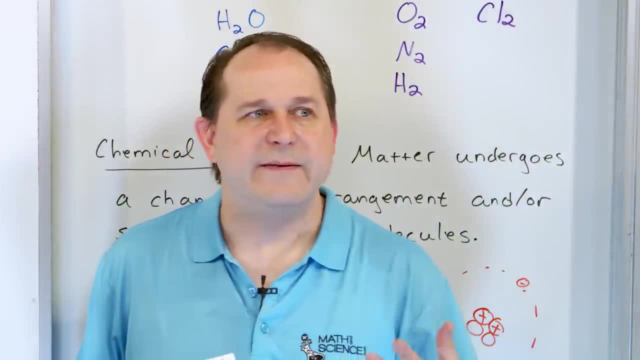 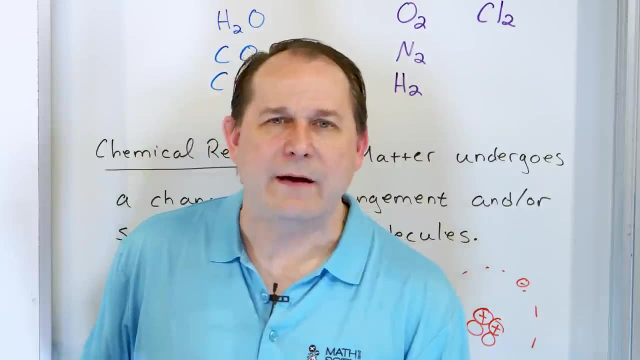 on this planet is attracting my body with gravity- The Himalayas, which are on the other side of the planet. they're attracting my body because of gravity. right, The center of the earth, thousands of miles away, is attracting my body. Someone on the 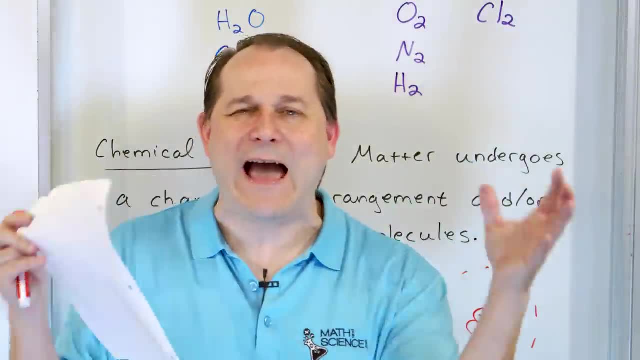 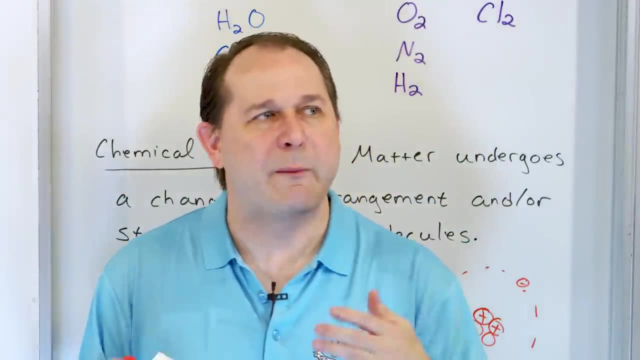 other side of the planet in their car they're attracting. every atom on this planet is pulling down on me, But yet I am strong enough to push up and separate myself from all of that attraction with my little bitty muscle energy. That tells you that, even though we kind of think as gravity, 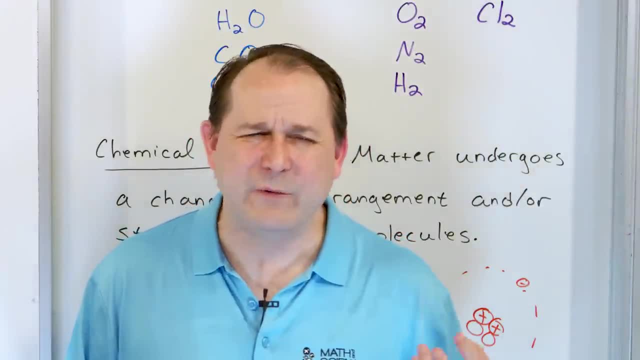 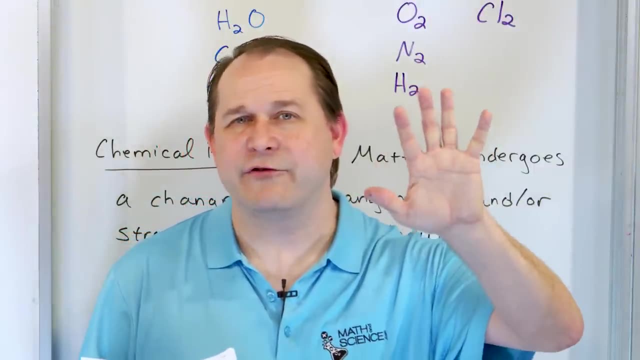 is being strong. gravity is actually really weak, right? It's really not that strong at all, And when you do the math, which I'll do for you one day, you will find out that the equation that governs gravity, which I could write on the board, 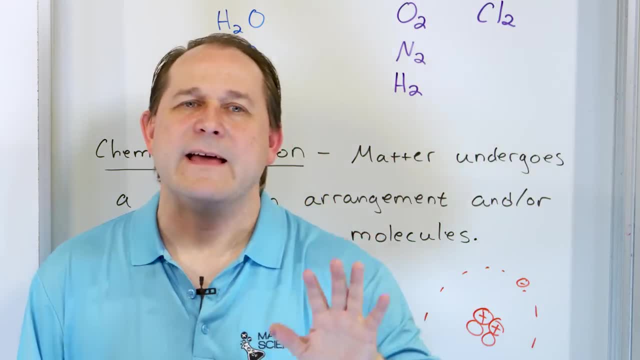 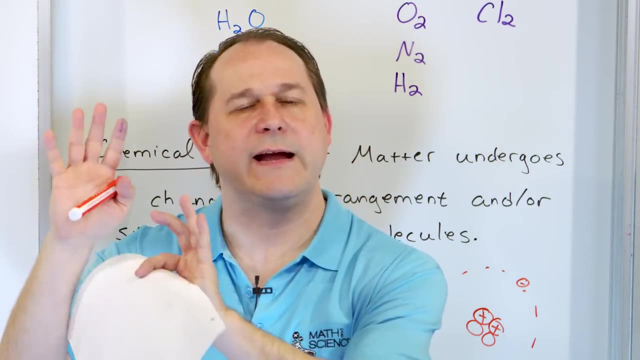 but I don't want to do it too early because we're going to save some stuff for later. right, It looks almost exactly the same as the equation that tells you how two electrons repel, or how an electron and a proton attract each other. The equations look the same, They have the same. 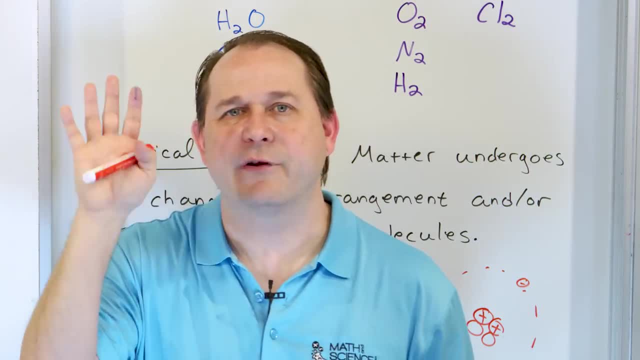 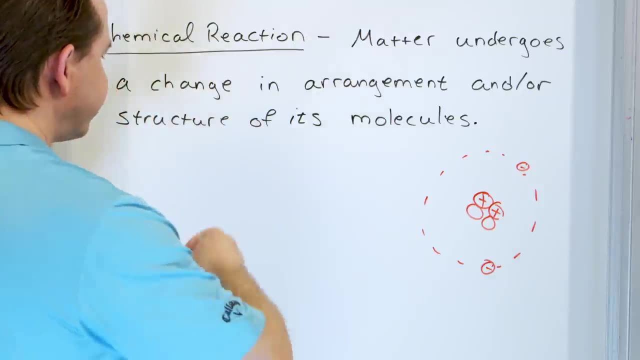 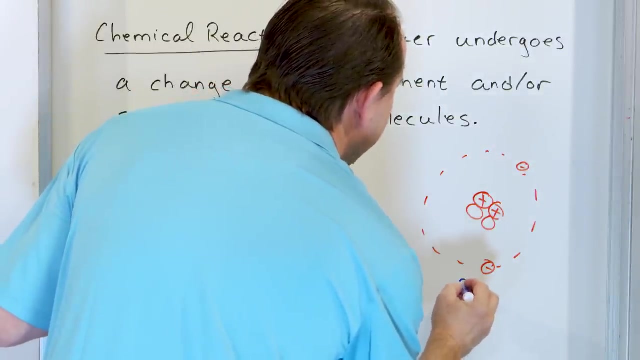 force. They have the same form. I mean, however, the electric force is millions and millions and millions of times stronger. In fact, just to give you an idea of how much stronger it is, if you remember back from math, if you have 10 squared, that's 10 times 10, which is 100, right? 10 squared means 10 times 10 is. 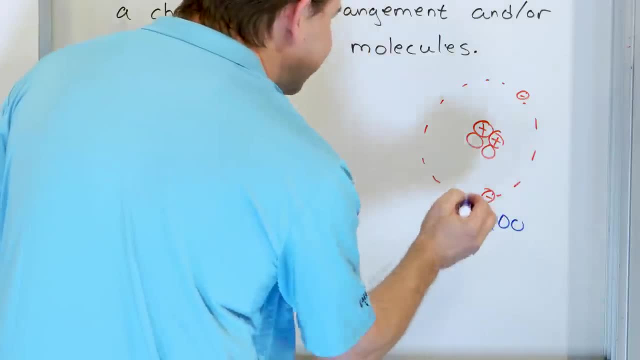 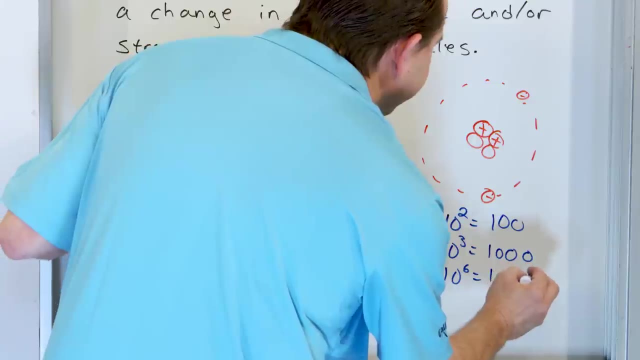 100.. If you have 10 to the third power, that's 10 times 10 times 10, that's 1,000, right. If you have 10 to the sixth power, that's 1,000,000, right. So you see what's going on, Because the number that you have in the exponent, that's 1,000,000.. So you see what's going on, Because the number that you have in the exponent that's 1,000,000, right. So you see what's going on, Because. 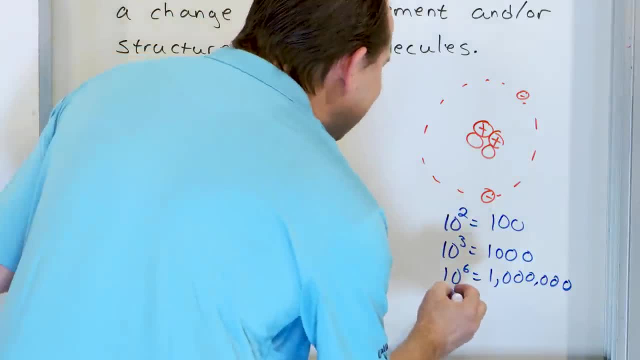 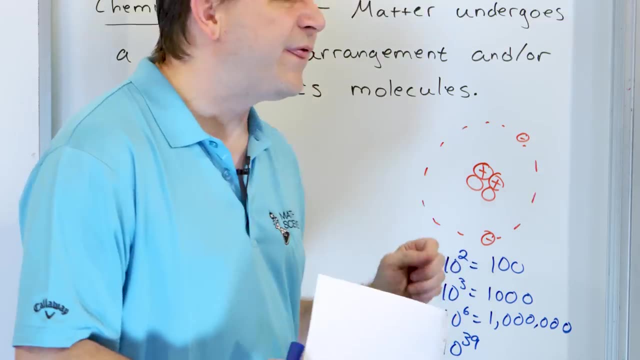 you have 10 to the third power, that's 1,000,000.. So you see what's going on Because the how many zeros you have here. So there's six zeros here because of this. But the electric force is actually 10 to the 39th power, stronger than gravity. That is a one with 39 zeros at the end. 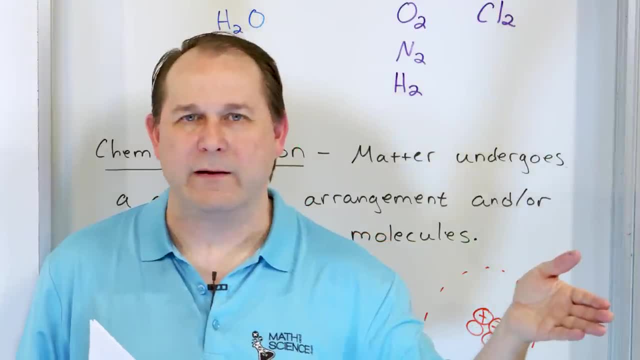 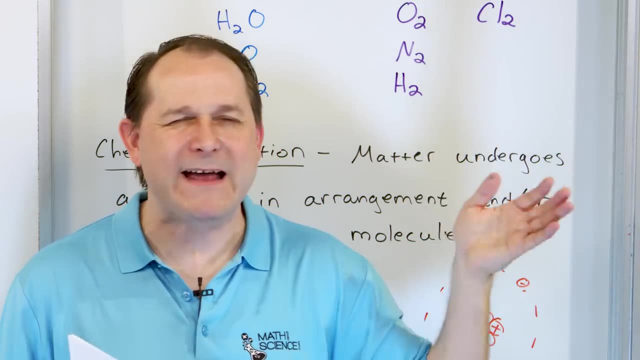 Think about it: A million is only six zeros after the one, But the electric force is a one followed by 39 zeros. That's many, many, many, many, many millions of times stronger. The only reason we don't see it is because we have equal numbers of electrons and protons. That's why we 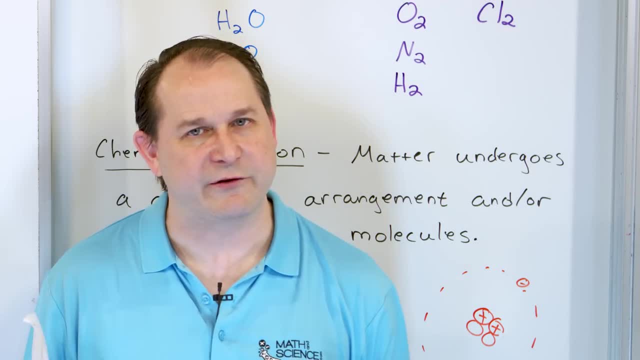 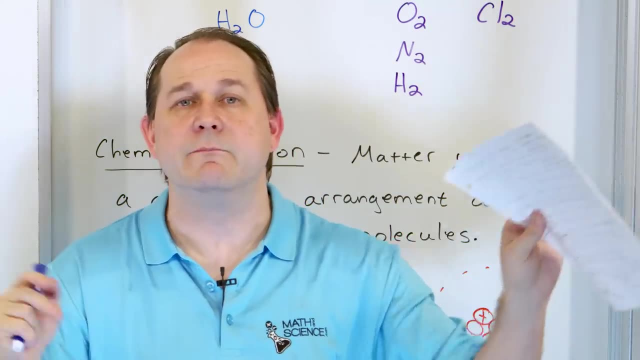 proton, so they cancel each other out. But in chemistry they don't cancel each other out because when one electron moves from one atom to the other, you have a charge imbalance and that causes everything to move to find its more stable positioning, which leads to what we call, when we 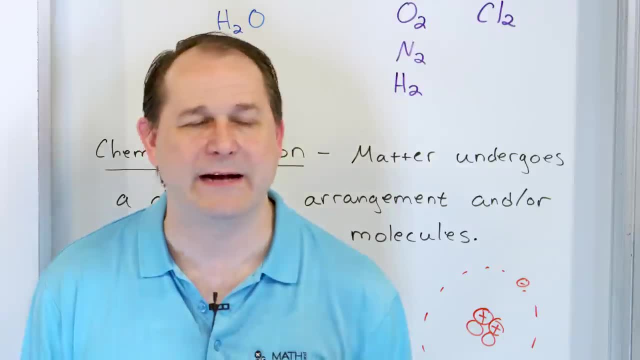 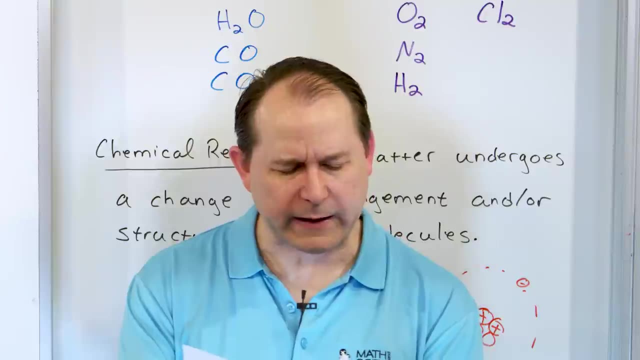 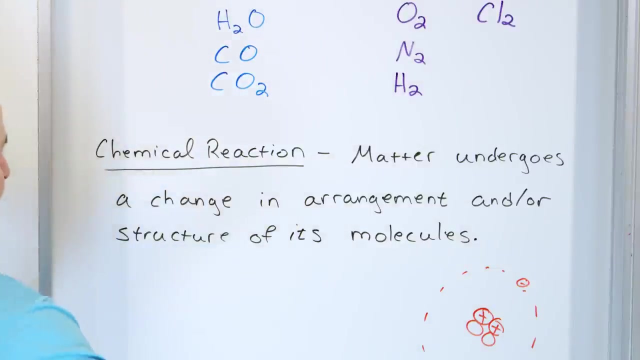 study this stuff, chemistry. That is why chemistry is happening. That is the stuff that you could spend the rest of your life studying if you really wanted to understand it in great detail. All right, So chemical reaction. Let's move on to chemical reaction, And then we're going to wrap. 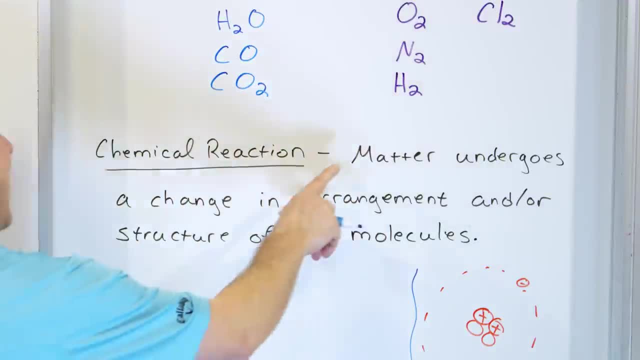 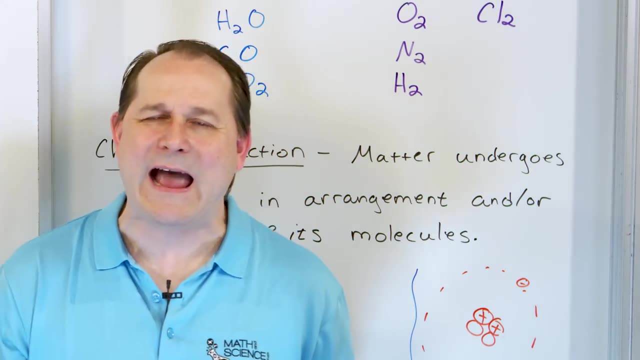 it up here. Chemical reaction is when matter undergoes a change in arrangement and or structure of its molecules. And now you know, all of these chemical reactions are really happening because the electric force is so strong that if there's ever any imbalance anywhere, things are. 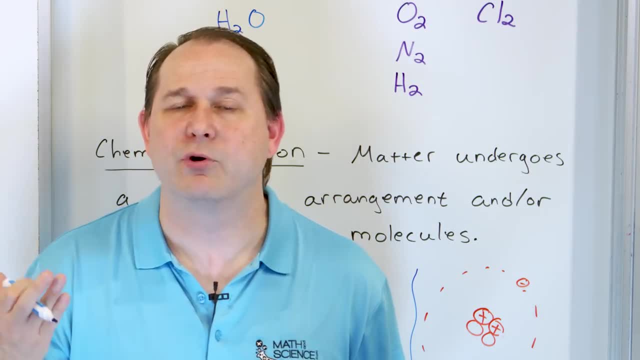 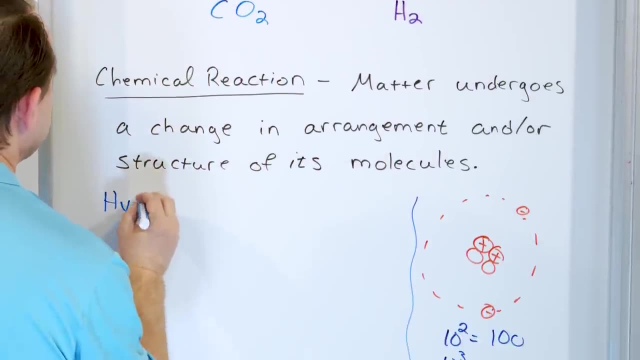 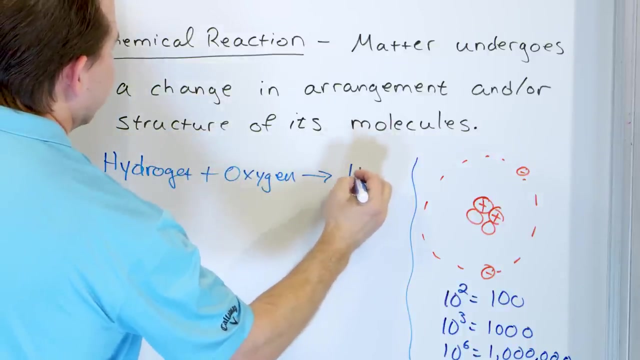 going to rearrange to get to the lowest, more stable configuration of a state. That's what we call a chemical reaction. And that's what we call a chemical reaction, And that's what we call a chemistry. And of course, the big one, hydrogen, right plus oxygen, gives you water, H2O, I could. 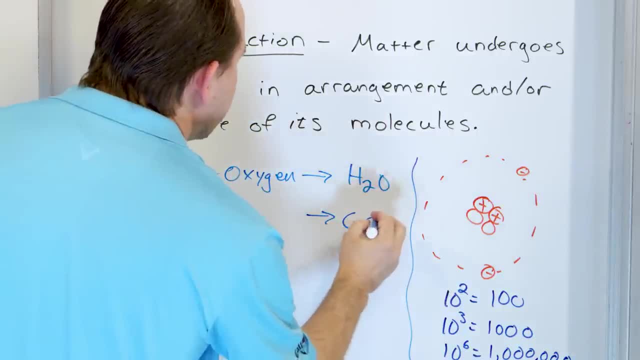 write: carbon plus oxygen gives you either carbon monoxide or carbon dioxide. Why does it form carbon monoxide with one atom of each sometimes, And why does it form carbon dioxide with two atoms of oxygen sometimes? Well, we're going to talk about that. It does different things in. 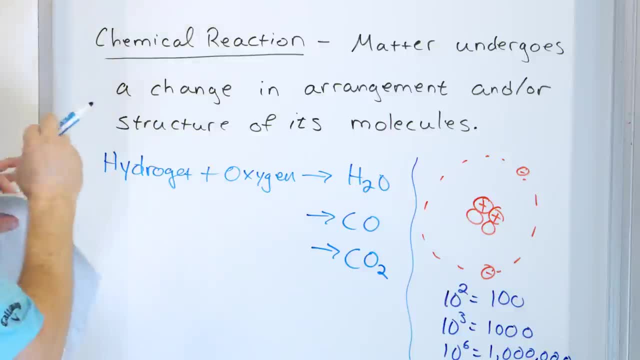 different situations, But when you combine these two things, you're going to get a different thing, And when you combine these things together, the electrons are transferred or shared in such a way that whatever we form on the end, here is a more stable configuration than what we started. 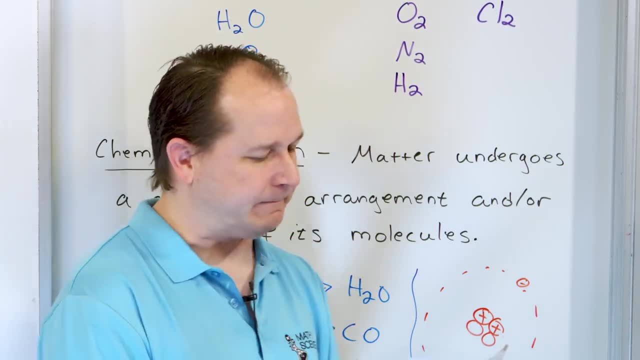 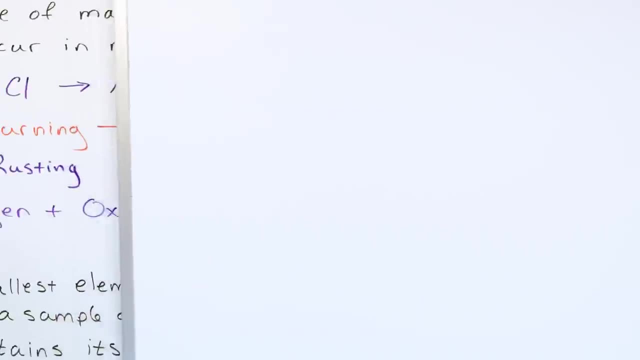 with. We're going to talk a whole lot more about what that means in a little bit. All right, Moving right along. we've talked about molecules. We talked about chemical reactions. Let's move back over here to the beginning. I promise we're almost done here. Let's talk about elements. 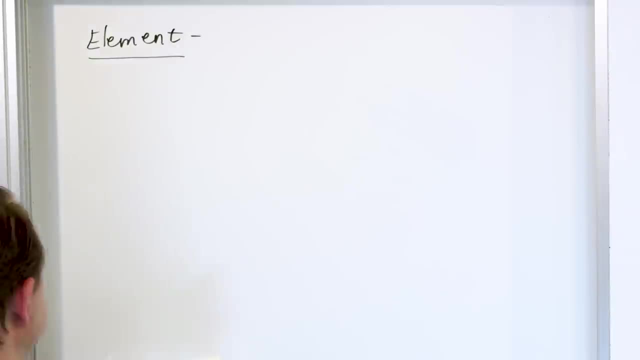 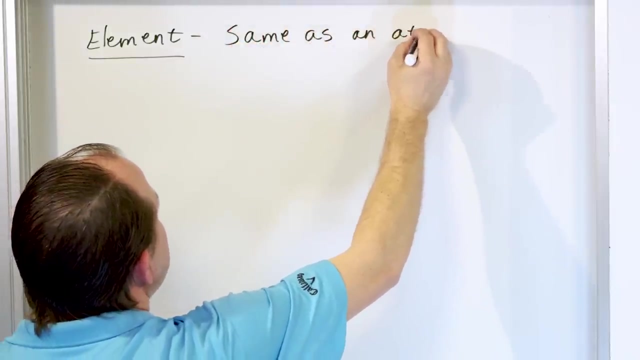 Now I know that you've heard the periodic table of the elements. You've heard me use the word elements For our definitions. we're going to say it's the same as an atom. If you hear the word atom, if you hear the word element, they mean the same thing From our point. 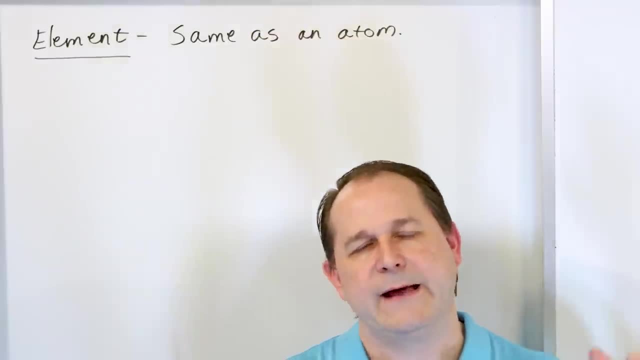 of view. I'm not saying there could be some other situation down the road where you might have something going on different. But for us, if I say here is an element of the periodic table in your mind you want to say, well, that's just a different kind of atom, That's a unique atom. 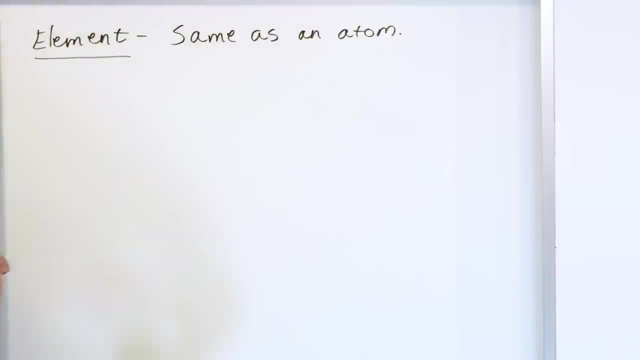 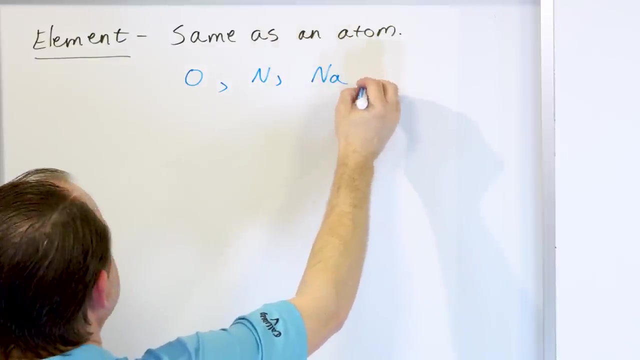 that we have listed on this thing called the periodic table In elements. you already know. We have oxygen, We have nitrogen, We have sodium, which goes into table salt, sodium chloride. We have argon And we also have things like neon. You might see those. 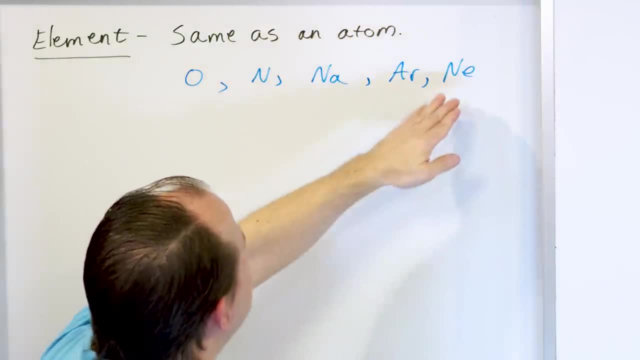 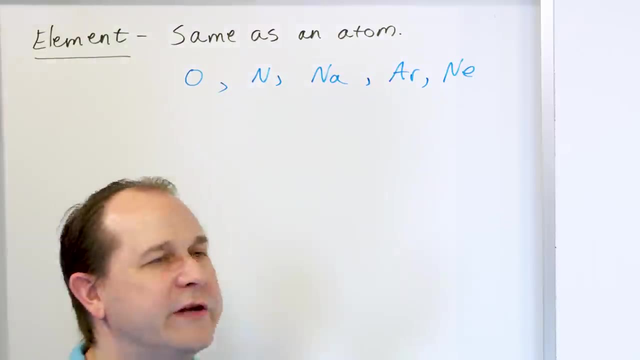 neon, signs that glow, orange or whatever. So we have all of these different symbols on the periodic table. We call it the periodic table of the elements. You could also call it the periodic table of atoms, because elements and atoms are the same thing. Moving right along. 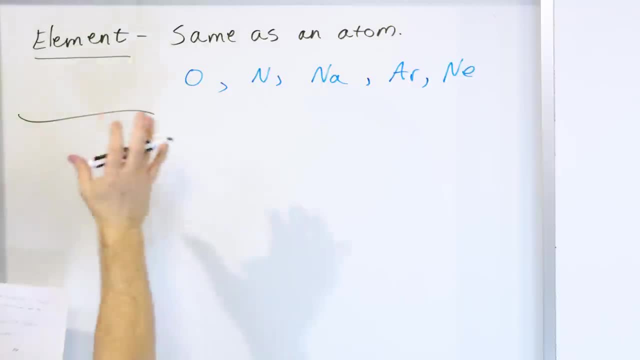 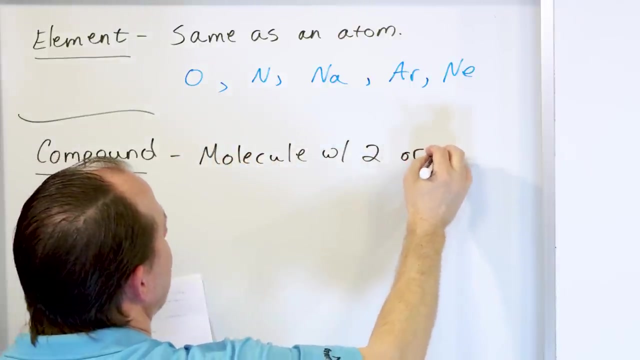 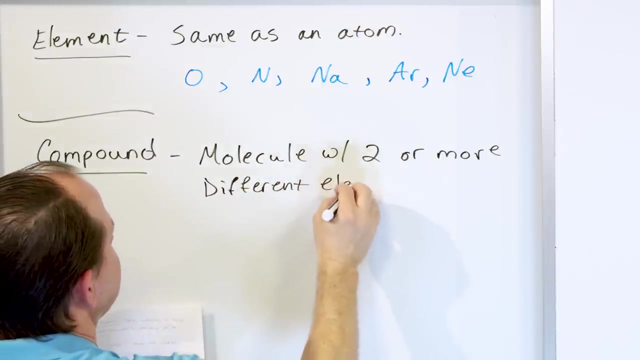 we've discussed this before, but we're going to dot our i's and cross our t's right here We have the idea of a compound. A compound is basically a molecule with two or more different elements. You might say: wait a minute, how is that different than a molecule? Let's go back to the 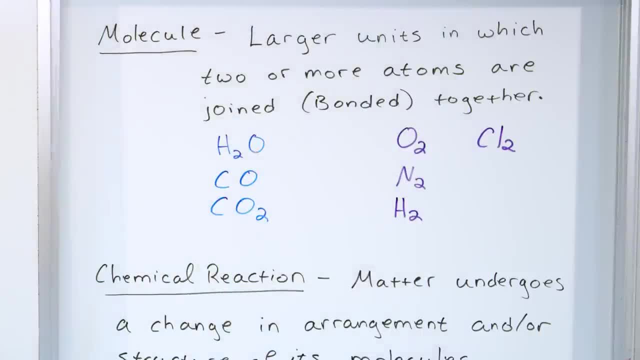 definition of a molecule. That's why I wrote everything down. A molecule is a larger unit in which two or more atoms are joined, bonded together, And we can give lots of examples. So a molecule is any time a molecule is like the general class of what's going on- A molecule. 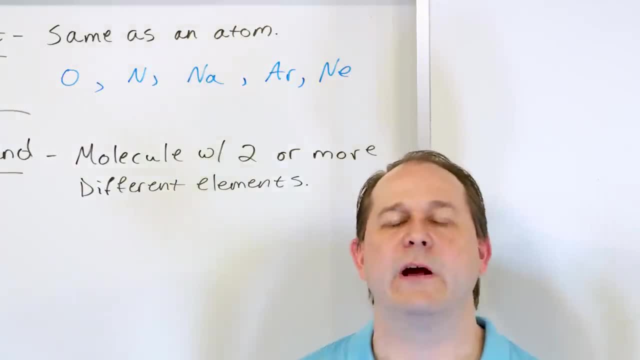 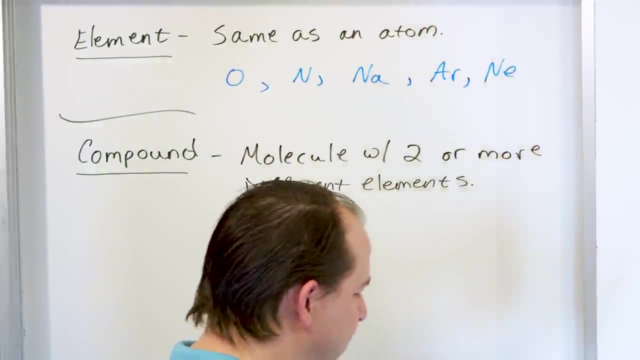 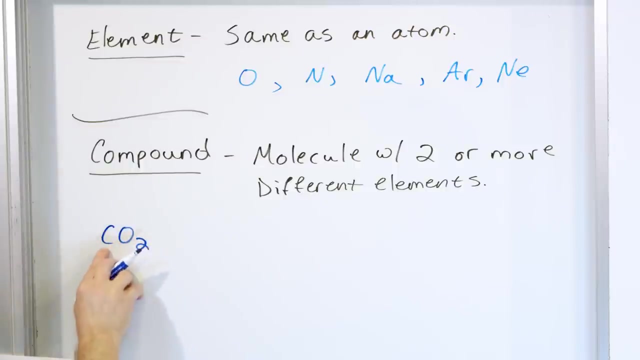 is any time you have two or more things coming together in what we call bonding. Almost everything in chemistry we study is some sort of molecule. Not always, but very, very often. Let's give a couple of examples. Let's talk about CO2.. This is carbon dioxide. One atom of carbon, two atoms of oxygen bonded. 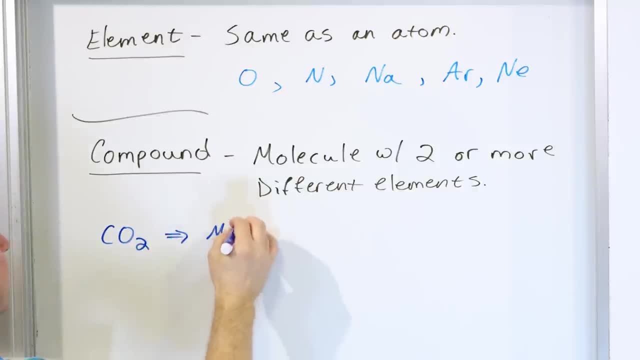 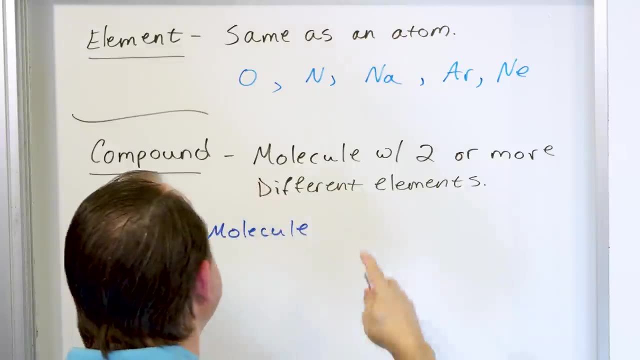 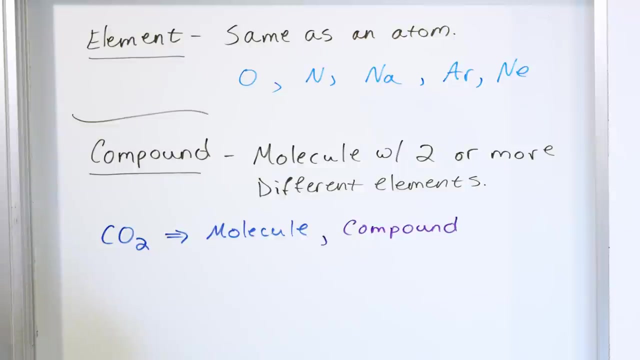 together. Now, this is a molecule. How is it a molecule? Because it's two or more things that are stuck together. Any time that happens, it's always called a molecule. But this is also called a compound. Why? Because these two elements that came together were different. 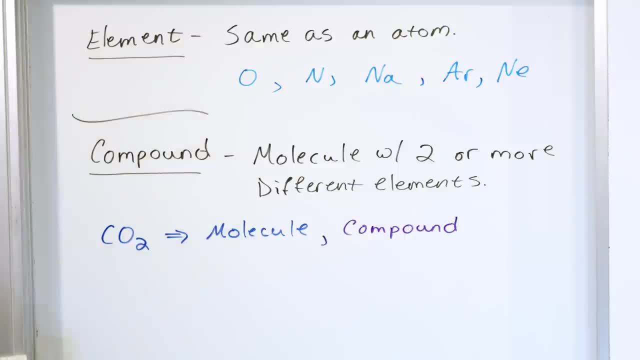 When they're different, we call them. we call it a compound that comes together. What about the famous H2O right? This is a molecule. I'm going to put little quotation marks. It's a molecule. It's also a compound. because it's a molecule? because it comes together two or more different. 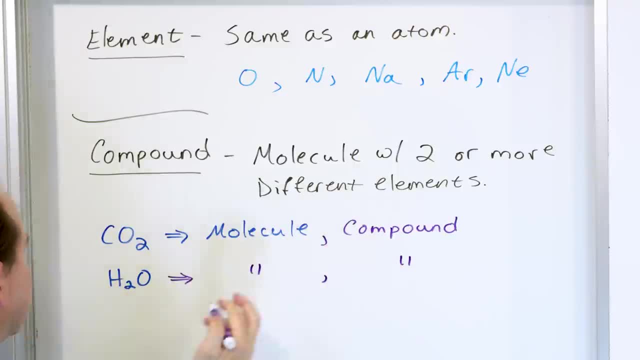 things And because they're different elements that come together, it's called a compound. What about the famous H2O2?? You know what that is? H2O2 is hydrogen peroxide. You use that to clean cuts, right. It is a molecule, because it is. any time two or more things come together, Notice. 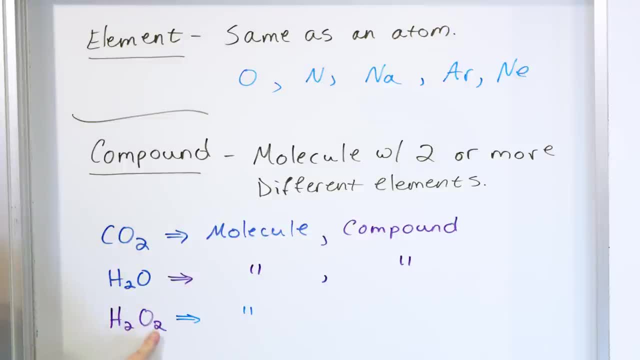 we have four atoms here: two atoms of hydrogen and two atoms of oxygen. So it's four atoms here. but it's also a compound, because it's different elements. So you might say: well, wait a minute. Everything you've listed here is a molecule and a compound, So when can it? 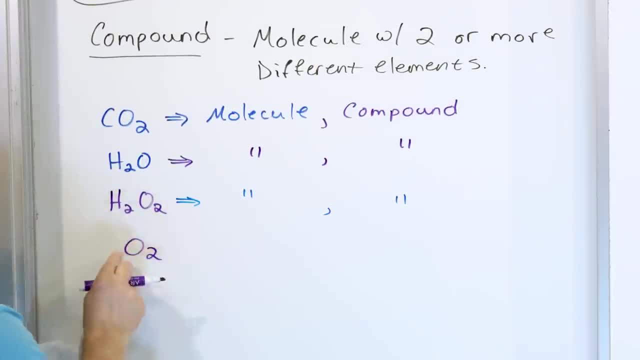 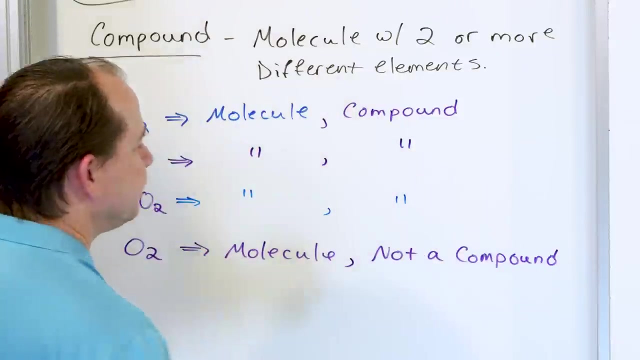 be different. Let's talk about the oxygen molecule. You know, just call it O2, right? Well, this is a molecule because it's two or more things stuck together, but it's not a compound. It's not a compound, right? The reason it's not a compound is because it's the same element stuck. 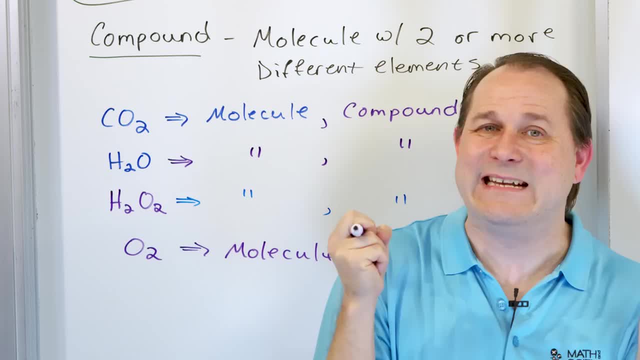 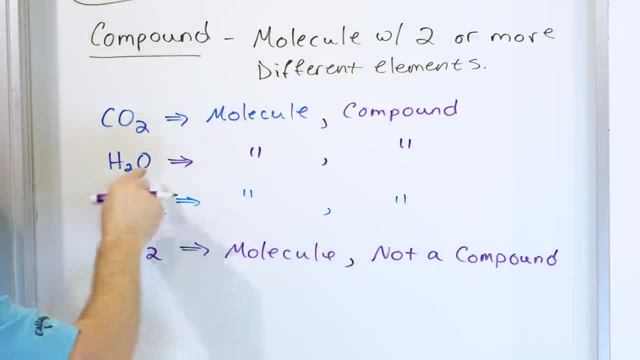 together, It's only a compound. when it's two or more differently named, different items that come together, then it's called a compound. These are different and they're stuck together. So it's a molecule and a compound. These are different, They're stuck together. So it's a molecule and. 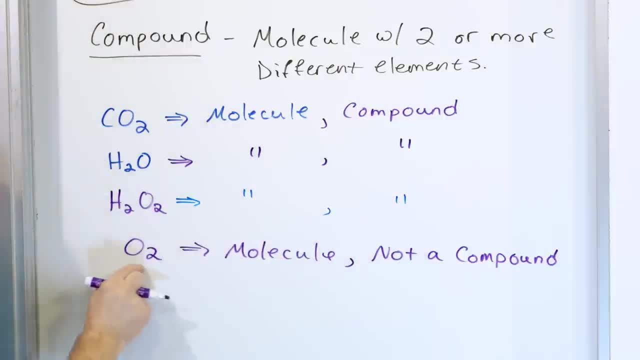 a compound. These are different. So it's a molecule and a compound. These are the same atoms. So it is a molecule, but it's not a compound, right? What about nitrogen gas? Right, Same thing. It's a molecule and not a compound. What about chlorine gas? Well, 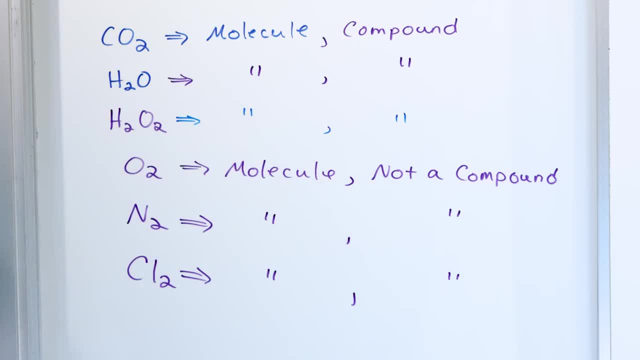 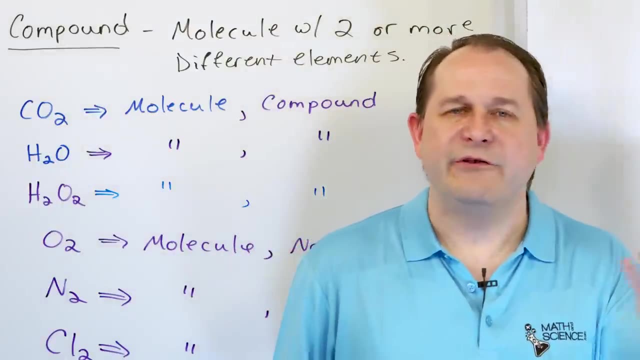 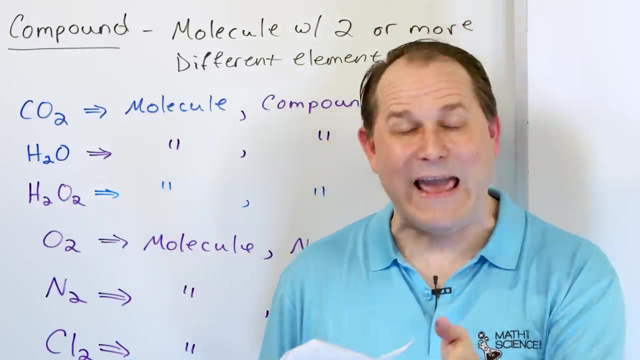 it's a molecule, but it's also not a compound. So I just want you to remember: most of the time, things that we study are compounds, because most of the time, the things you're studying are not the simple ones, like oxygen gas or nitrogen gas, O2, N2, Cl2, H2, hydrogen gas. 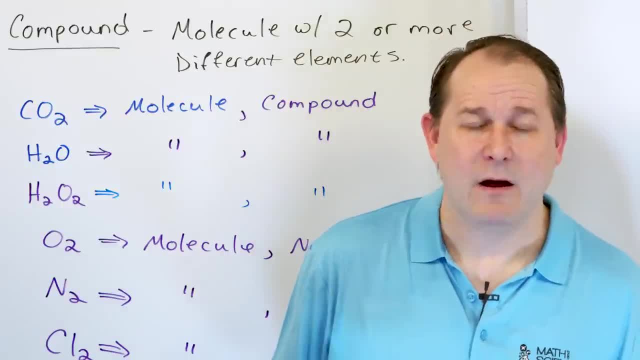 Usually we're studying other things like methane or something like that, with lots of different compounds. So it's a molecule and not a compound. What about chlorine gas? Well, it's a molecule, but it's also not a compound. So I just want you to remember most of the time. 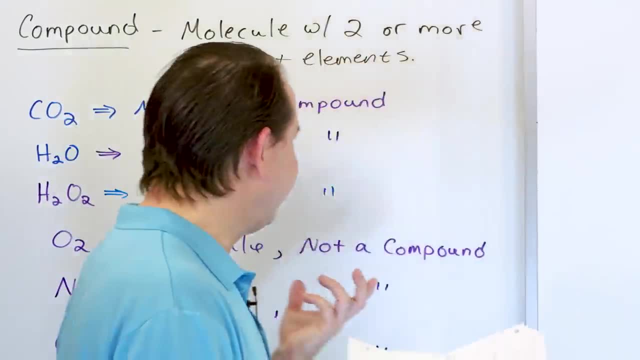 things that we study are compounds. So it's a molecule and not a compound. So it's a molecule, different elements in there. So we almost always call them compounds. But just so you know, it's only really a compound if the things that are made up of that molecule are different items. 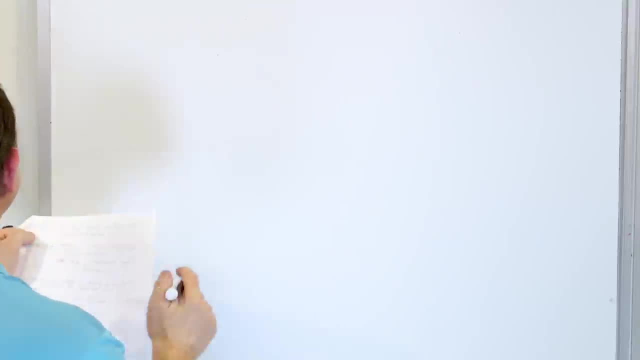 All right, And we're going to round out the tail end of this lesson by talking about mixtures. Now, so far we've talked about chemical reactions. We talked about things coming together, rearranging their electrons, rearranging their atoms. 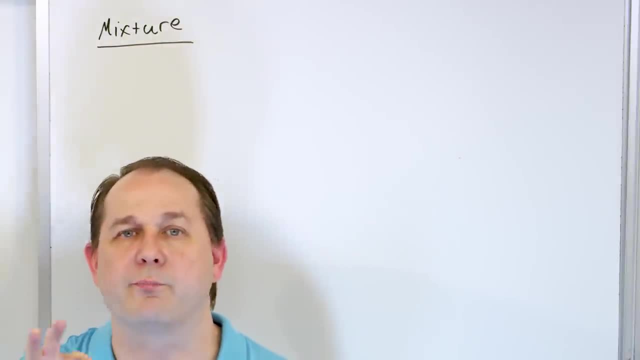 and coming out with a new arrangement which we call the products or the outcomes of the chemical reactions. So we're going to round out the tail end of this lesson with some of the reaction. So that's chemistry, right, But we also have this other thing that we 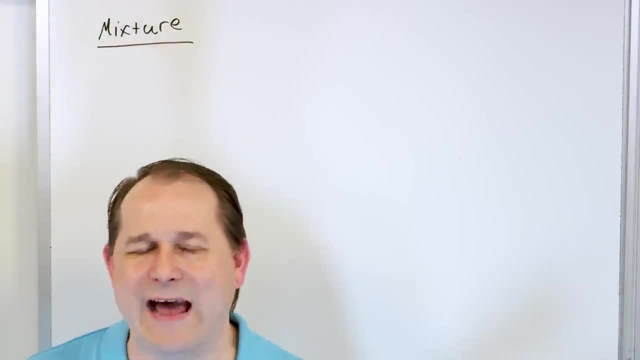 want to compare it with which we call a mixture. In a mixture there's no chemistry happening at all. It's just taking two objects and literally mixing them together, but nothing chemically is happening. So I'm not even going to write down the definition of this, because I think it's easy. 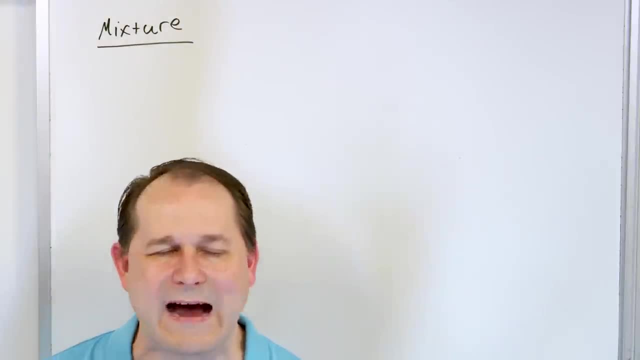 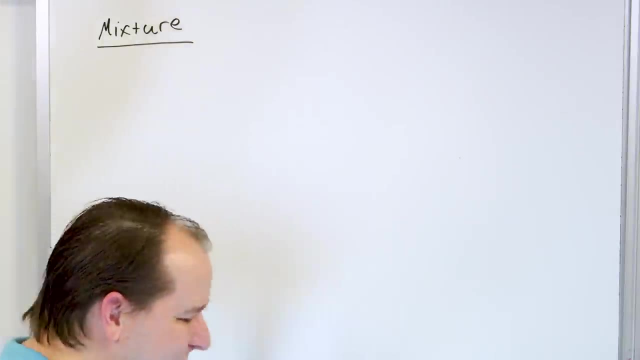 enough to understand. It's basically when you have two or more items or samples of things mixed together, where no chemical reaction is happening. So examples of this, of mixtures, You know well. before I give you examples, let me give you examples of the different kinds of 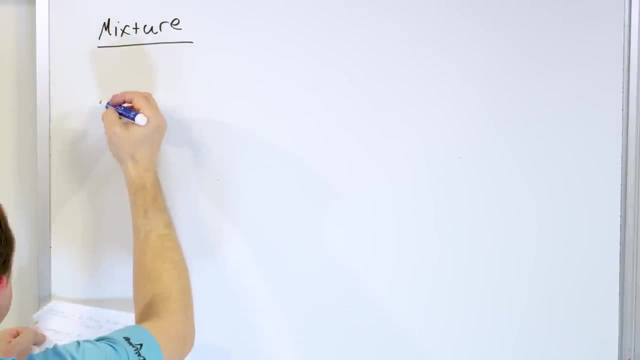 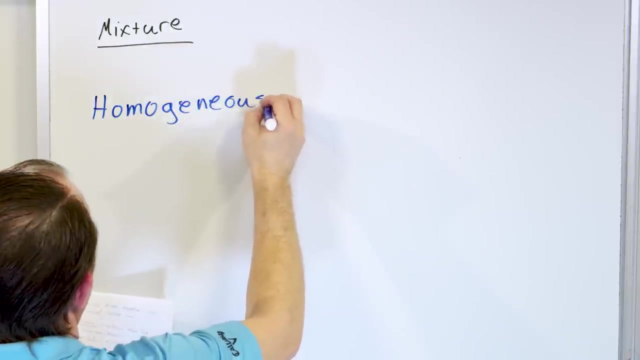 mixtures, and then we'll give specific examples. right, We have two different kinds of mixtures. The first one is a homogeneous mixture. Homo-genious mixture- Right Homo- genius. Homo means same. Homogeneous mixture means that the mixture that you have has the same composition, everywhere Same. 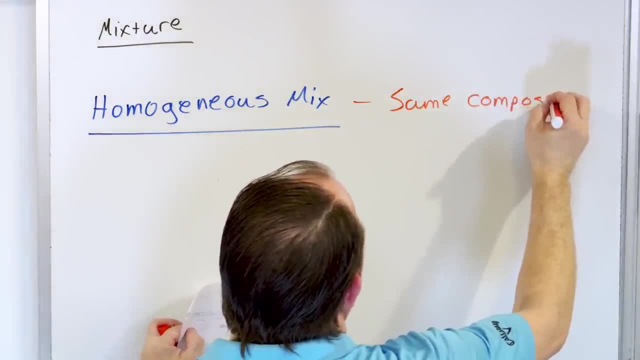 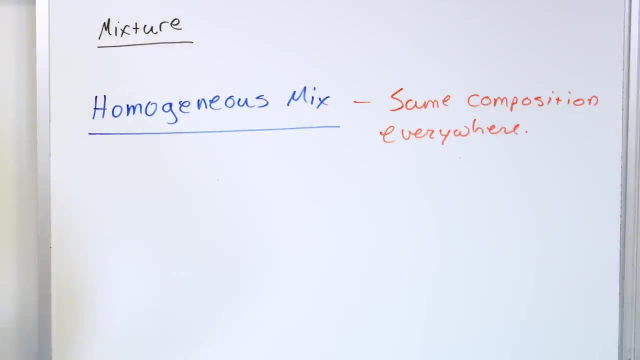 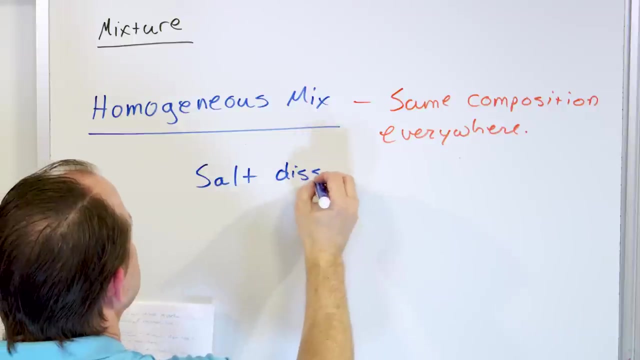 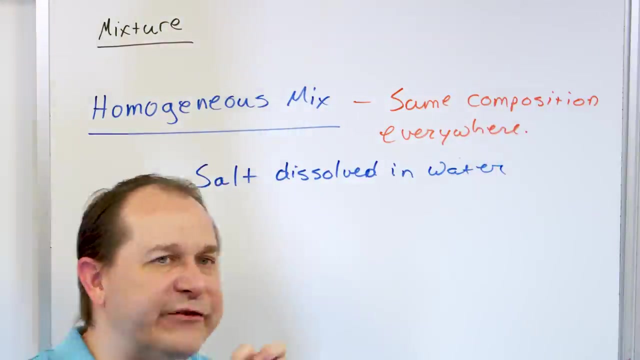 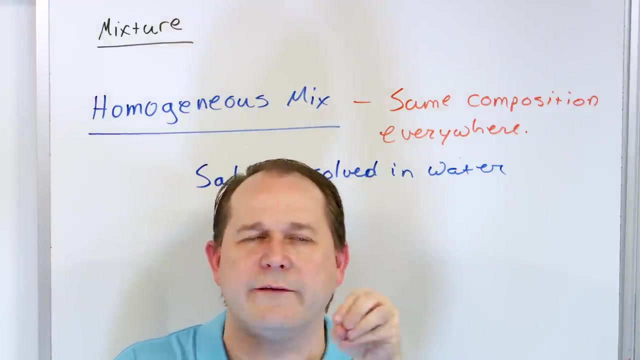 composition everywhere, right. so examples of this right would be something like salt dissolved in water. you know, in water the salt is dissolved and the the the salt is that it doesn't disappear. it's just in between all of the water molecules that are there and, whether or not you take a drink of water, the salt 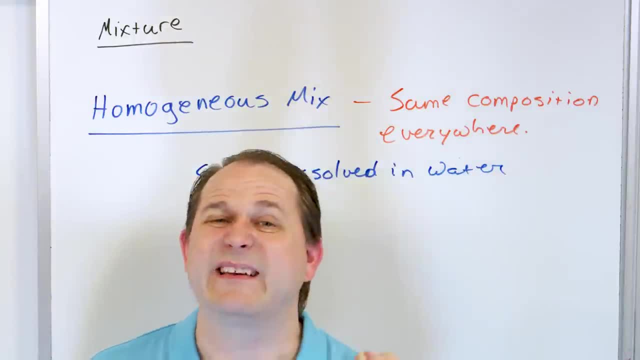 water from the top, or if you take a drink of the salt water from the bottom, it's gonna taste the same saltiness, because once everything is evenly distributed and dissolved, then we have the same concentration of salt everywhere. so that's called a homogeneous mixture, all of these. 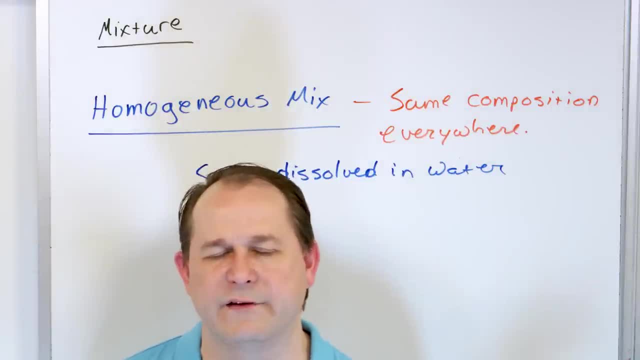 solutions like sugar in water, salt in water, other things dissolved in water. they're going to be homogeneous situations. if you take sand over water and balance it all out in a solid form, just like that, you're going with rocks and pebbles and you mix it up really, really, really good and you have. 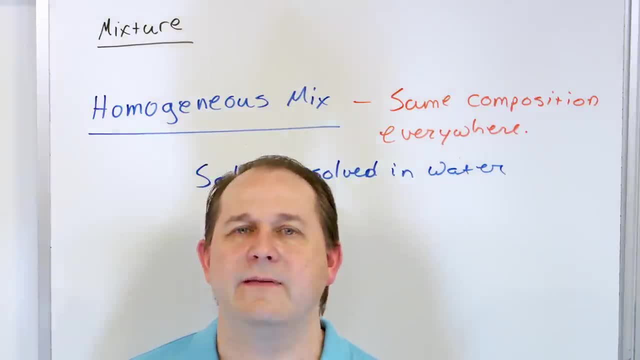 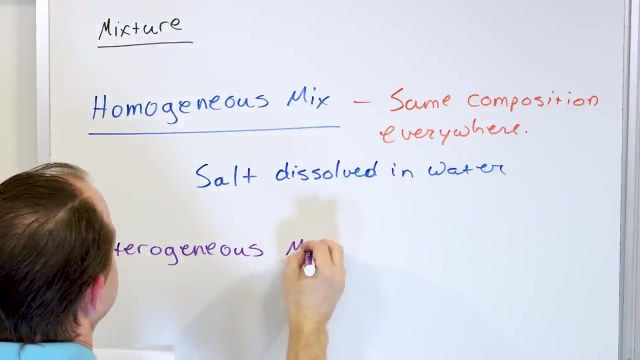 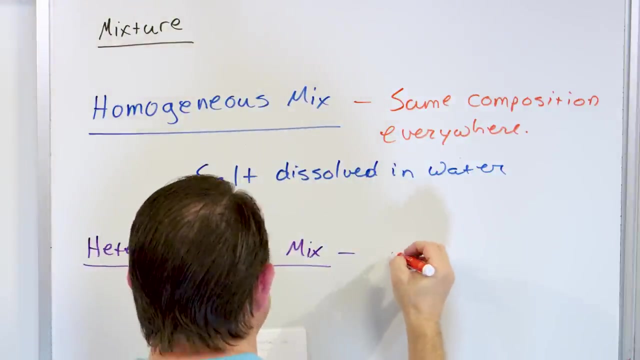 very uniform situation, no clumping. that's what we call a homogeneous mixture. but we also have the situation where it's not homogeneous. we have heterogeneous mixture, we have the heterogeneous mixture. so homo means same, hetero means different, so different, different composition in the mixture. so what we see here when we have a heterogeneous mixture, is the it varies in. 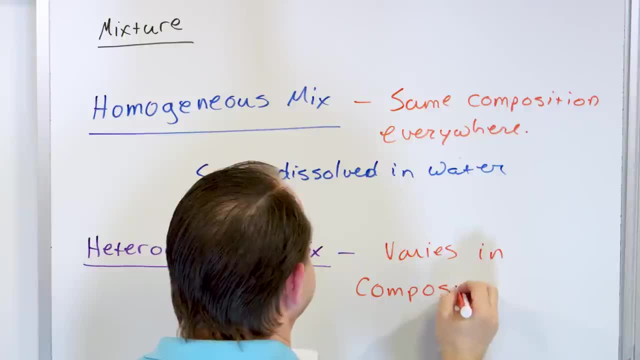 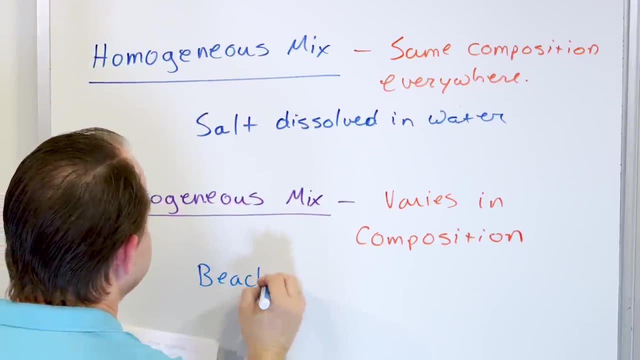 composition. so here I'm gonna put as an example, I'm gonna put beach sand. now you could mix the sand. it really really well. but if you don't really mix it, if you take one of the first two mixtures, and you take one of the first two mixtures, 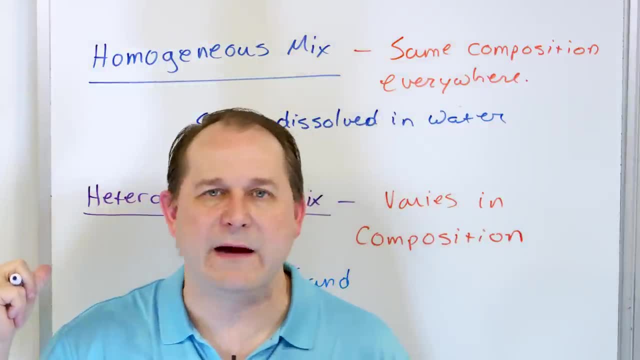 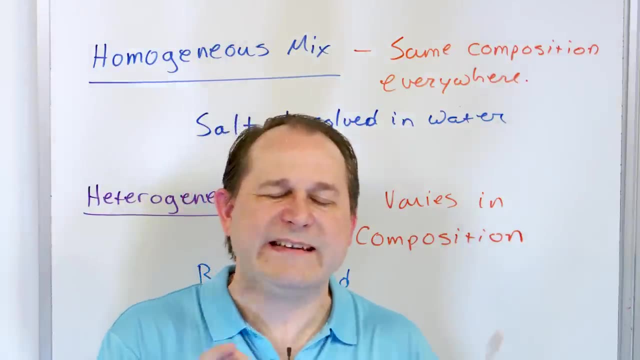 scoop of sand from one part of the beach and then go five miles away down the beach and take another sample of sand, then the compositions are going to be a little bit different, right, Because the sand on the beach has not been mixed thoroughly, It's just deposited by the ocean, so it's going to be. 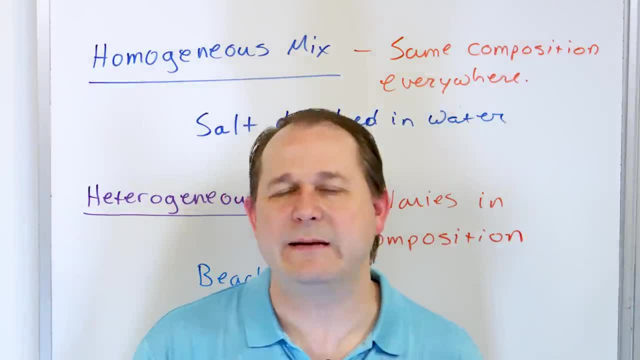 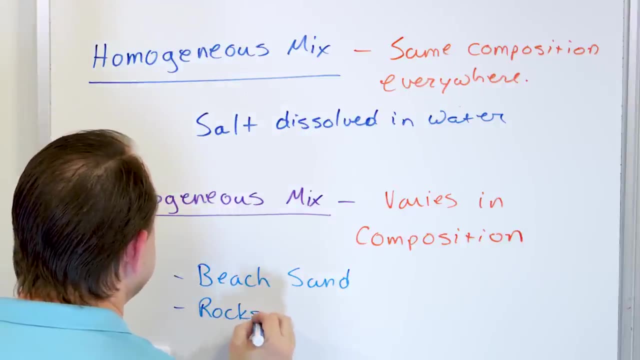 a little different. You're still going to have similar things going on, but it's not evenly mixed or evenly distributed. so we call it a heterogeneous mixture. Another example would be like rocks and dirt. Now, if I mix the rocks and dirt really really, really well, if I pulverize, 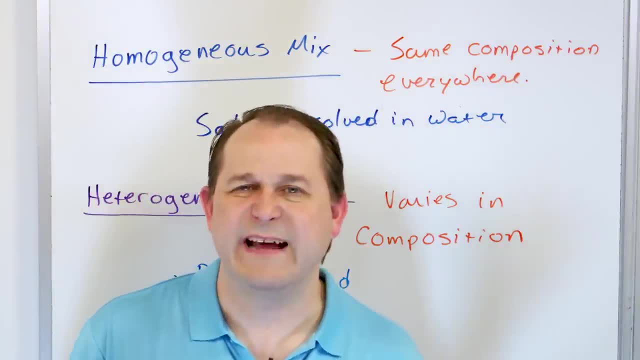 the rocks to get it really uniformly distributed. with the dirt you could say it's homogeneous. but if you just throw some rocks in the dirt and do a little shaking, it's not going to be uniformly distributed. We call that a heterogeneous mixture. So we have mixtures which nothing. 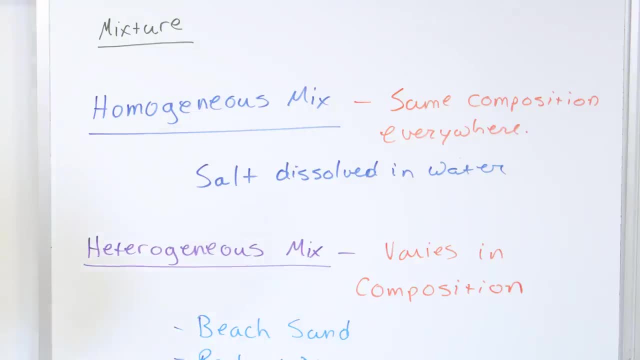 chemically is happening. We just have two or more species coming together and mixing and when you have these mixtures where everything's very evenly mixed, very uniformly distributed, you're going to have a heterogeneous mixture. We call it a homogenous mixture. Any kind of solution where things are dissolved are 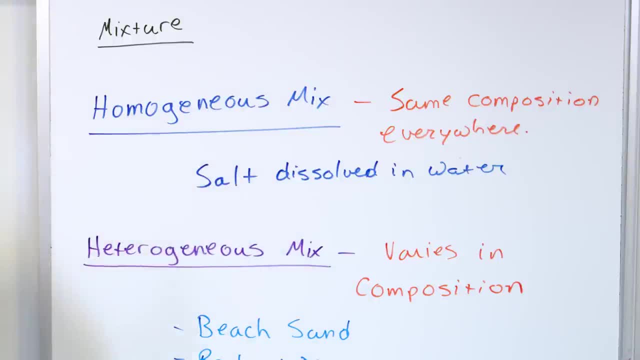 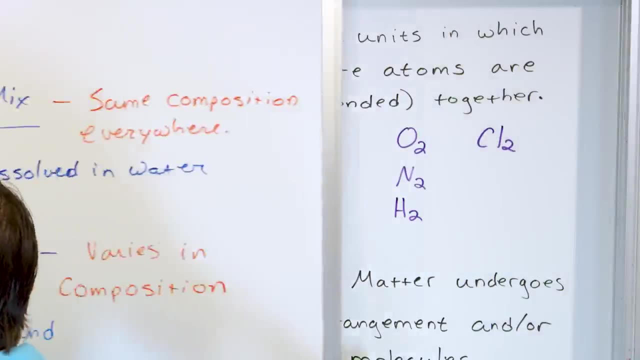 homogeneous. and then you have the heterogeneous mixtures, where things are just clumpy and not mixed very well at all. Now I want to wrap up this lesson with a conclusion, and I do want to wrap this up with a conclusion, and I'm going to do that now, but I'm going to 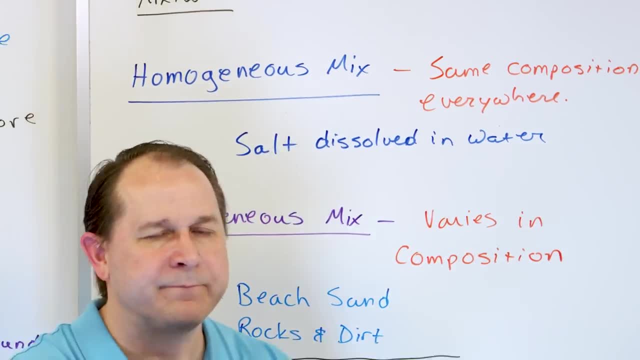 give you a little bonus material at the end. before I do that, because it's on my mind and I don't want to forget to mention it. I'm sure I'll mention it and we'll have entire lessons in the future, but while I'm at it, I'm going to give you a little bonus material at the end. 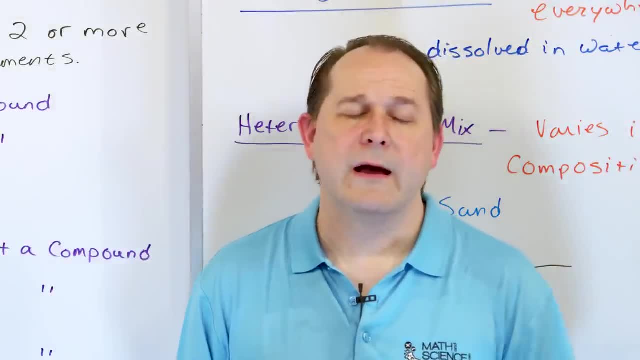 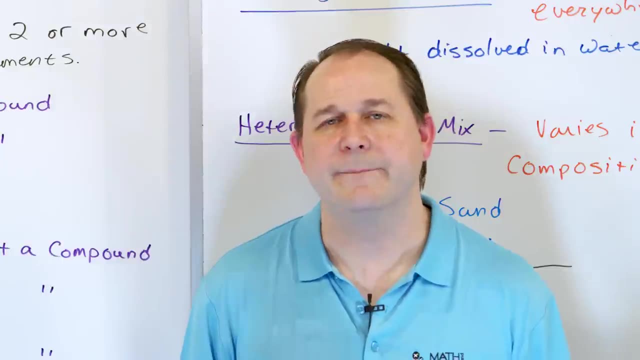 While it's on my mind, I do want to tell you a few things, and I'm going to close by kind of giving you a roadmap as to what you really learned throughout chemistry, from here on out to the next lesson, all the way to the end of the road, kind of deal. Before we do that, I want to go back to what 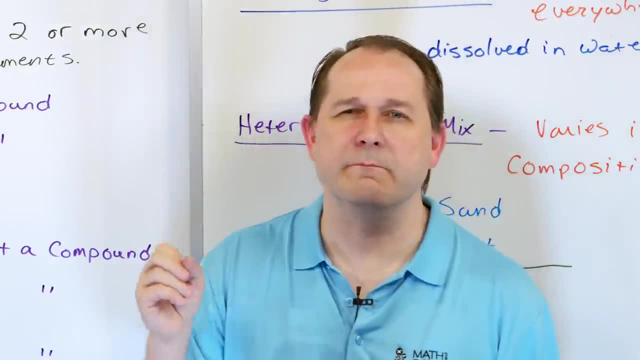 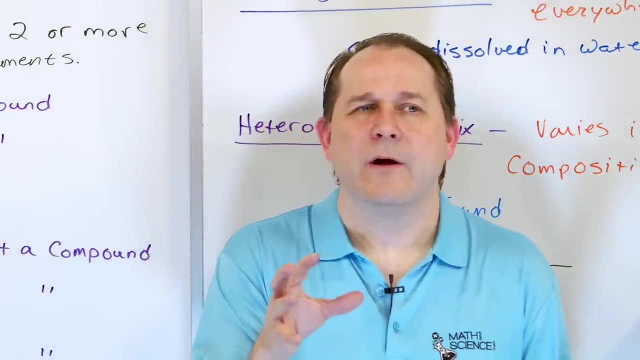 we talked a minute ago- We talked about the electric force- is millions and millions of times stronger than gravity. I keep harping on that because it really governs everything. It governs how they start to share when they gain and lose electrons, and that leads to all the chemistry that 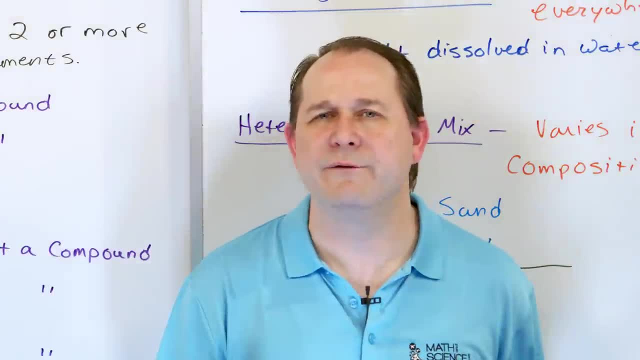 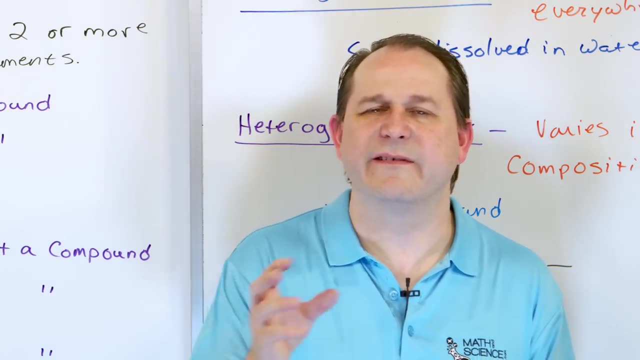 we have. I'm going to give you a little bonus material at the end of this lesson I'm going to. all of the chemistry that we have is all due to electrons moving around on the outer layers of the shells of the atoms that are mixed together. Sometimes they share electrons and sometimes they. 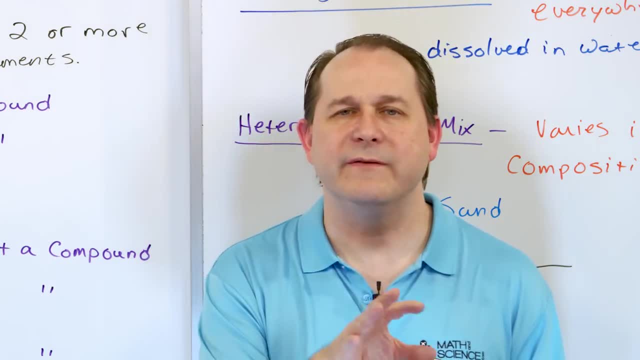 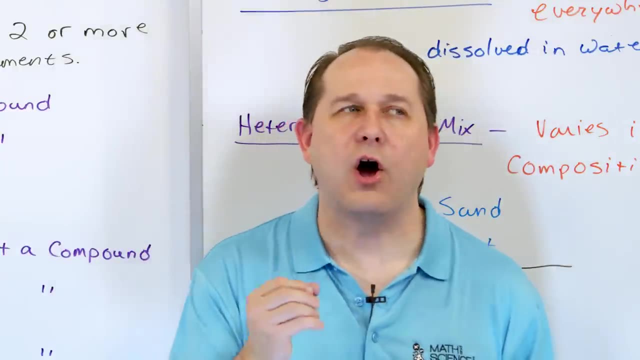 transfer electrons and all of that sharing and transferring comes from the strength of the Coulomb force. It's called the Coulomb force, also called the electric force Because of that, because all of the chemistry that we have is due to that. then all of the chemical bonding is also. 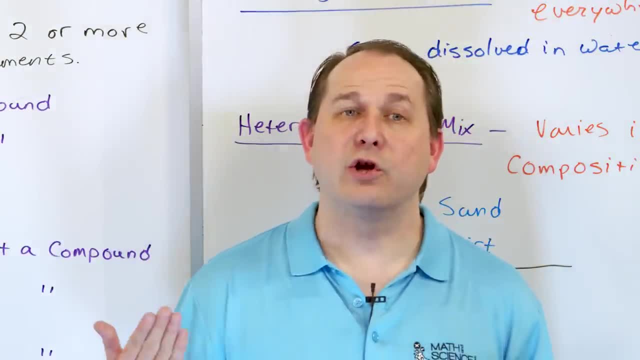 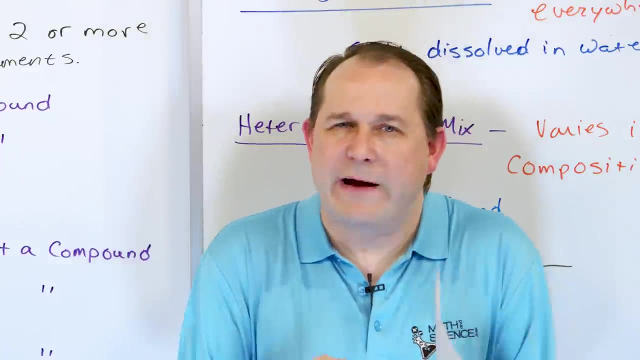 due to the strength of the electric force. We're going to learn about single bonds and we're going to learn about double bonds and we're going to learn about triple bonds and their different strength of bonds: Some bonds, some chemical bonds. 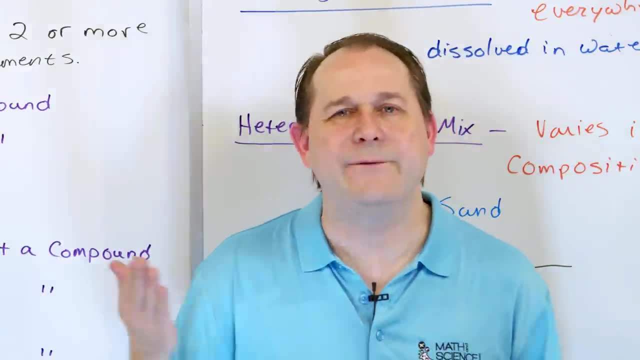 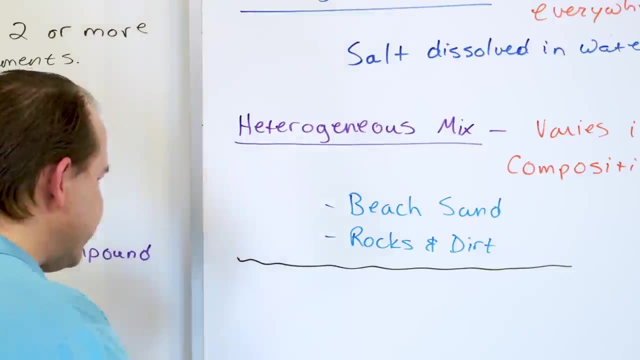 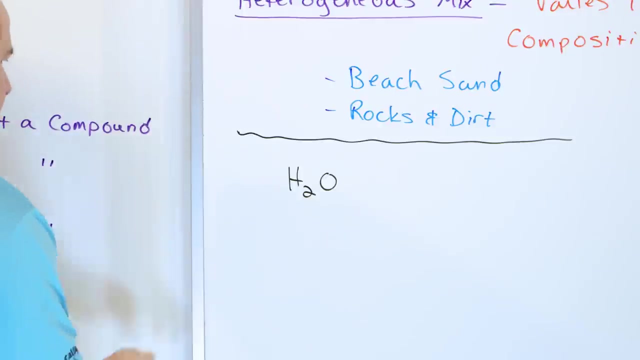 are stronger than others and the strength of the bond. it comes directly from how strong that electric force is. Then I'm going to talk about the most important molecule in our world, which is called H2O. Now, the way we write H2O is two atoms of hydrogen and one. 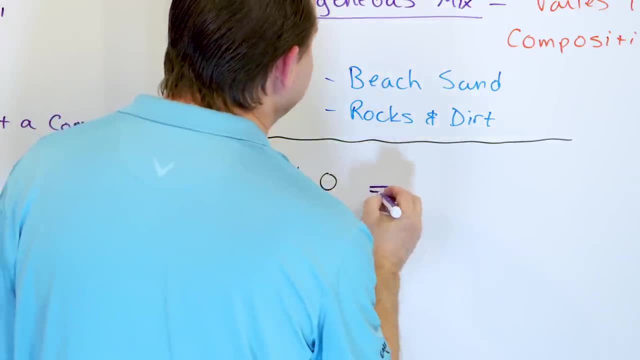 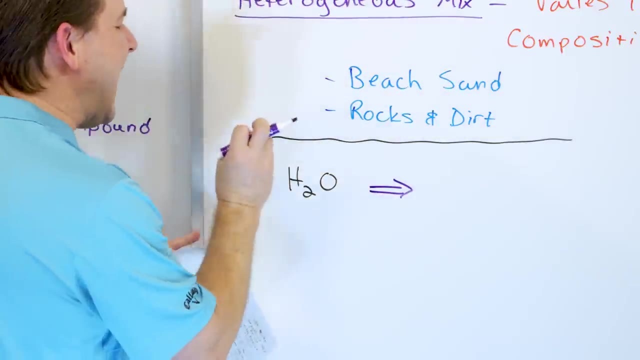 atom of oxygen. Now, later on we're going to get into this a lot more. We're going to have entire chapters on this later. But the way this thing is written is, or the way this thing, if you could zoom in on a microscope and see one atom, you wouldn't see a little letter here: H2 and O. you. 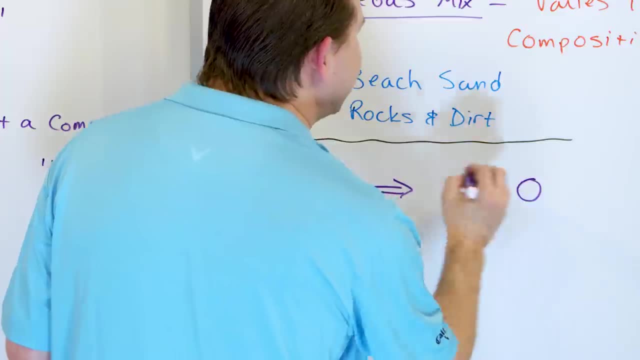 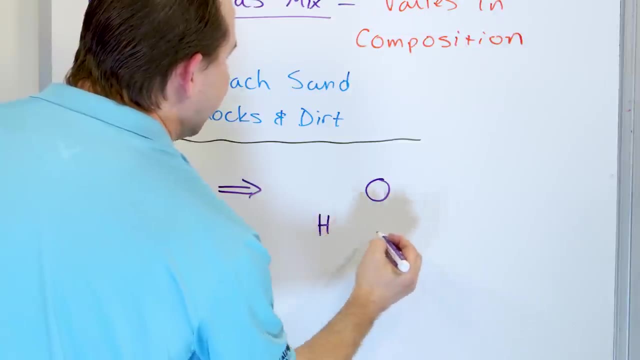 wouldn't see that. You would see something like this. You would see the oxygen atom in the center and these two hydrogens would be off to the side, but it wouldn't be in a line. It turns out that the water molecule is actually bent a little bit, and I'll explain why in just a minute. 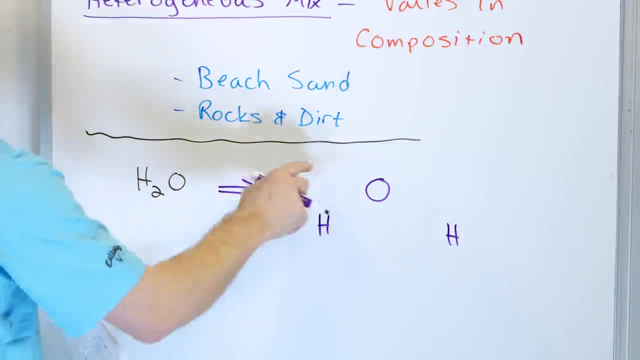 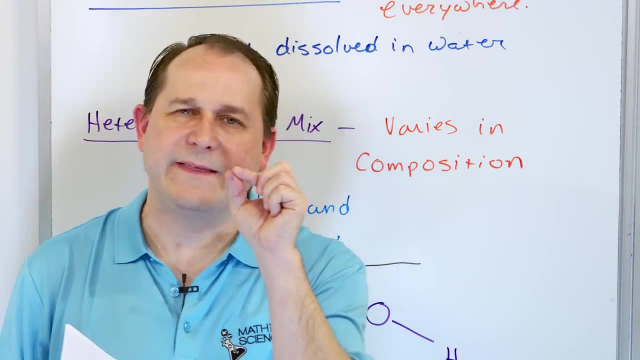 But here are the two atoms of hydrogen and the single atom of oxygen. And this line that joins from here to here, and this line that joins from here to here shows the idea that the oxygen is bonded to the hydrogen. And when we say bonded, 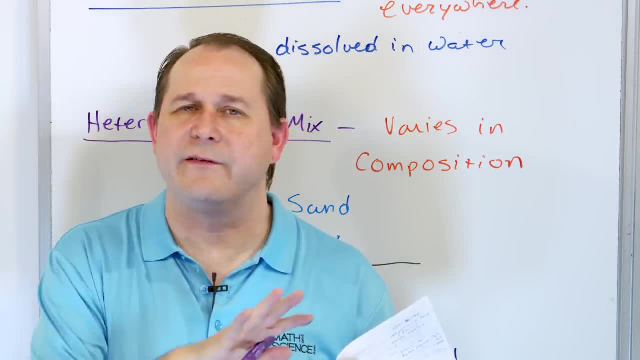 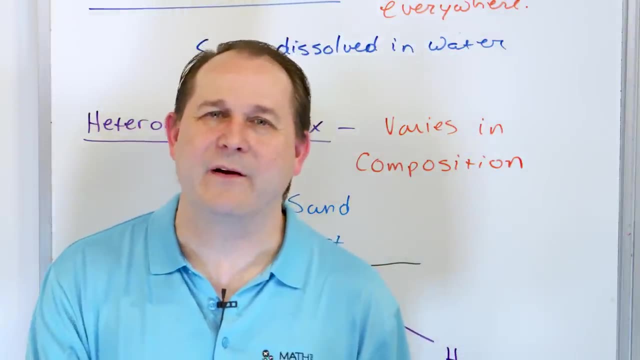 generally it means we're sharing electrons. So there's other situations, we'll talk about it later, but usually we're sharing electrons. You might say: why are they sharing electrons? Well, you can't get too far ahead of me here. okay, We got to go crawl before we walk. The reason they 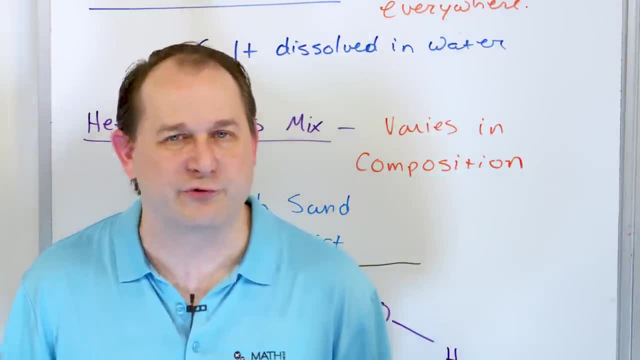 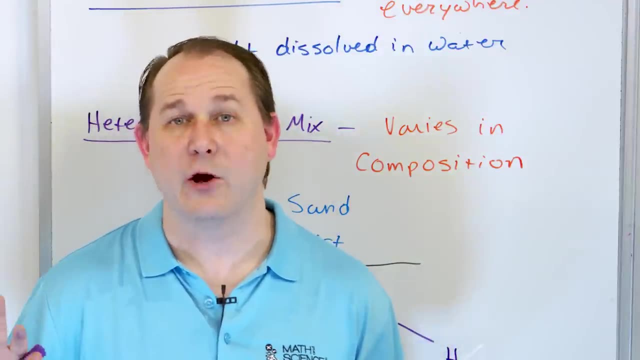 share electrons is all because of that electric force is so strong. Why, If you really get down to it, that's why- And also there's a lot of quantum mechanics which is way beyond the scope of this lesson that gets into why atoms bond with each other. 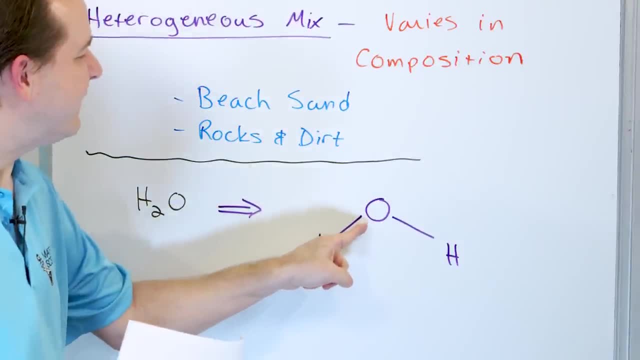 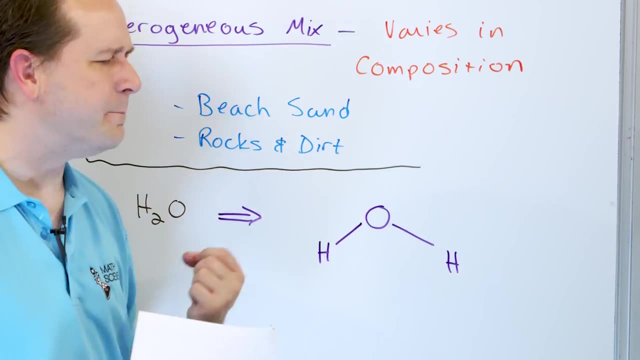 But just for now, we have to crawl before we walk, and these lines are representing a single bond from here to this hydrogen and from here to this oxygen. Now, why is it bent? We're going to talk about why it's bent. We're going to have an entire chapter trying to understand what molecules look. 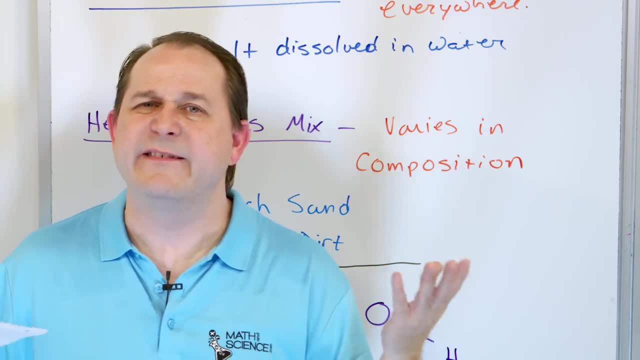 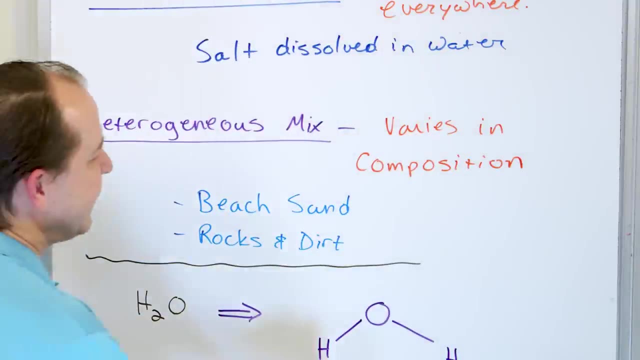 like when we actually draw them out, if we could zoom in and look at them, And some of them have different shapes. and water is a bent molecule, right? The other thing that I want to impress upon you is that not all atoms attract the electrons with the same strength. It turns out that oxygen 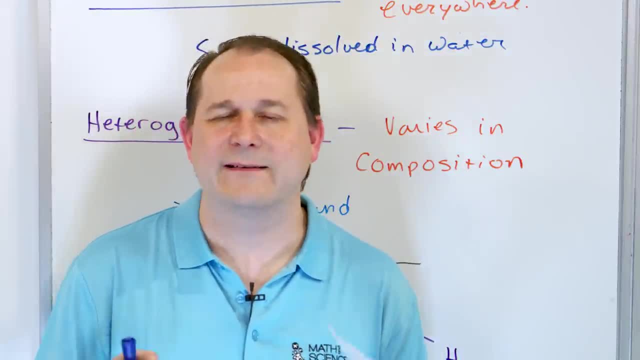 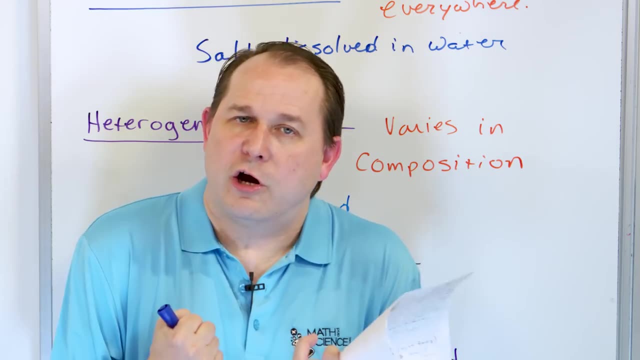 is an electron hog. It loves to attract electrons. And when I say it loves, I don't mean that it has a personality. I mean that the electric force is stronger on the oxygen to pull the electrons closer to it. So because of that, see, this electron is so strong, it's going to attract electrons. 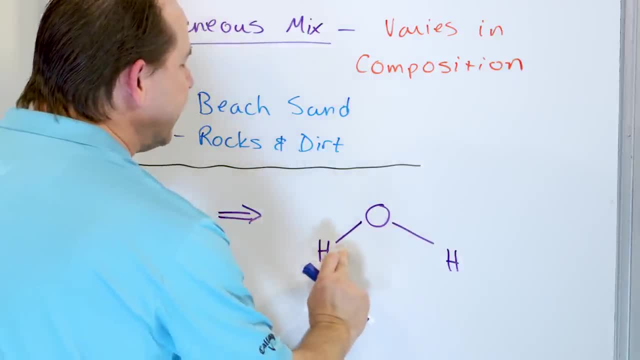 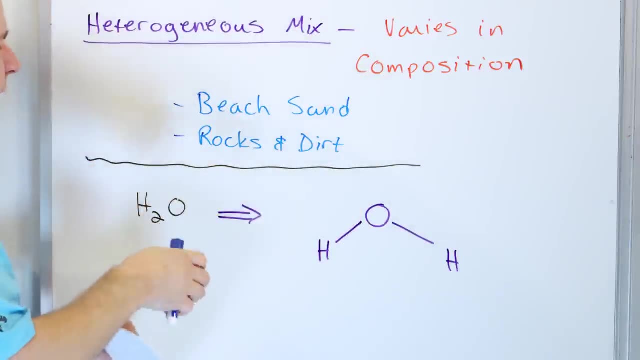 line represents a sharing of the electrons between the hydrogen and the oxygen, and a sharing here between the oxygen and the hydrogen. But since oxygen is so much stronger at pulling the electrons that are here, the shared electrons are not in the middle, They're pulled a little. 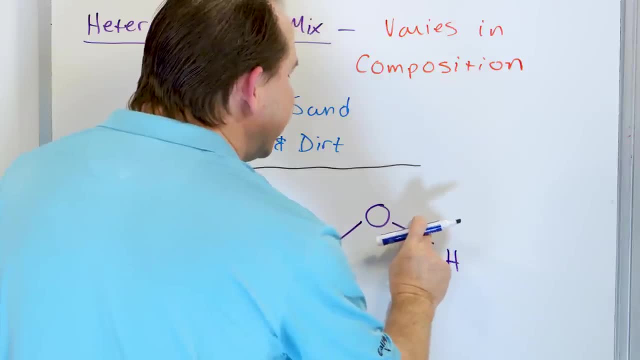 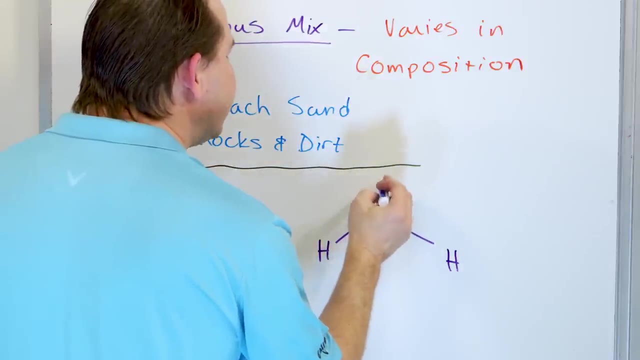 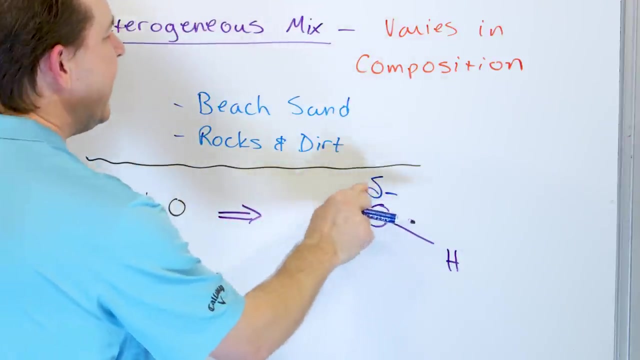 bit closer to the oxygen, These shared electrons. here they're not in the middle, They're pulled a little bit closer to the oxygen. So because of that, the oxygen has a little bit of a slight negative charge. And this little symbol is a Greek letter, delta. It's a delta, And I don't 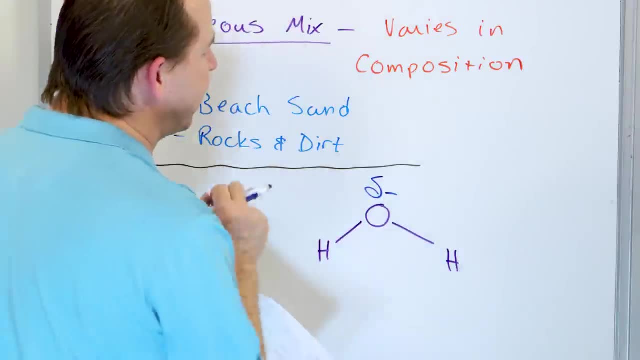 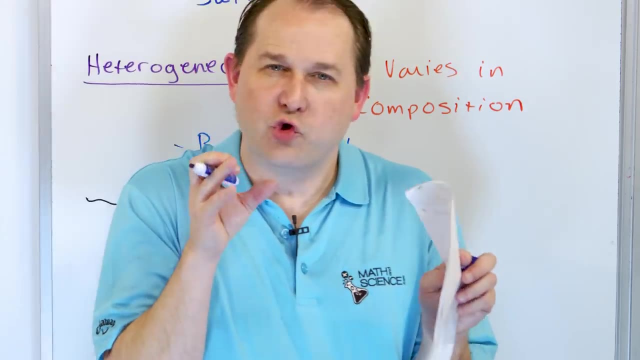 care so much about what symbol you use, I just want you to focus on there. There's a minus sign here And because the electrons are pulled this way, and pulled this way, the oxygen, which normally would have a zero charge, it's pulling the electrons a little bit closer towards it. Why? 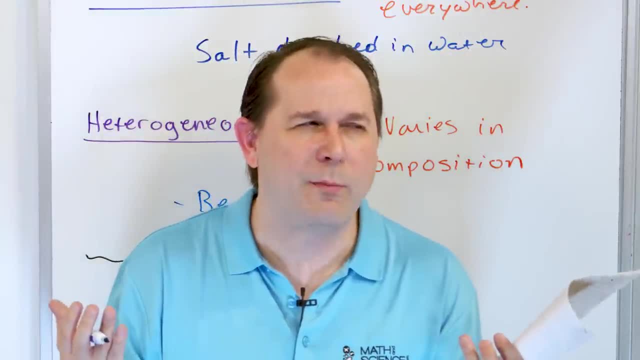 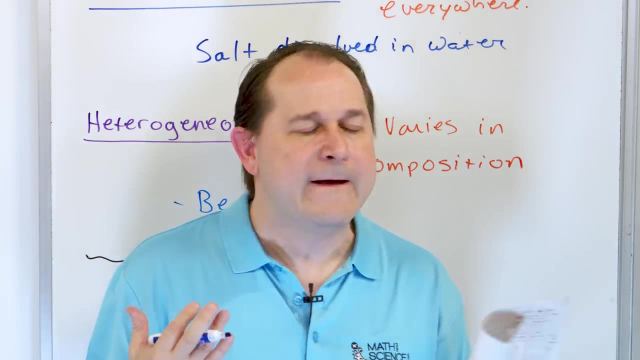 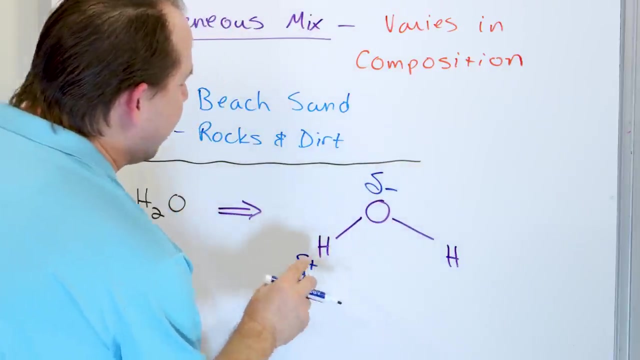 Because of the electric force. If you ever ask why in chemistry it's almost always because of the electric force is so strong And because it's unbalanced and it's unequal in the sharing, then there's a teeny tiny, tiny more negative charge around this oxygen And because of that there's a teeny tiny bit of a positive. 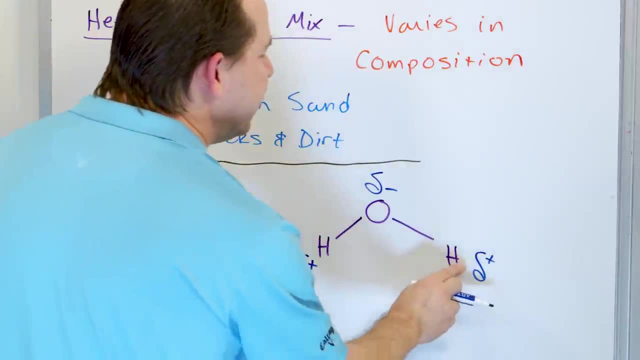 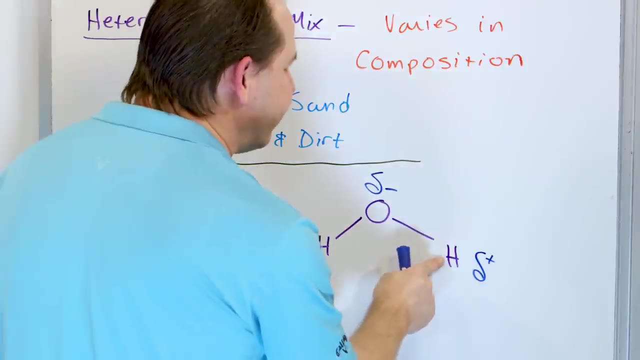 charge around this hydrogen and a teeny tiny bit of a positive charge around that hydrogen, Because, you remember, when these come together, the hydrogen has its own electrons, This hydrogen has its own electron, These oxygen has its own electrons. When they come together, they share. 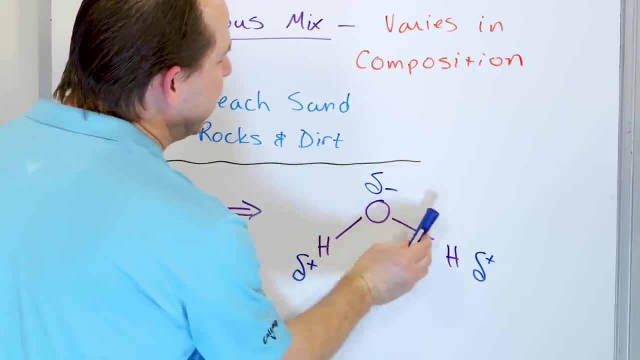 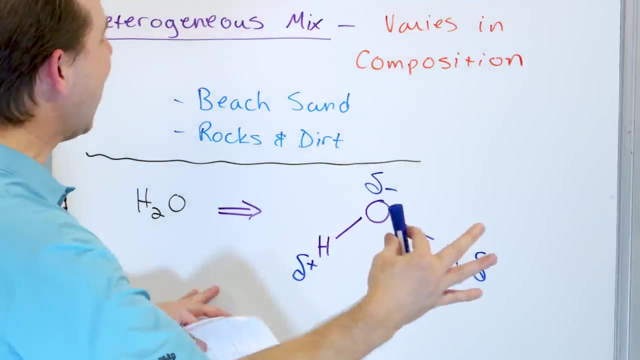 You would think they would share right in the middle. so they're equal. they share between the two. However, oxygen pulls the electrons a little closer and it pulls these electrons a little closer. So if you zoom out and look at it, it appears that the oxygen has a. 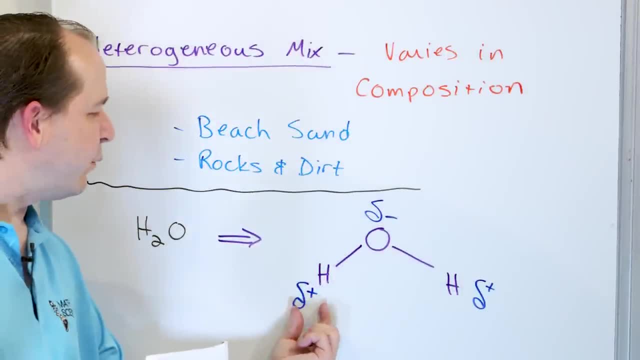 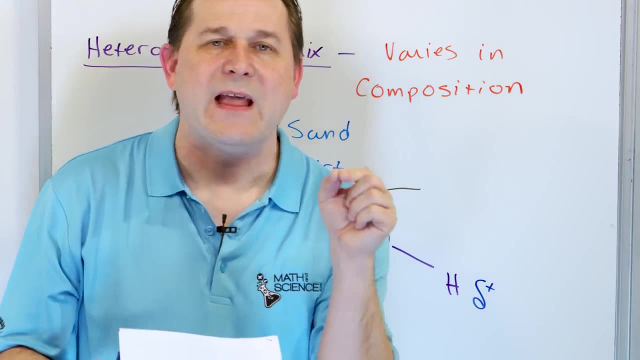 slightly more negative charge than these hydrogens, which have a slightly more positive charge. So don't worry about the Greek symbol, Focus on that. the hydrogens are very slightly positive and the oxygens are very slightly negative, So normally we don't talk about this for about. 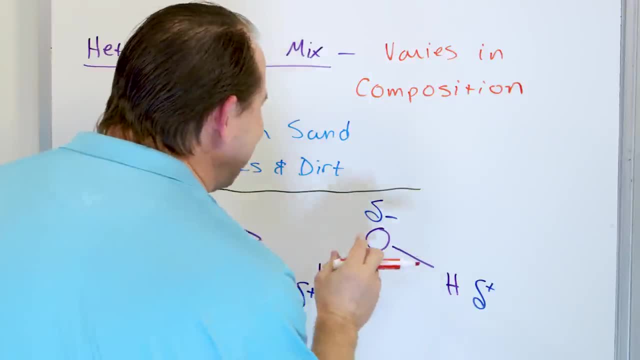 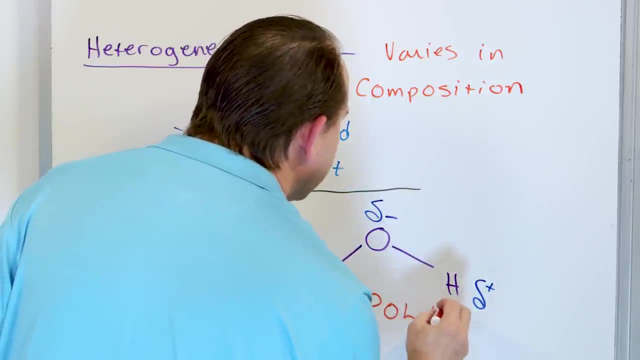 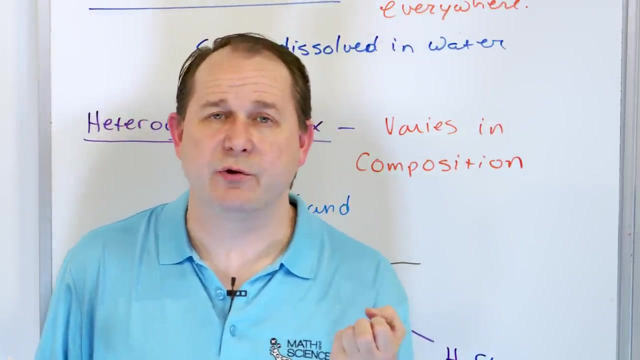 five chapters in the chemistry, or six or seven chapters, This idea that the oxygen is a little more negative and the hydrogen is a little more positive. this is called polar. This means water is polar. Polar just means that one side of the molecule 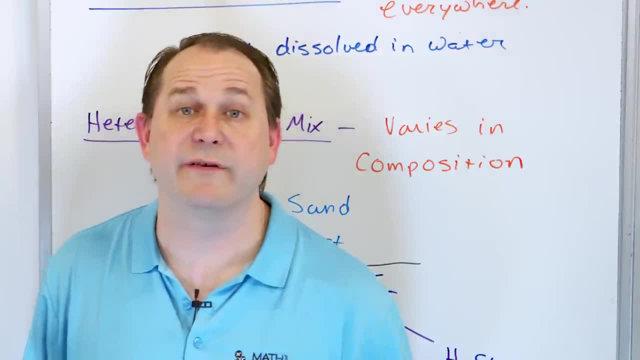 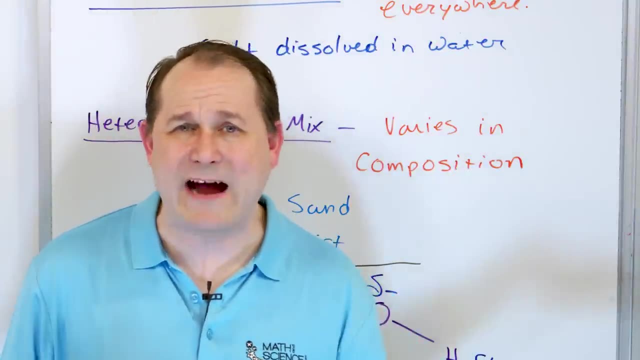 is a slightly negative charge and the other side of the molecule is a slightly positive charge. Now, why did I tell you this? Because this is just an introduction. I don't have to tell you this now. We're going to have an entire chapter talking about this, right? Why? Well, it's incredibly. 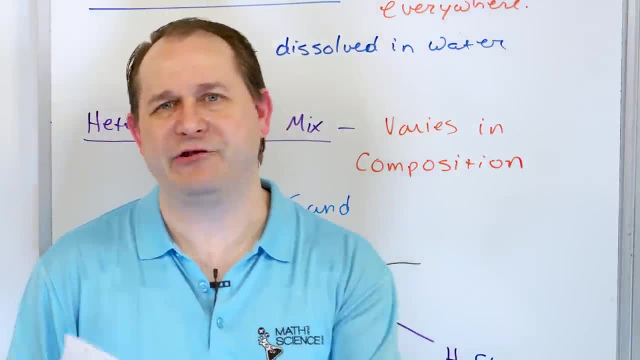 important that water is a slightly positive charge. It's incredibly important that water is a slightly positive charge. It's polar. I'm trying to give you motivation. more than anything, I'm trying to get you excited. I'm trying to get you to be like: wow, that's neat, I didn't know that. Well, all the water you drink, 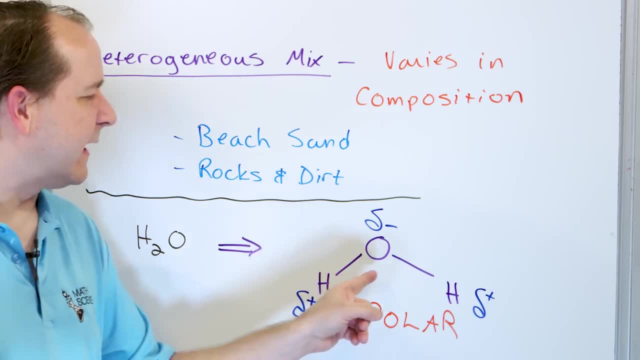 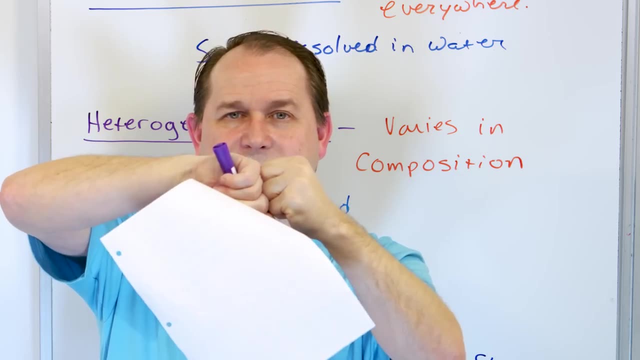 is very slightly negative on the oxygen and very slightly positive on the hydrogen. Now, why do we care about that? Well, because if I put salt in the water, the salt is also bonded together and it falls into the water. But you see, since part of the water is negative and part of 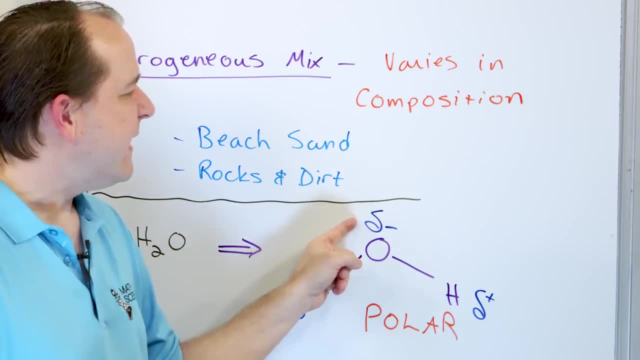 the water is positive, this negative side is going to attract the sodium out of the water. So if I put salt in the water, the salt is also bonded together and it falls into the water. So if I put salt in the water, the salt is also bonded together and it falls into the water. 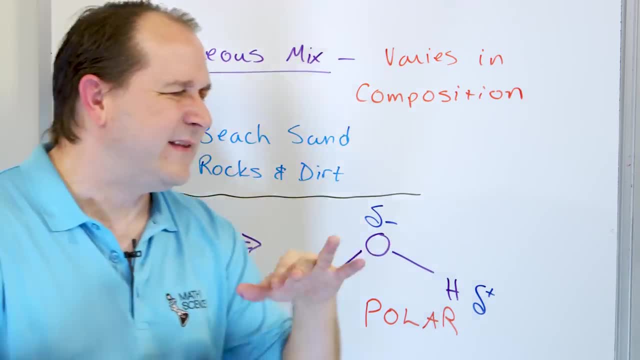 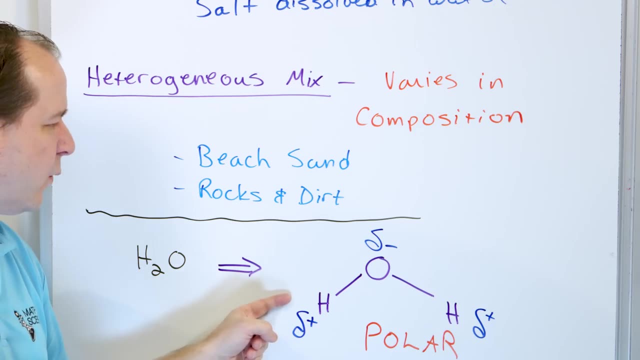 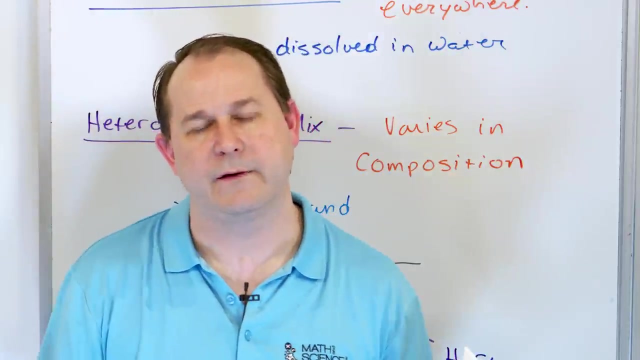 The details don't matter, but one side of the oxygen is going to attract one side of the salt and the other side of the hydrogen side of the water is going to attract the other side of the salt, the sodium chloride, and it's going to pull the sodium chloride apart. What do you think that? 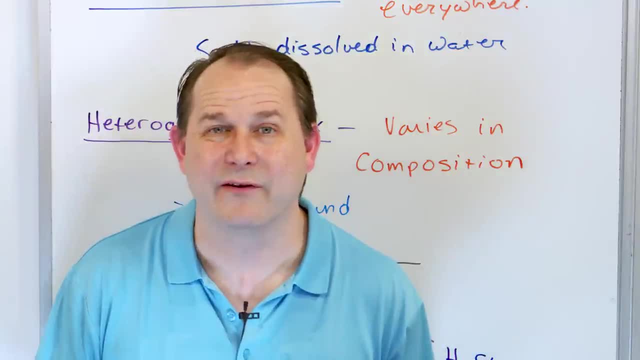 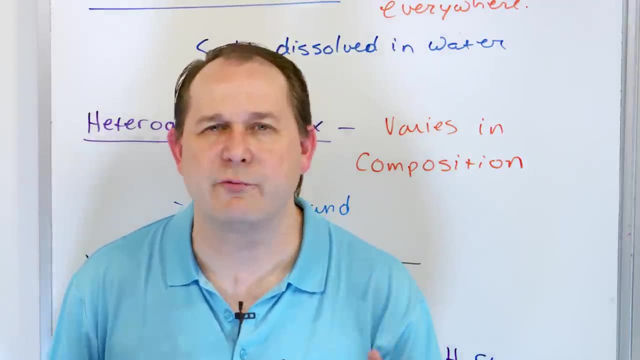 means when sodium chloride gets pulled apart, It means it dissolves. So when you pour salt in a glass, I want you to start thinking microscopically. what's happened? It's trillions and trillions and trillions of water. 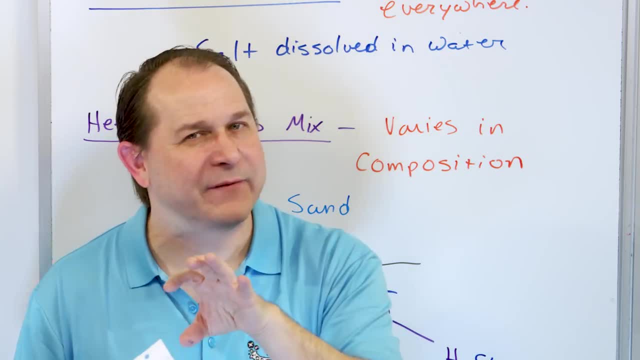 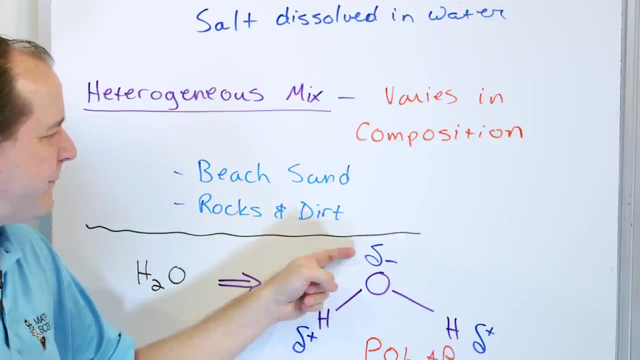 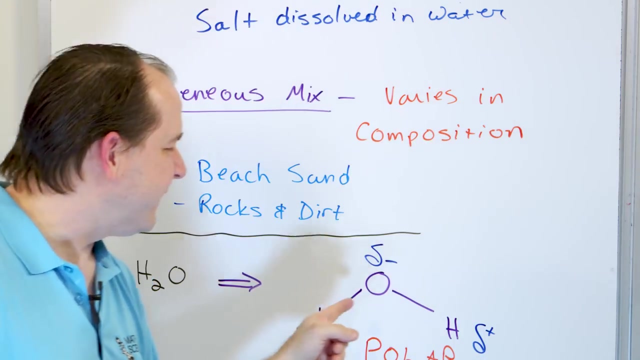 molecules, which, one half of which are positive and the other half is negative, and all together it allows you, because the electric force is so strong, this tiny little charge imbalance on the oxygen, this slightly negative can attract the positive part of this, of the sodium chloride salt, and this tiny little positive charge on the hydrogen can attract the very slightly negative. 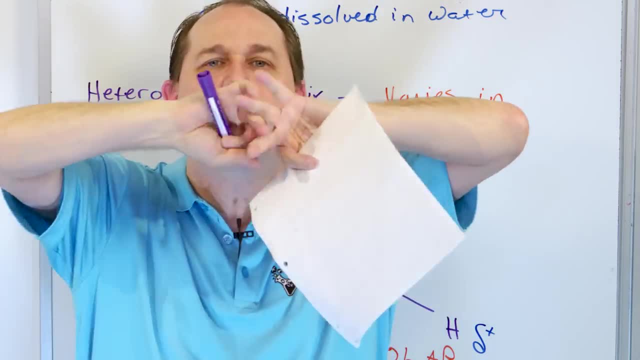 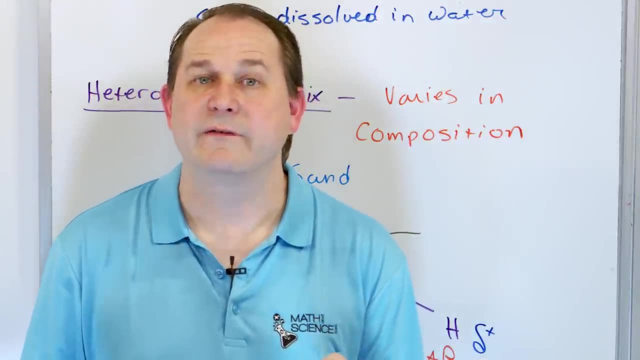 side of the salt and because they're pulling on different ends of the salt. they pull the salt apart and they dissolve it. if you put sugar in, it dissolves the sugar and water turns out to be able to dissolve a lot of different things. why am i bringing this up? because your body is mostly 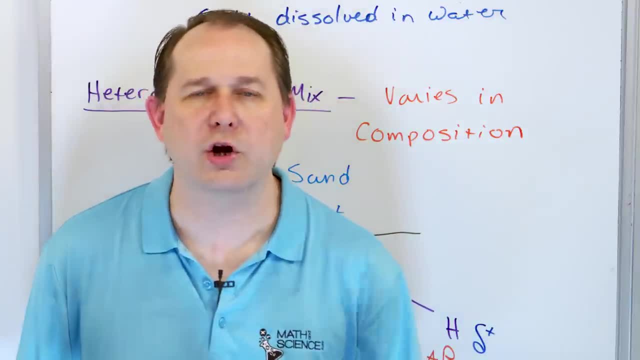 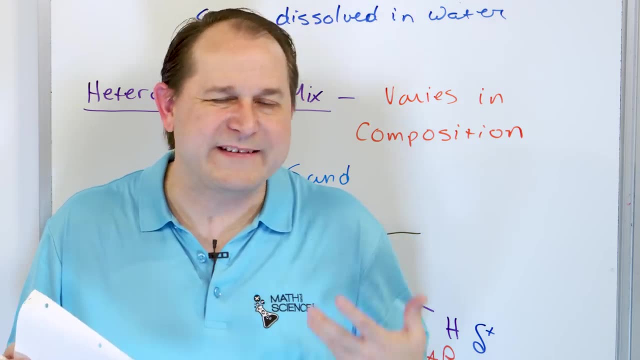 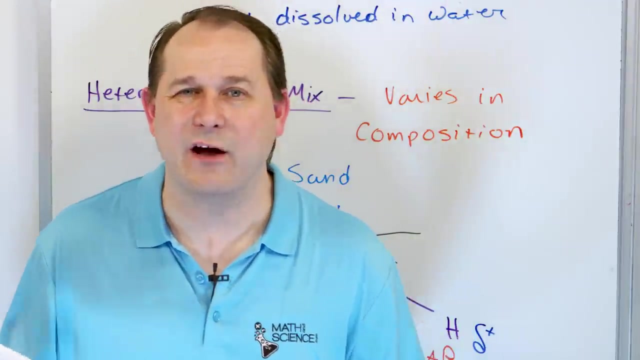 water. all the chemistry in your body relies on water. why? because all of the things that are happening, that are important, are dissolved in water. yourself, all the cells of your body, they're basically chemistry, little bags of chemistry happening inside of water. and if water did not dissolve things, 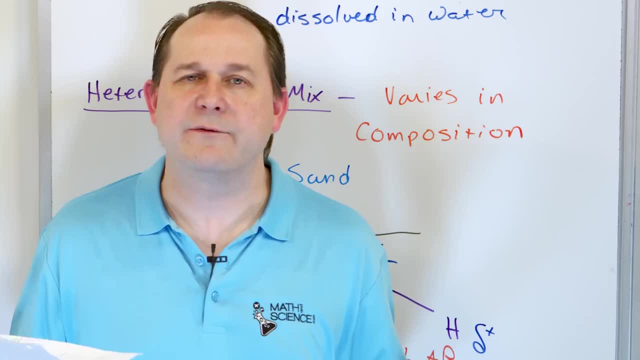 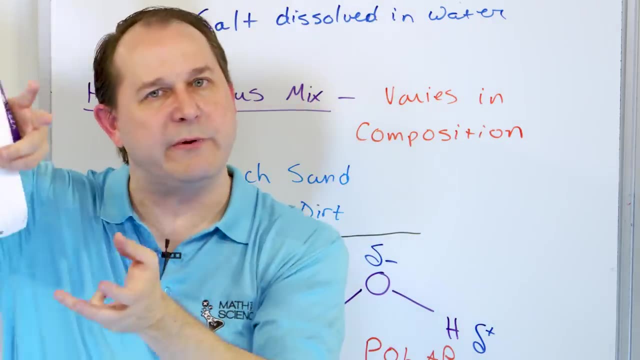 then you wouldn't be able to have liquid chemistry inside of your body. nothing would work, because when you have things floating around in a liquid, they can bump into each other and they can have chemistry with each other. when you have salt poured into water and it dissolves the salt, you 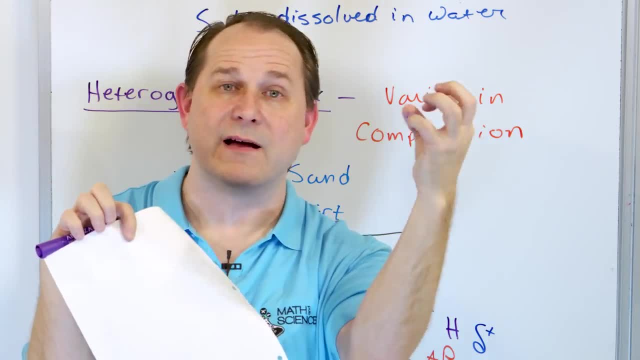 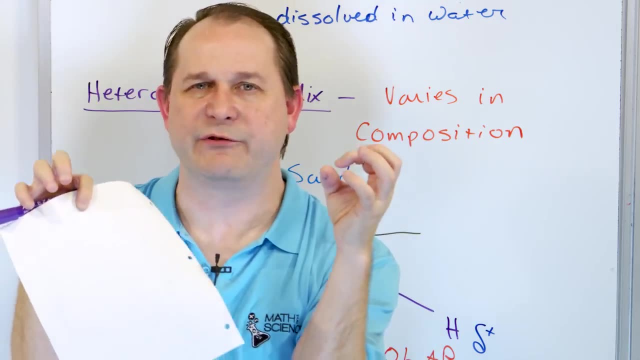 have the salt broken apart, literally broken up into a sodium and a chlorine, sodium and a chlorine. we'll talk about ions later. but it pulls them into ions which are just basically breaking them in half. but they're, they're charged now and they're just breaking them in half and they're just 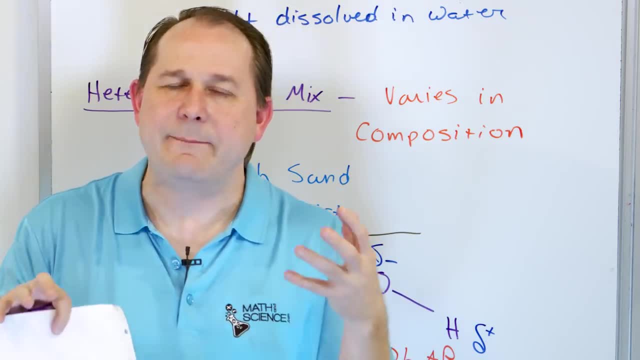 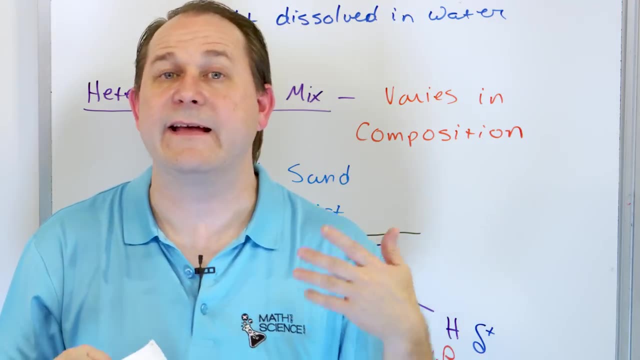 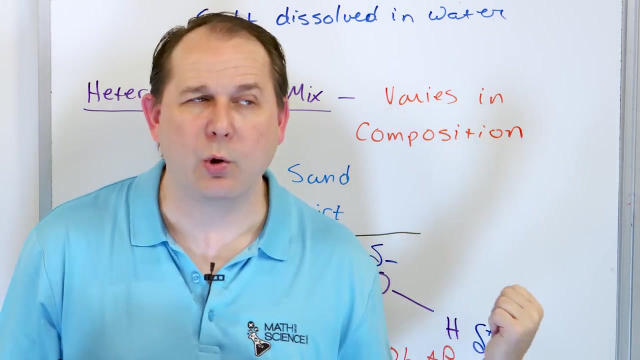 floating around in the water, but in your body that means everything can be floating around and it allows chemistry to happen, because when things are floating around they can bump in to other species and they can have chemical reactions. so if the electric force wasn't that strong, then water would not be a polar molecule, which means it wouldn't have a positive and a 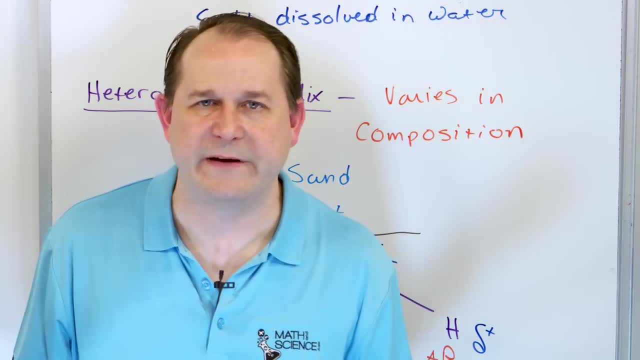 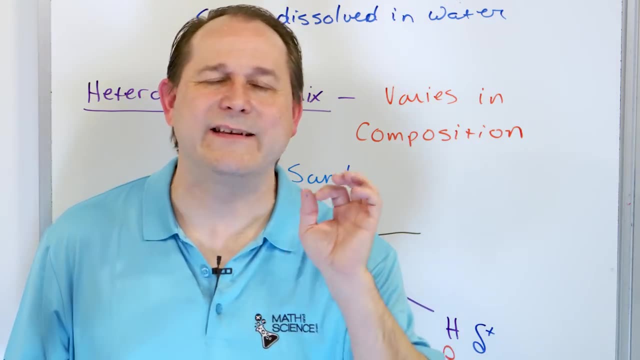 negative side, and if that didn't happen, then water wouldn't dissolve anything and if that didn't happen, you wouldn't have chemistry for your body. and it also means ice wouldn't float, because ice also floats because of this charge imbalance and i'll talk about that later, but it 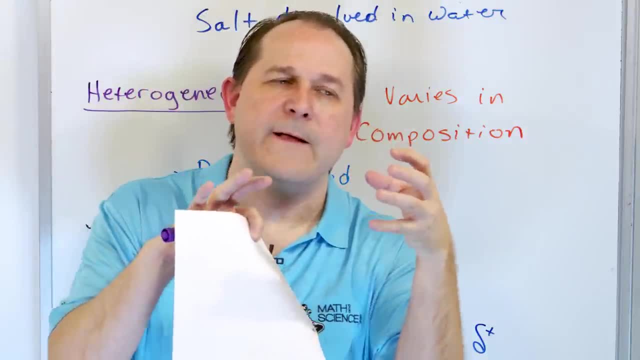 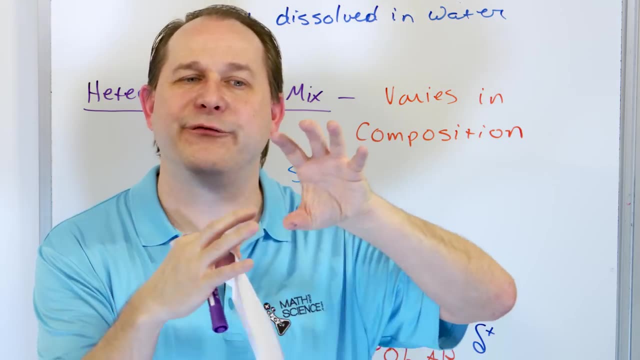 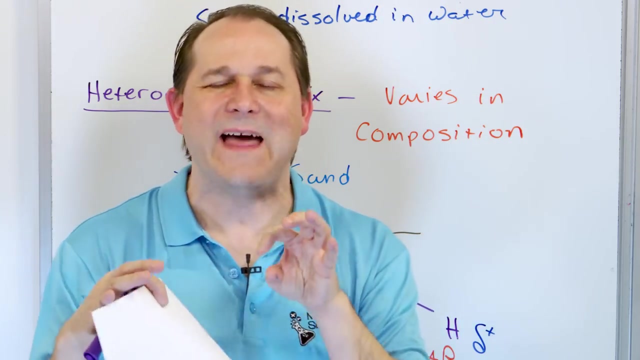 has to do with when you cool down, water it. it has to do with these charges on the hydrogens and the oxygens. they are what causes ice to form the structure that ice forms. it causes them to join up in a certain way to form the structure of the ice crystal, and that joining is what causes ice. 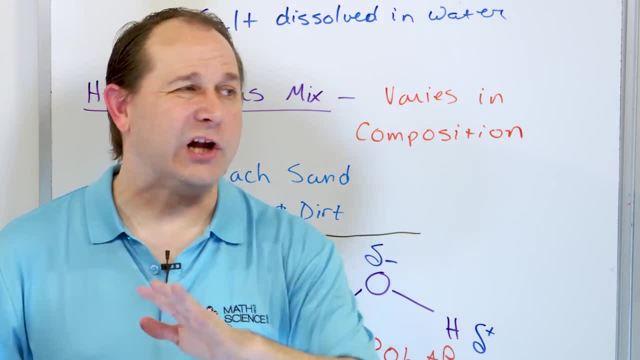 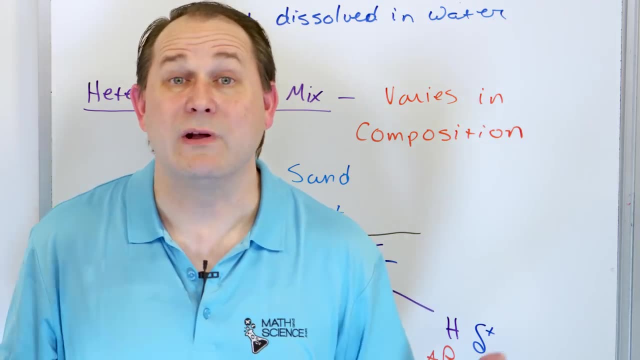 to float, and if ice didn't float, then long time ago all of the oceanic gases would have been dissolved and the oceans would have just froze over from the bottom up and there'd be no fishes and no, you know, no, no life on earth. so i guess i'm just trying to give you a little bit of motivation. 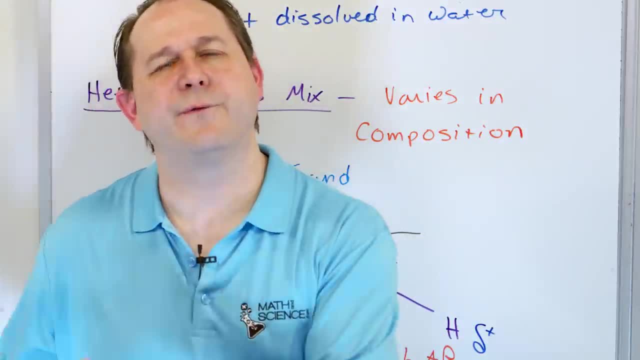 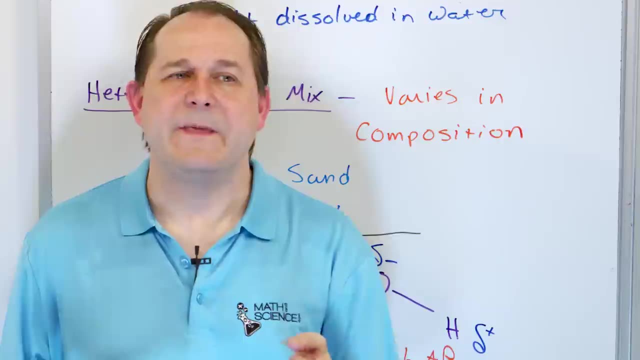 that something as simple as: oh, i tell you, the electric force is so incredibly strong. believe me, it's strong and you're like, okay, i get it. but now i'm trying to give you a practical thing. if it wasn't that strong, then water would not have this charge imbalance, it wouldn't be polar. 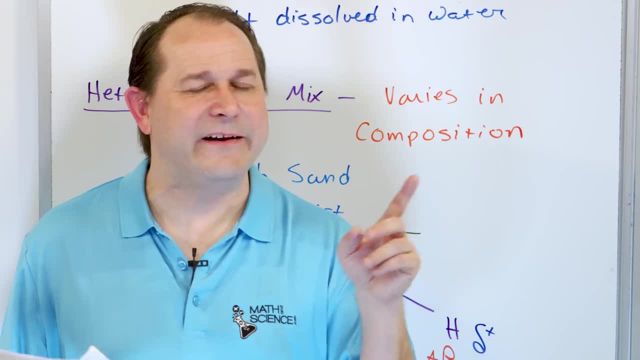 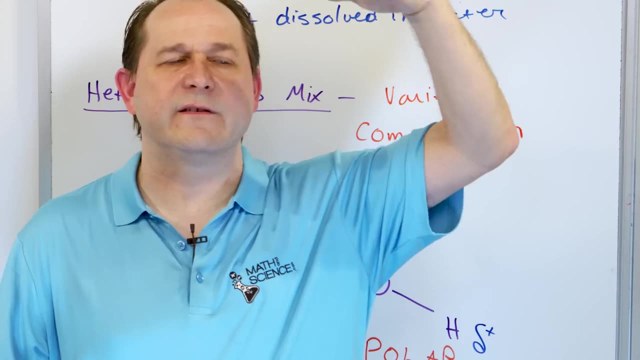 and if it wasn't polar, nothing would dissolve and ice wouldn't float. and that means we wouldn't have the oceans, because ice would be frozen solid Because ice floats. it means when ice floats to the top you could still have fish swimming on the bottom. But if the oceans froze from the bottom, 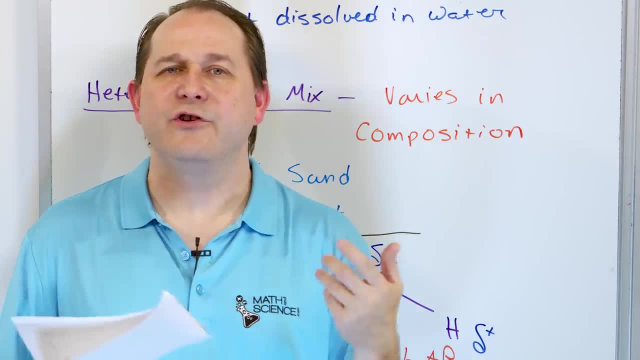 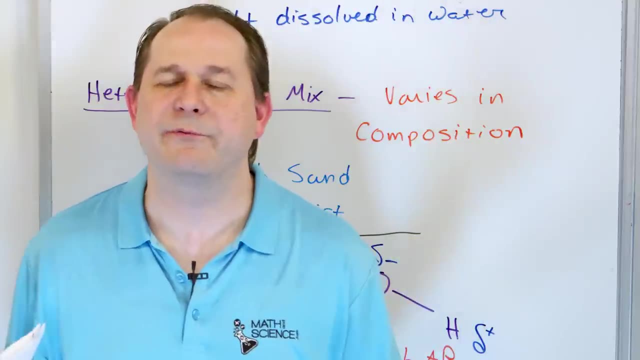 then the whole thing just gets frozen solid, right, And you would never have any complex chemistry happening in a liquid vessel, which is what your body is doing all the time. So you wouldn't have any respiration, you couldn't have any metabolism and you wouldn't have any life. 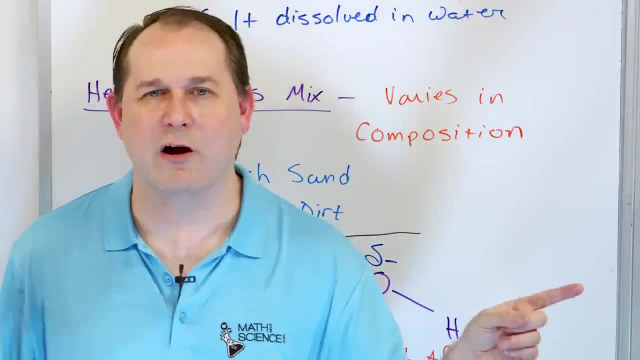 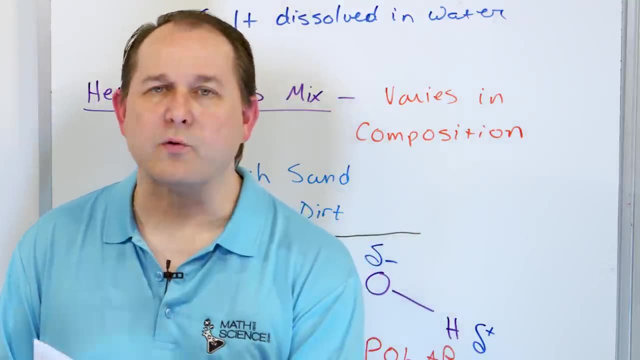 So everything literally comes back to how strong that electric force is. It's millions of times stronger than gravity. All right, I've done enough talking. I want to wrap this up. The last part of what I'm going to leave you with is a roadmap for what we're going to study in the 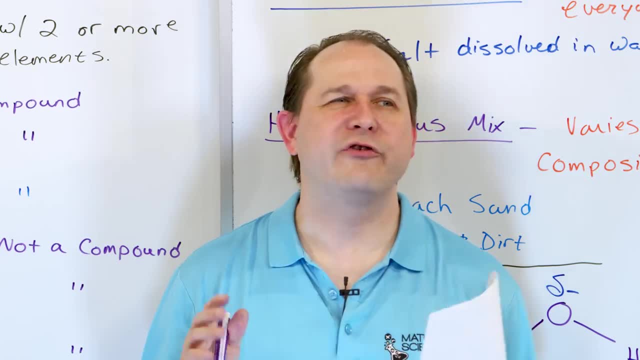 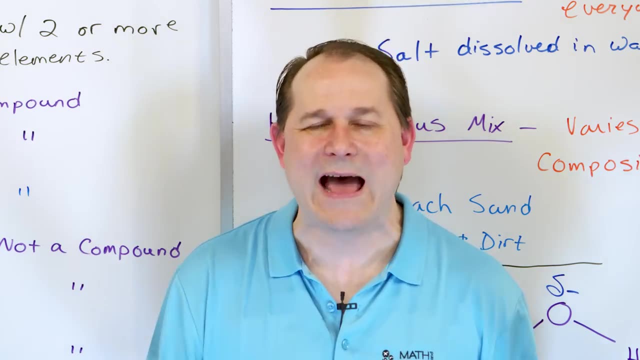 future. We're going to study chemical compounds in detail. We're going to talk about when they combine, how they combine and how do we name them, What do we call them And how to determine what happens when we have two things coming together. Then we're going to talk about chemical 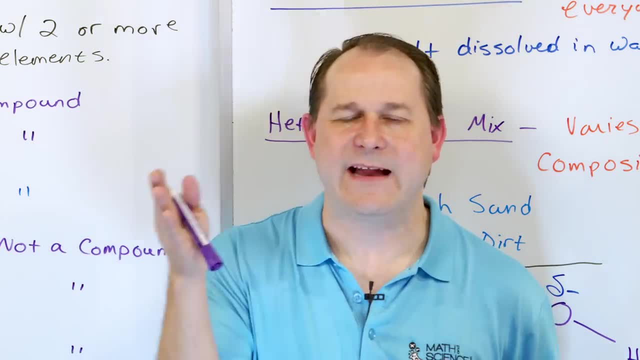 reactions. When does a chemical reaction happen, Why does it happen, And what forms on the other end of the spectrum And what forms on the other end of the spectrum And what forms on the other end of the chemical reaction. And then we're going to calculate. okay, if I mix so many grams, 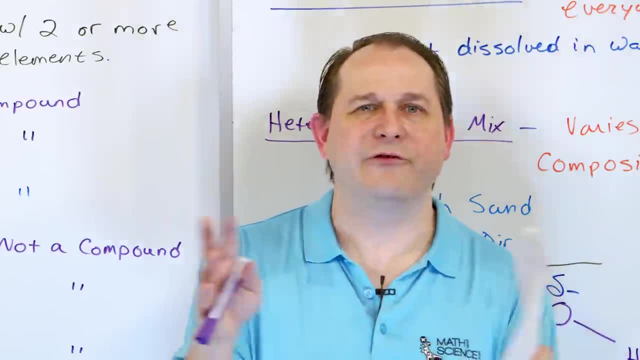 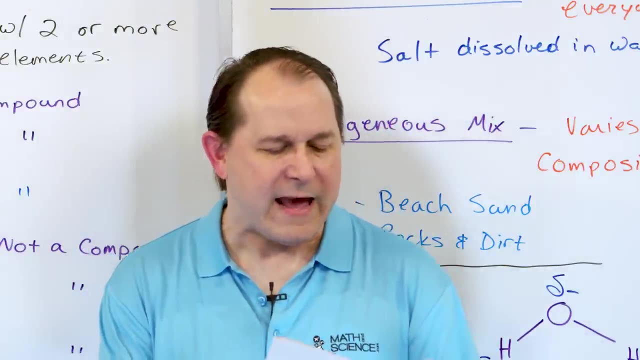 of reactants together. that's the things you mix in the test tube. how much grams of product am I going to get? Will it be solid, liquid or gas that comes out the other end, And how many grams of it will I have right? And then we're going to talk about how much heat comes out of that. 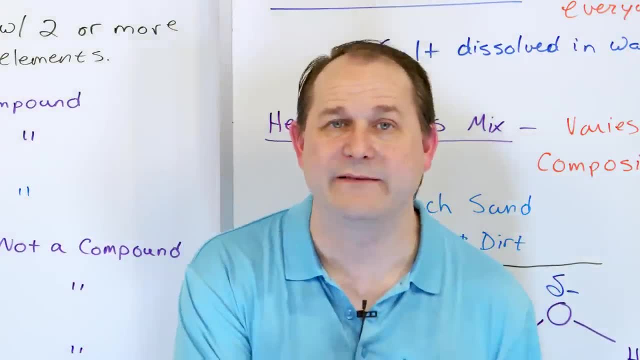 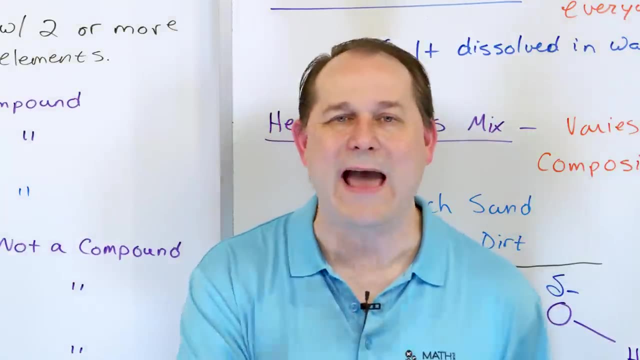 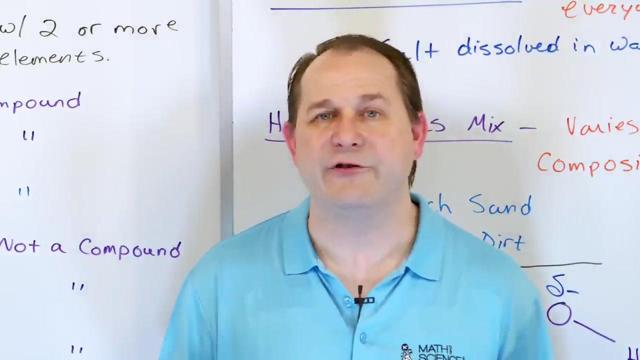 chemical reaction, Or sometimes chemical reactions require heat to get started, Like when you burn the log. nothing happens until you add heat. Some reactions don't happen unless you add heat to get it started. Some reactions are very, they liberate a lot of heat, like rocket engines for instance. 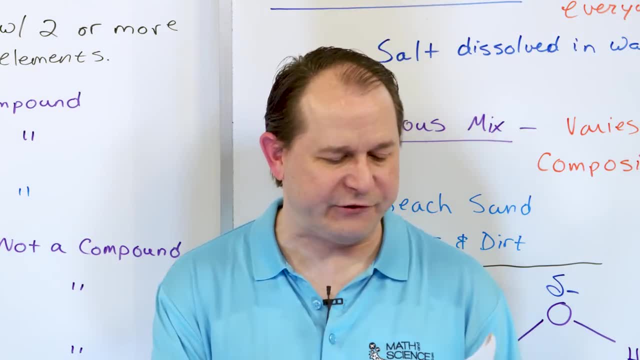 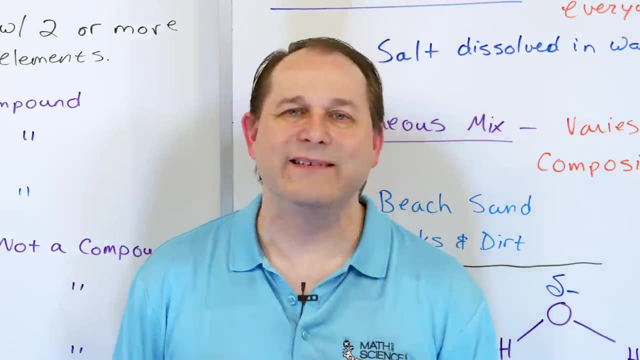 They liberate a lot of heat. So how much heat comes out of a chemical reaction? What is heat? by the way, It's a microscopic motion of atoms. So we're going to talk a lot about what heat is and temperature. Is light released? We're going to talk about what causes light to come out of a 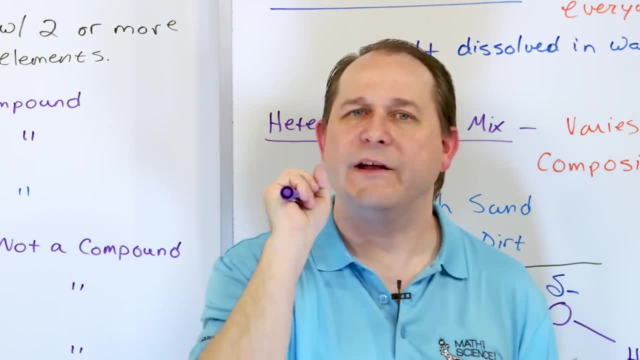 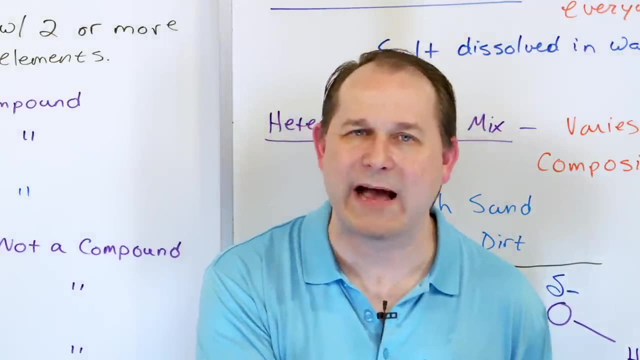 fire. It's the electrons jumping around inside of the atom and they generate a photon of energy which we call light that comes out of that. So a campfire is heat and light. It's a chemical reaction, also with electrons moving so we can see. 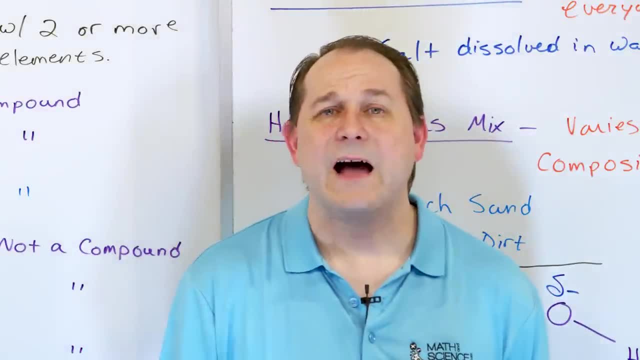 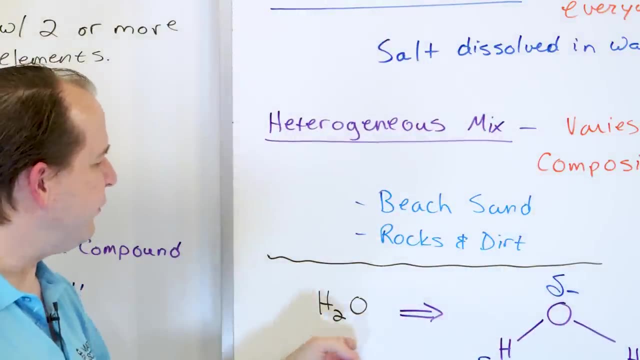 the light that comes out. Then we're going to talk a lot about the structure of molecules. So you can write these things down, like H2O and CH4 and other things. You can just write them down with letters and numbers, but it doesn't tell you the structure, It doesn't tell you the shape. 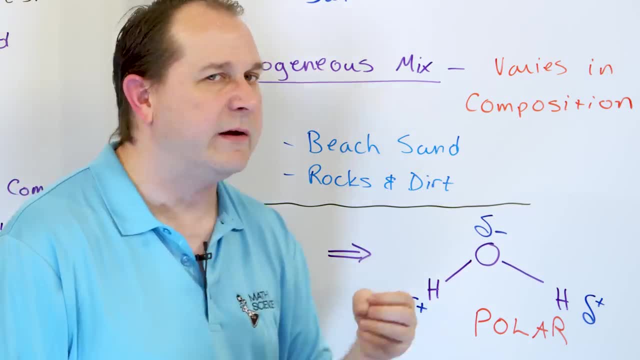 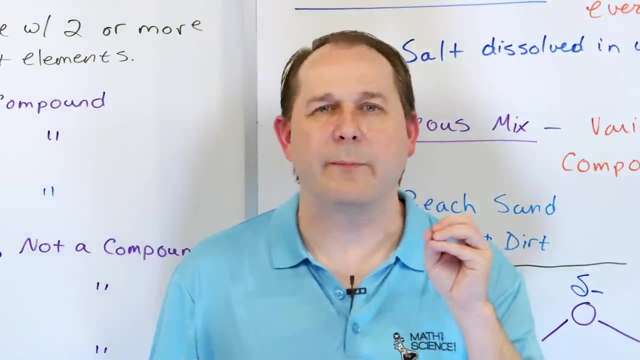 Why is water bent like this? It's not a straight line. It doesn't make sense. Well, it actually does make sense, but we have to dive into the details of what's happening. So we have to talk about electric structure. We have to talk about electronic structure. 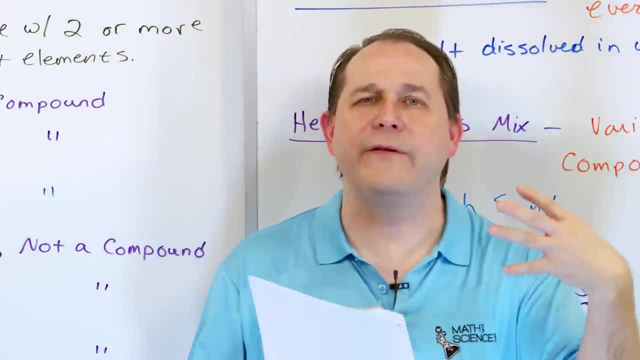 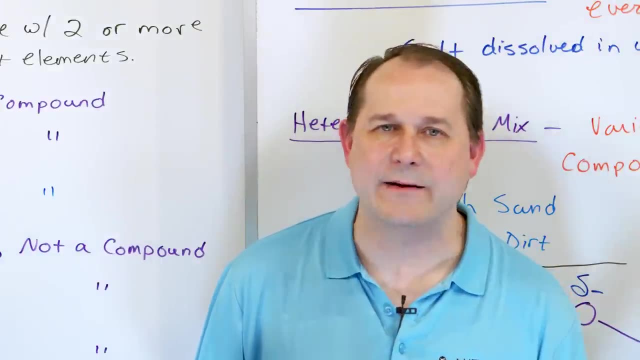 around every one of these atoms? How are the electrons organized around the atom and how do they interplay when two things come together? So we have to talk a lot about atoms and a lot about a little bit of quantum mechanics to understand how the electrons are structured. 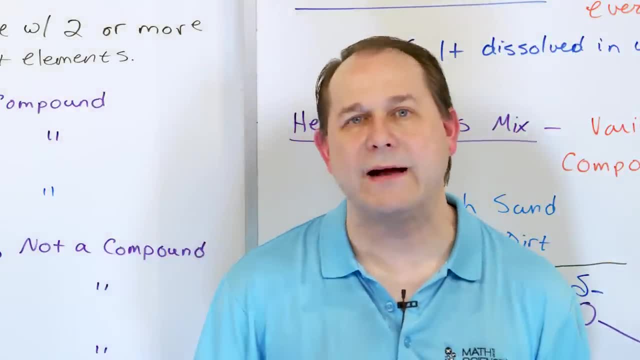 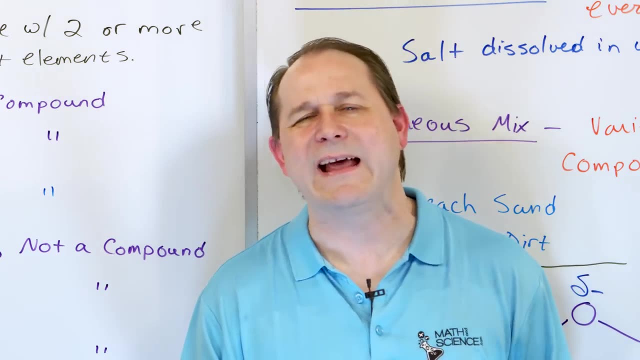 around atoms and how they come together. We're going to talk about the chemical bonds next: single bond, double bond, triple bond and then all other flavors of bond called sigma bond and pi bonds. How are the electrons coming together to make a bond and what is a bond? 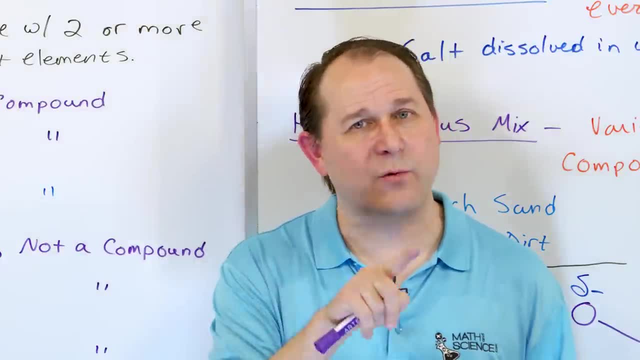 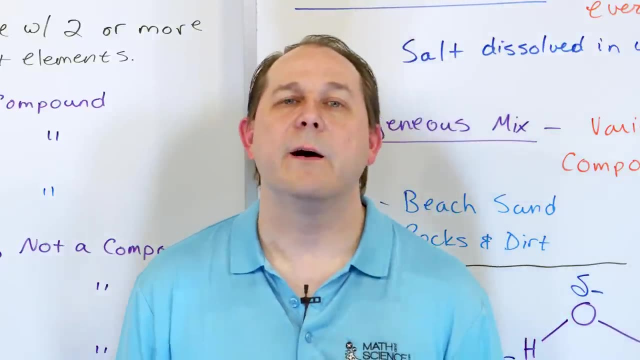 and why do bonds happen anyway? Because, believe me, that question is not as easy to answer as you might think. We're still studying exactly how bonds happen, right? Then we're going to talk about reaction rates. How fast does a reaction happen? How far will it go? How much heat is? 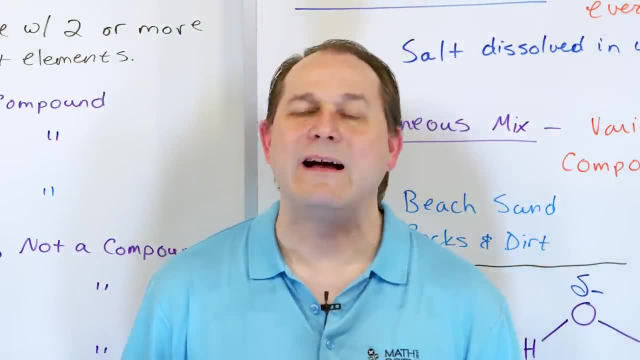 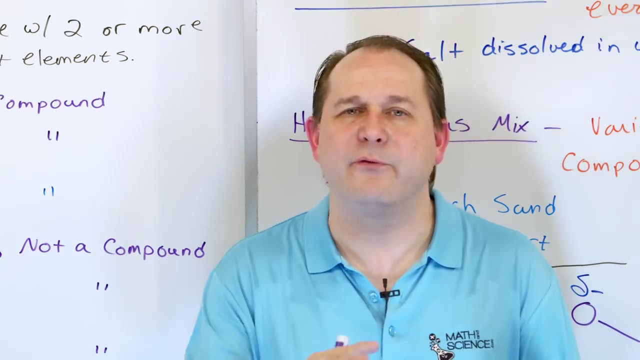 released and how fast will it happen? And then we're going to talk about gas laws- solid, liquid- and then we have the gas phase where we're going to have, you know, when you compress a gas, what happens when a gas expands? What kind of chemistry can you have with? 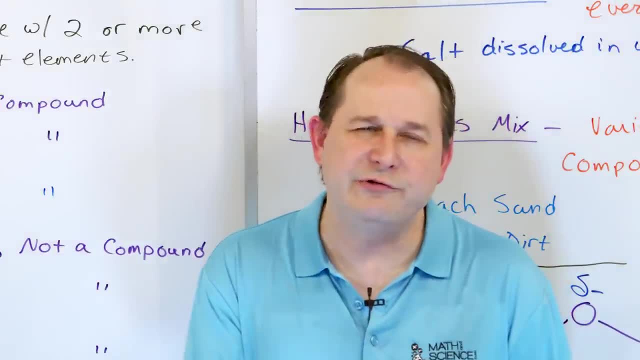 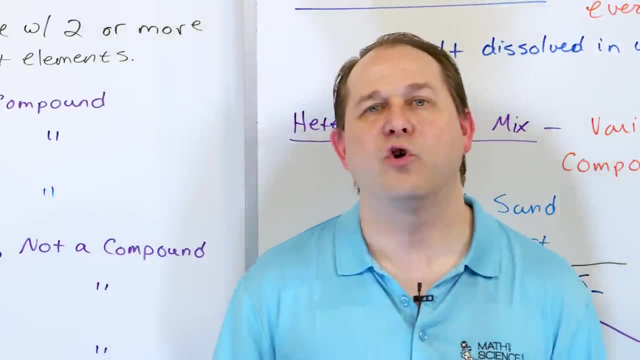 gases, if any right. And then we're going to talk quite a bit about solutions and intermolecular forces between the atoms and solutions, and then, at the very end, we're going to talk a lot about quantum chemistry. In fact, you can go beyond this chemistry class to study an entire career. 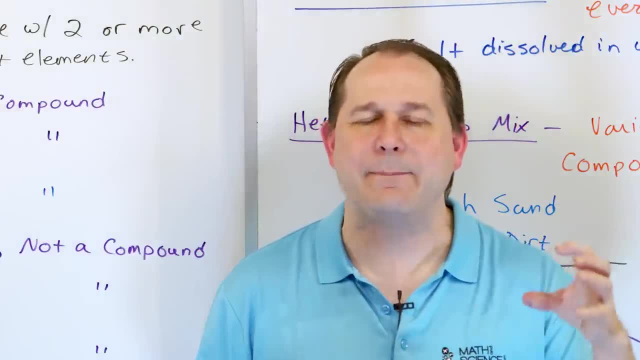 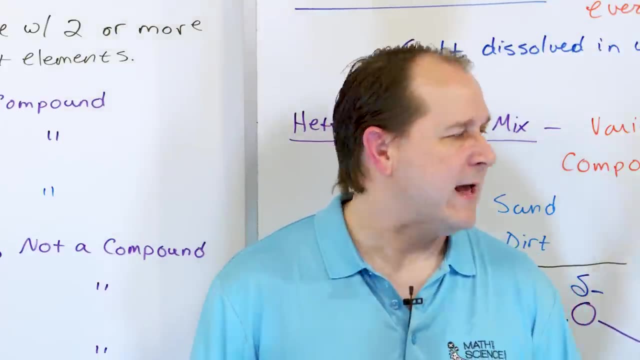 in quantum chemistry, and that's all about what is happening around that atom. Why do the electrons behave the way they do? What is an electron, Anyway? and let me clue you in, an electron is not what I drew on the board. You see a teacher. 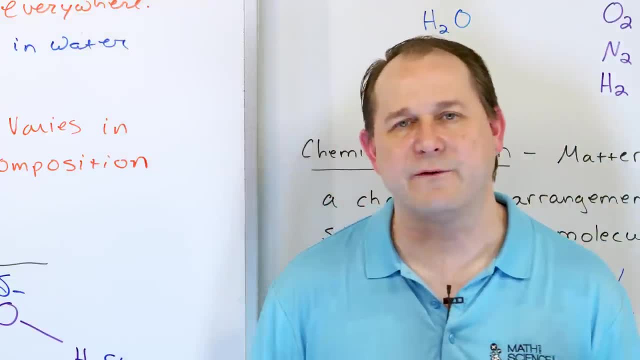 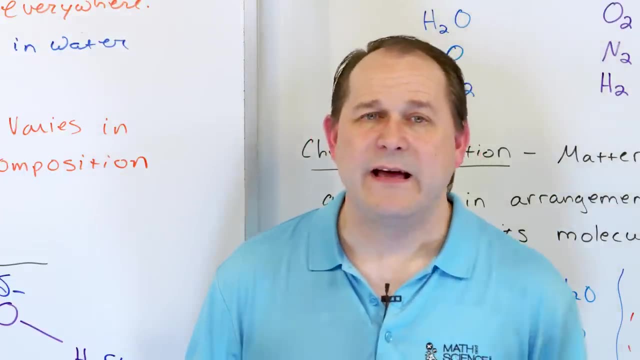 told me a long time ago my favorite teacher I've ever had in my life in university. he told me education was a series of lies And it took me a while to understand what he meant. but what he meant is that I have to lie to you a little bit in the beginning so that you can understand something. 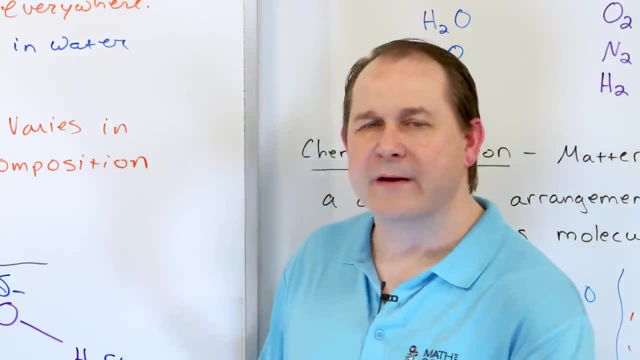 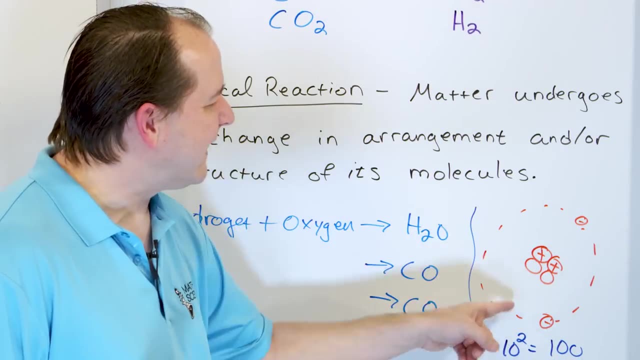 And then, as you understand more and more, I can tell you more truths so that you can make your own. you know, jump and make your own discoveries. So at first we tell you that atoms look like this: positive, negative electrons, they. 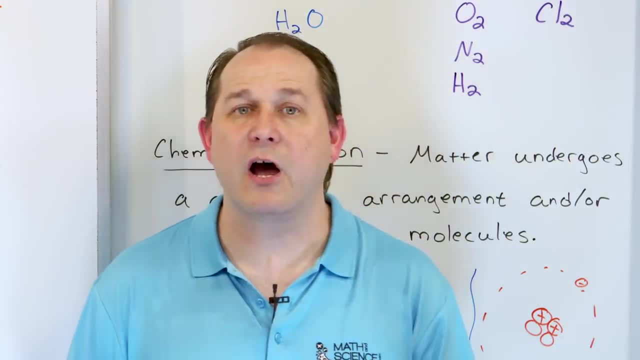 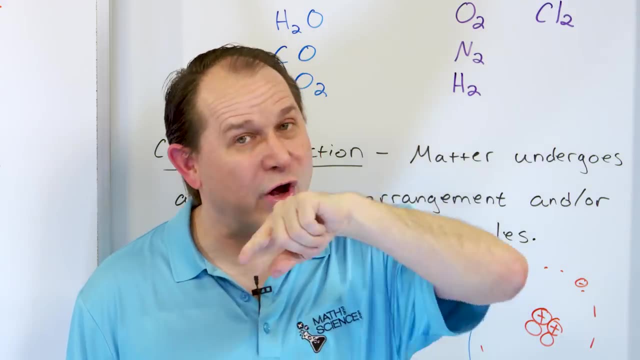 go round and round, but actually this picture is not right. So we have to talk about. what do we really know about electrons? And I'll give you a hint: Electrons are little bitty waves, Protons are also little bitty waves, And even the light that you see are little bitty waves. So it turns out. 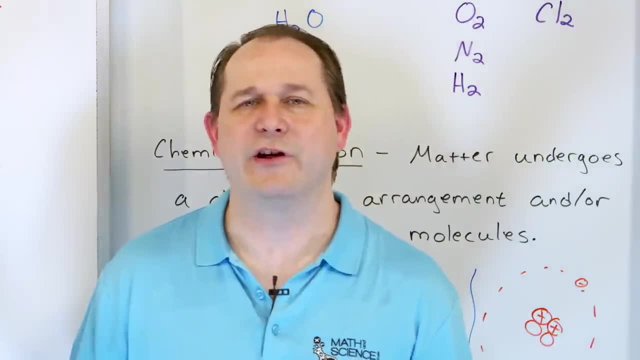 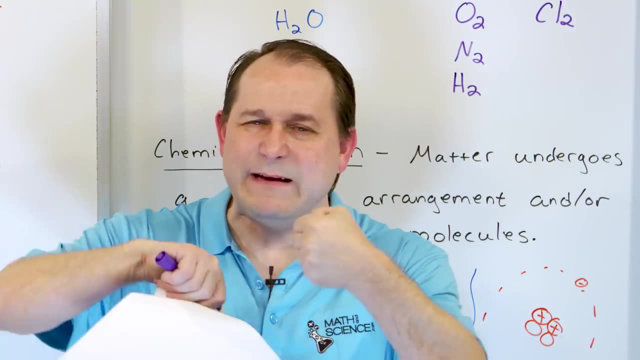 that I can summarize about 50 years of quantum research in the early 20th century by telling you that we pretty much figured, figured out that everything is made of waves, Even the things that seem hard. they're really made of microscopic little waves. But we have to to. 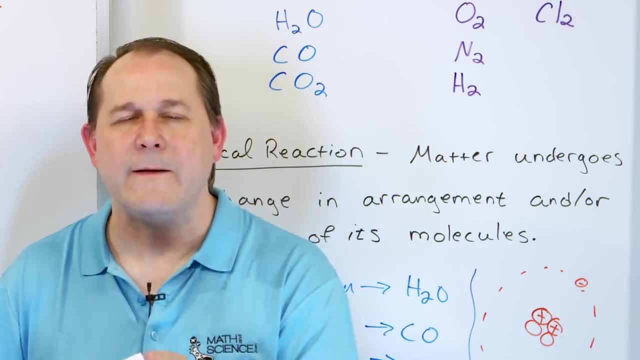 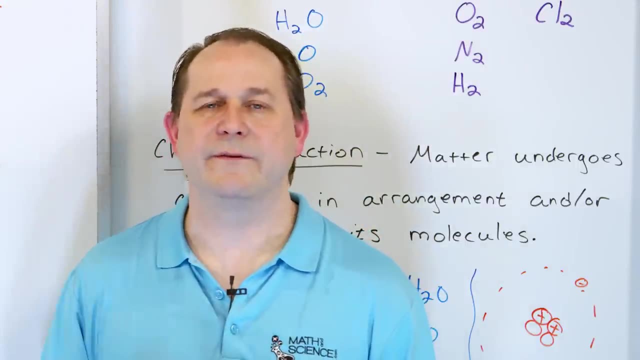 treat this education as a series of lies. we have to start somewhere, And then we have to build step, by step by step, so that you gain confidence as you go, And then we can get to the stuff down the line, in which case we run out of road, we have no more road, and you then have the tools to continue.